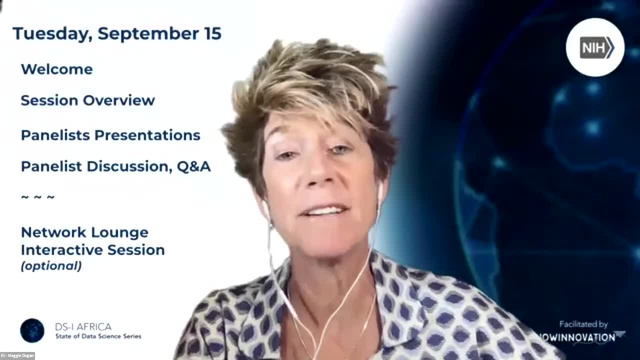 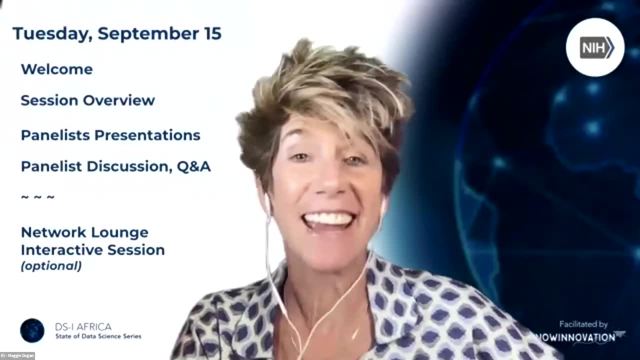 This is hosted by the National Institutes of Health Common Fund. My name is Maggie Dugan and I'm here with my colleagues from KnowInnovation. We're also known as KI. that's the KI in Kai Storm we used to get here. 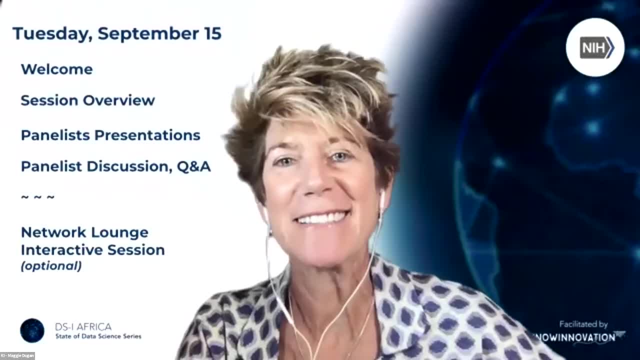 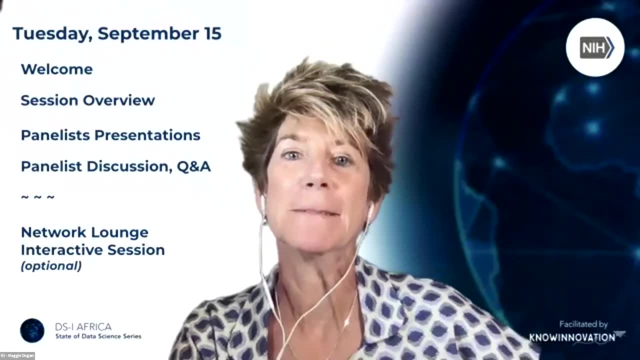 We're a facilitation team that specializes in accelerating scientific innovation and we are very pleased to be here. We've been asked to help support this virtual event for the NIH Common Fund. Briefly, our agenda today: Some welcoming remarks and tips for engaging successfully in the webinar. 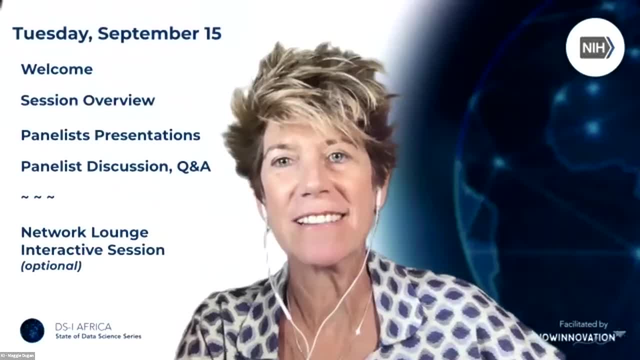 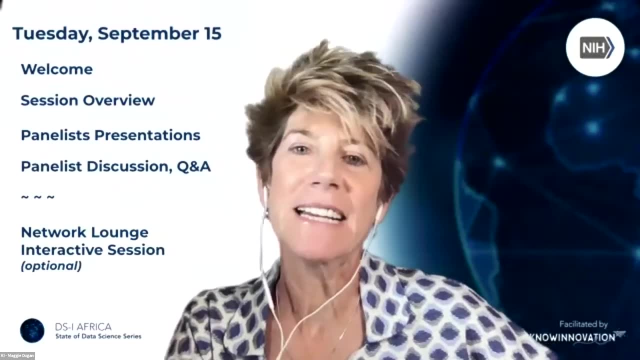 We'll have an overview of today's session on biomedical imaging acquisition and analysis from our moderator, Paul Perlman. This will be followed by 10 to 12 minute presentations from each one of our panelists. I'll let Dr Perlman introduce them. 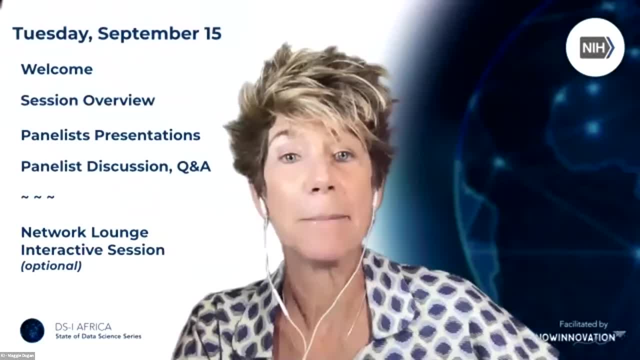 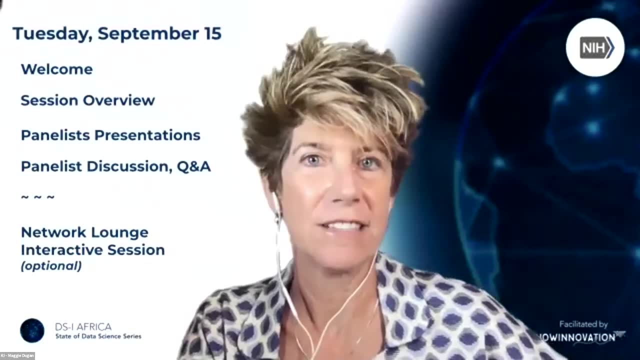 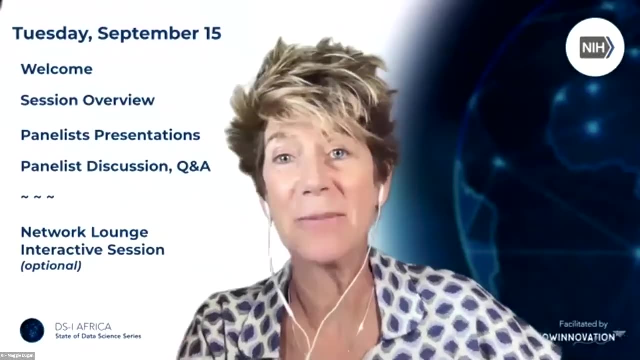 And followed by questions that will be answered, And then we'll have a plenary conclusion. This is all followed by an interactive networking session. This is an opt-in, So we hope you will choose to join. It will be an opportunity to engage further with the panelists and with each other. 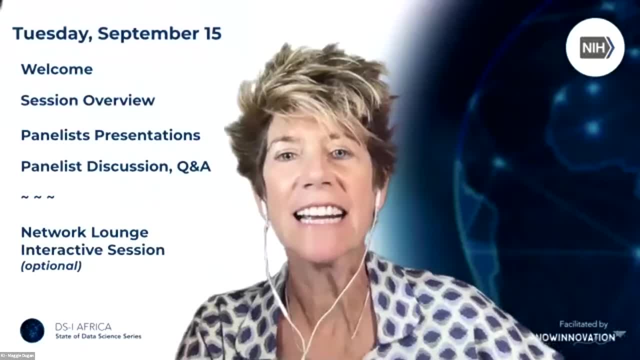 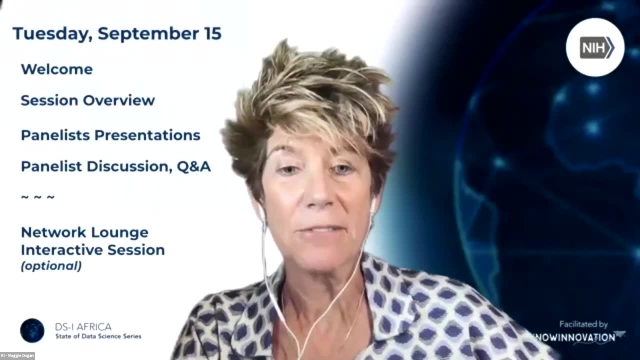 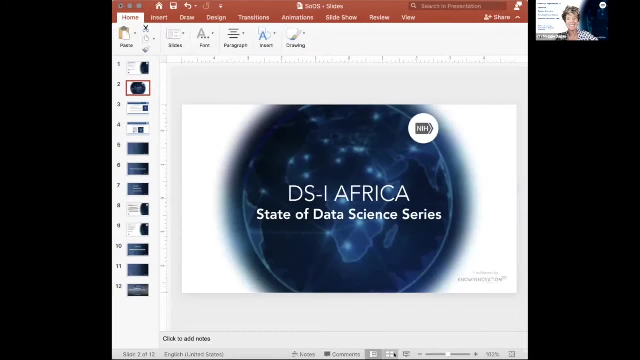 And continue to interact with everybody and dig deeper on the topic of biomedical imaging and data science in Africa. So, incidentally, I want to show you just a few slides to let you know that today's event- she opens a slide presentation associated with the funding opportunity. 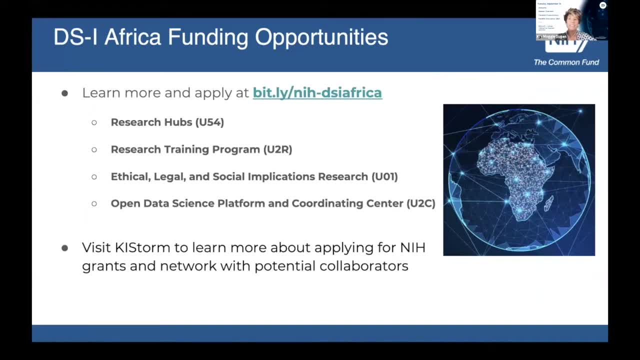 This is the NIH program on harnessing data science for health and discovery and innovation in Africa. So there are four different opportunities that are currently open: Research hubs, research training, ethical, legal and social implications, open data science platform and coordinating session. 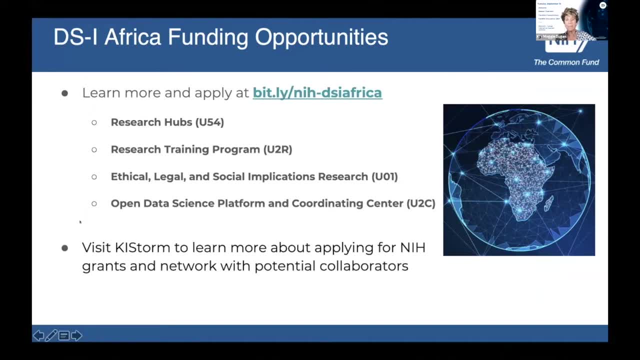 And then we have a webinar. This is an interactive session. If you want to learn anything more about any of these funding opportunities, we invite you to visit ChiStorm to learn more about how to apply, or also to go to the NIH site. bitly slash NIH dash, DSI Africa. 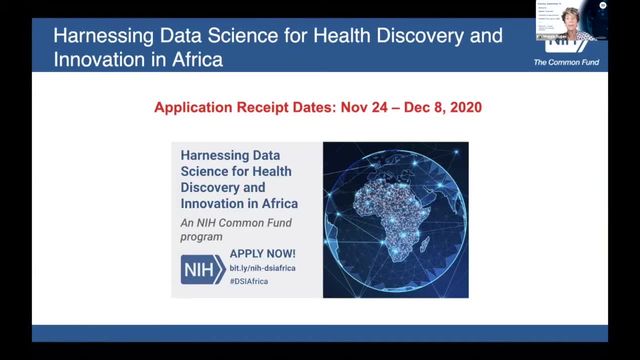 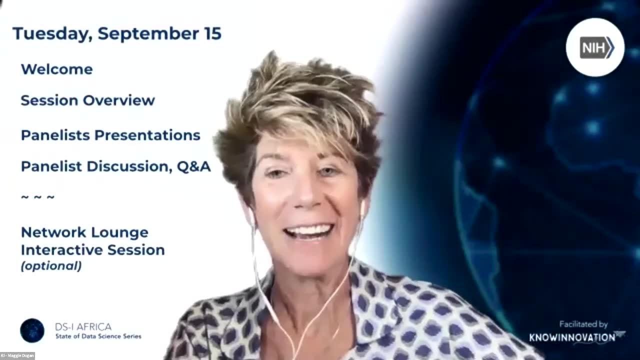 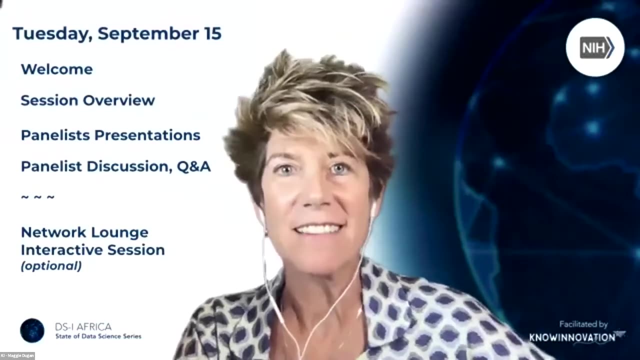 The application receipt dates are between the end of November and early December, So we encourage you to explore this further and find out more about how you can be part of this program. So before we start, just a few tips. We are recording this program. 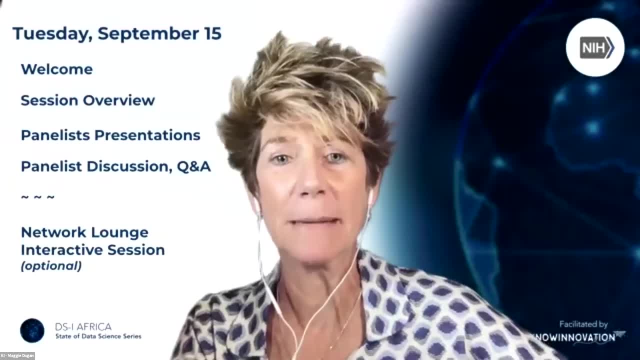 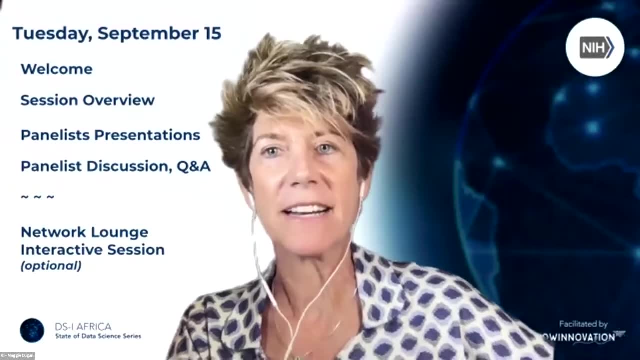 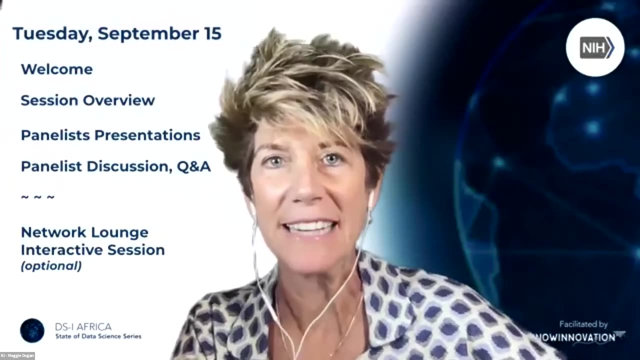 So if you want to see anything again, you'll be able to find it here on ChiStorm or on the NIH site. If at any point during today's session you get bumped out, you get kicked out, you have problems with Zoom, you can't find where you're supposed to go, you can always go onto the ChiStorm need help page. 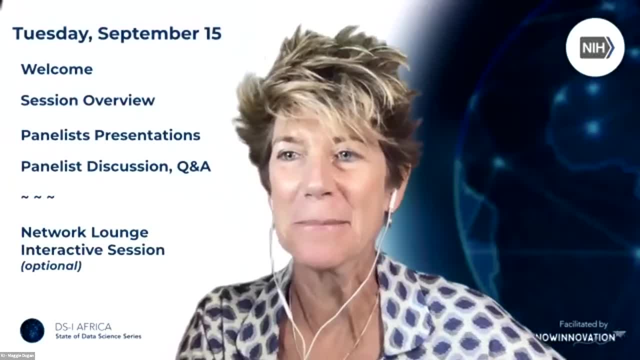 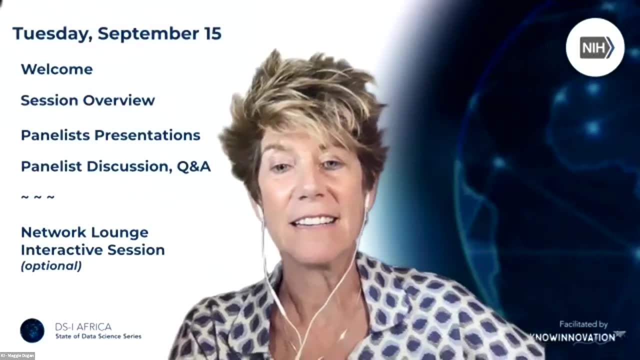 Someone will be monitoring and we can help you find your way back to where you need to be. In this webinar we have the opportunity to ask questions, So you'll notice at the bottom of your screen there is a little Q&A button with some thought clouds, some speech clouds. 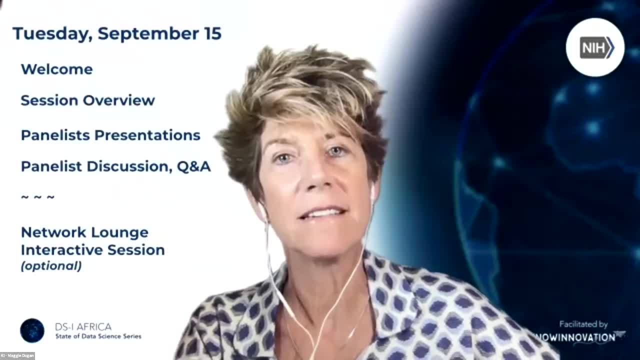 You can click on that and add a question And as well, you can see what other people are asking, And if there's a question that resonates with you particularly, you can say: yeah, I like that question too, by uploading that. 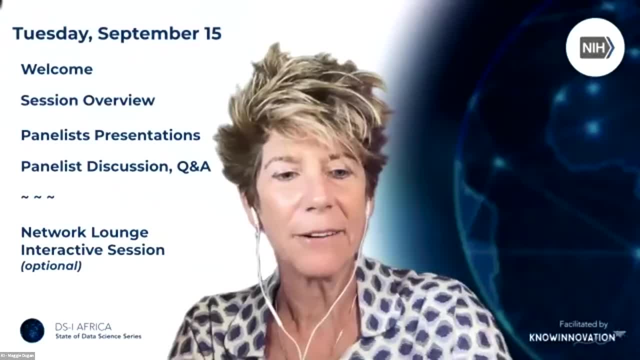 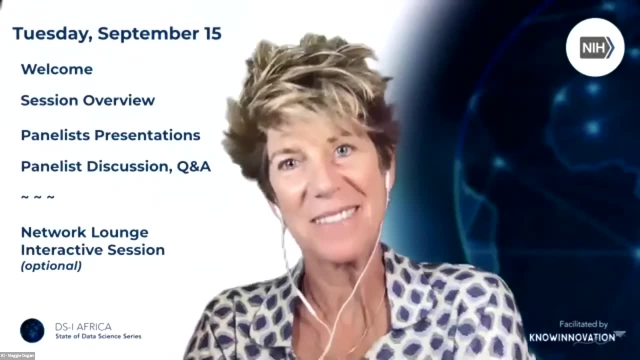 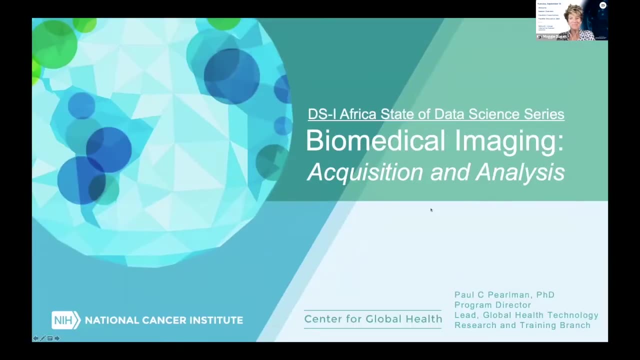 And I would just like to introduce to you our moderator, who is Dr Paul Perman, from the Cancer Institute. Dr Perman's backdrop is a photo of the Institute. He opens a slide presentation. Thank you, Maggie. I'm going to keep this brief so we can get directly into our talks. 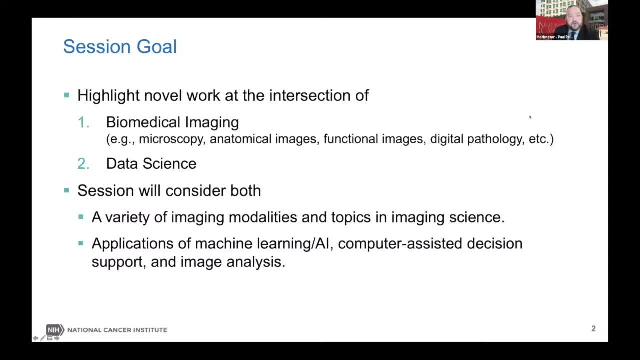 So our session goal today is to highlight novel work at the intersection of biomedical imaging and data science. The session will consider both a variety of imaging modalities and topics in imaging science, as well as the applications of machine learning, artificial intelligence and computer-assisted decision support and image analysis. 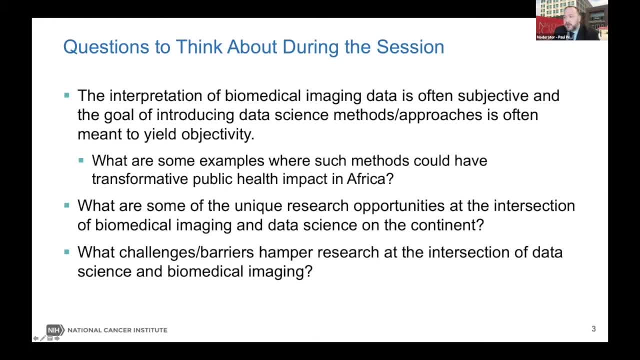 As we're starting to think during the session about the broader DSI program and maybe potential applications to that program, I want you to think about the interpretation of biomedical imaging data often being subjective and that the goal of introducing data science methods and approaches is often meant to yield objectivity. 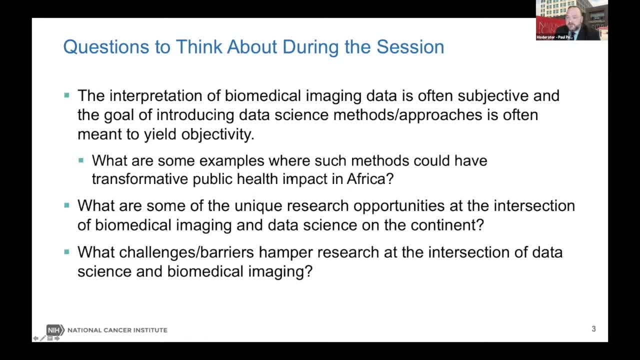 So, with that in mind, what are some of the examples And what are some of the examples of research opportunities that you see in the field where such methods could have a transformative public health impact in Africa? Furthermore, what are some of the unique research opportunities at the intersection of biomedical imaging and data science on the continent? 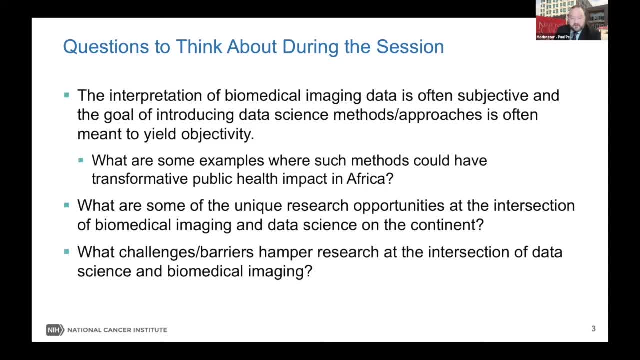 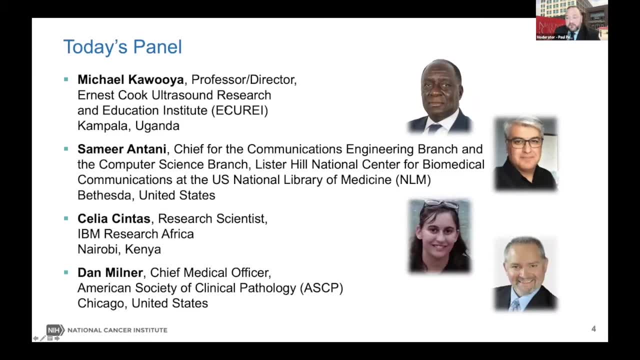 Finally, what are the challenges and barriers that hamper research at the intersection of data science and biomedical imaging? So today's panel consists of these four speakers: Dr Michael Kaluuya, Dr Samir Antani, Dr Celia Sintos and Dr Dan Milner. 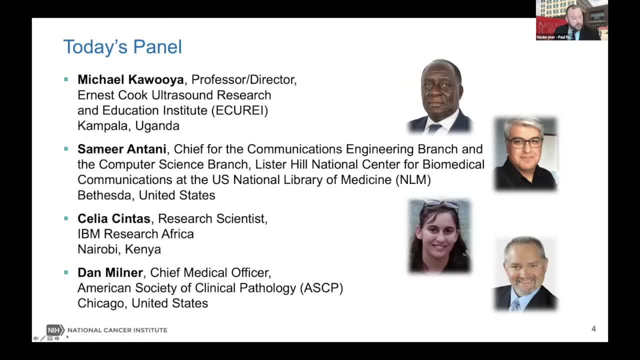 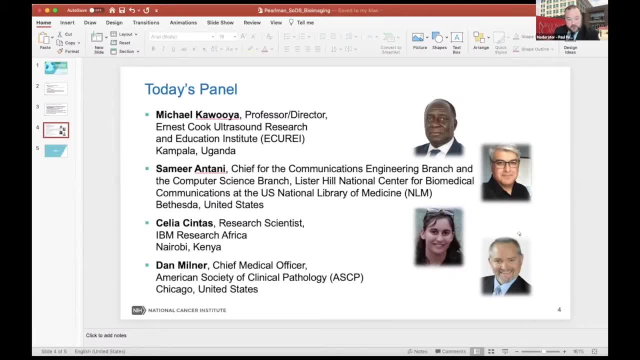 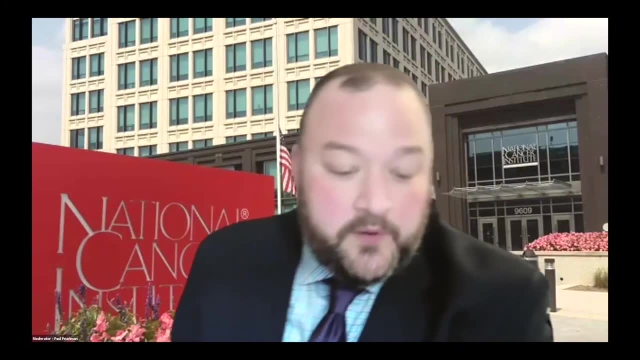 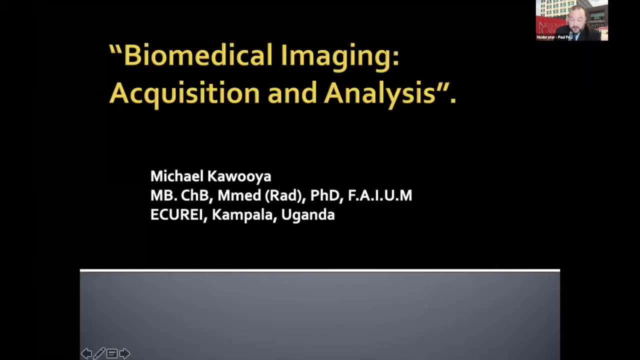 who I'll introduce prior to each talk. talk. So as Dr Kulia is getting his slides up, I will go ahead and stop sharing and introduce him. So Professor Michael Kulia is a general radiologist with a special interest in diagnostic and interventional ultrasound. He's engaged in clinical work, research and teaching at 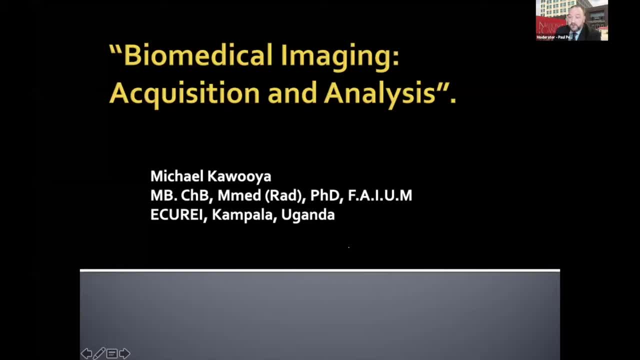 the Ernst Koch Ultrasound Research and Education Institute in Kampala. With that, I'll turn it over to you, Professor Kulia. Professor Kulia sits in front of a blue wall with a photo of an MRI machine. Good afternoon to you from Uganda. He opens his presentation, The talk I'm going to. 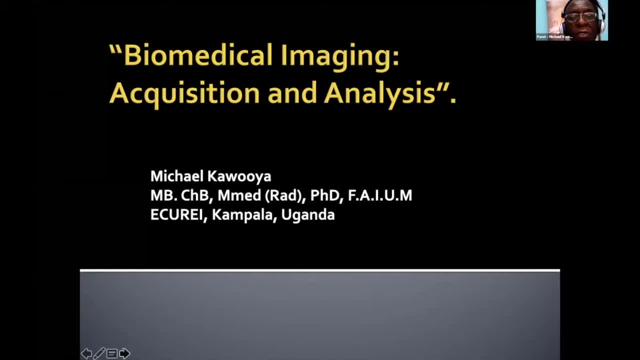 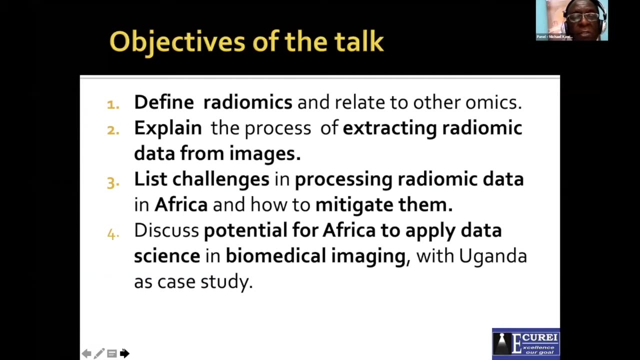 handle is going to be basically on imaging And we are going to look at the ultrasound. The objectives to define radiomics and relate to other omics. Explain the process of extracting radiomic data from images. List challenges in processing radiomic data in Africa and. 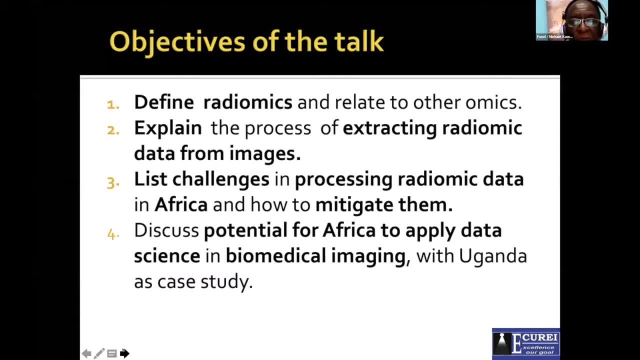 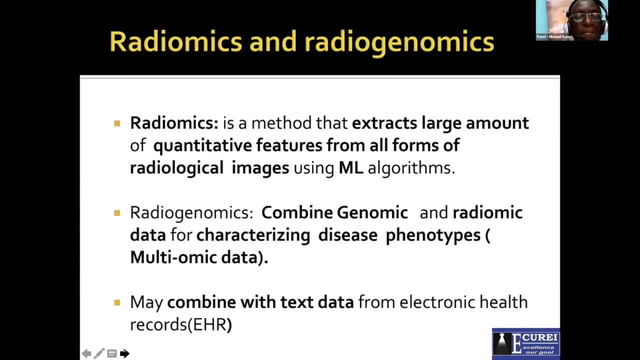 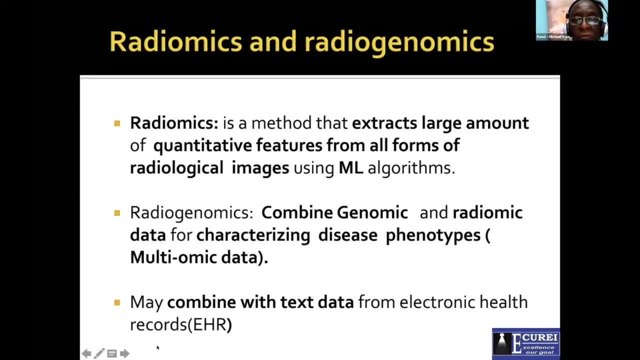 radiological imaging using machine learning algorithms, And there's also what we call radiogenomics, which combines genomic and radiomic data to characterize disease phenotypes, and we call this multi-omic data. You may also combine this with text data from electronic health records, if that is necessary. 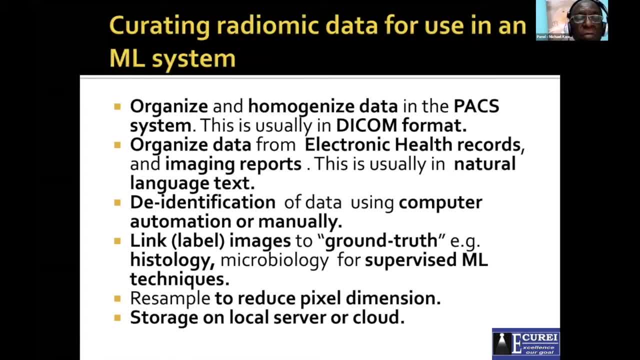 Curating radiomic data for use in an ML system. Data from imaging studies has to be organized and homogenized in the PACS system, and this is usually in a DICOM format. We organize the data from electronic health records and imaging reports, and this is usually in natural language text. 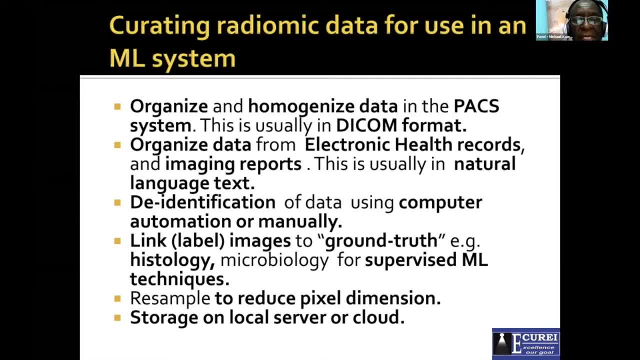 The data has to be de-identified and then also has to be linked to the ground truth, which may be histology or microbiology, because it is data which is very highly had to reduce the pixel dimensions so that then we can be able to process it with a computer we have. Others requires a very high speed computer And then that data 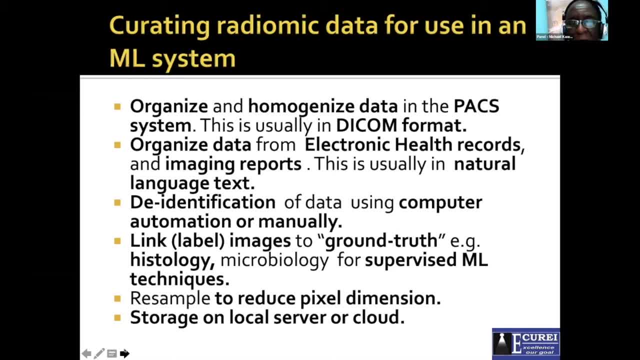 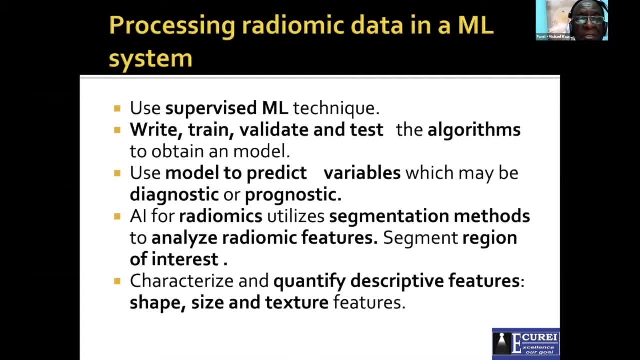 can be stored in the source, you the source stored on a local server or on a cloud. Now how do we process radiomic data in a machine learning system? We usually use supervised machine learning technique. We write, train, validate and test the algorithms to obtain a model. Then we use that model to predict variables which 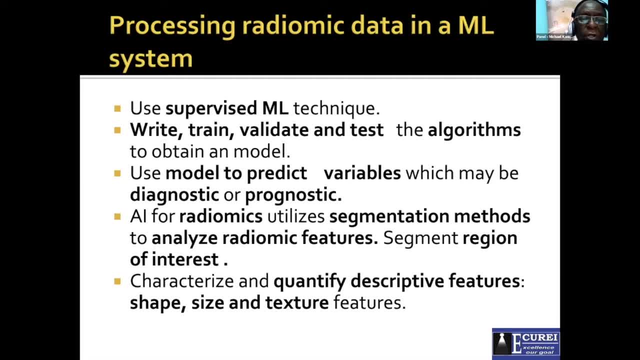 may be diagnostic or prognostic. Artificial intelligence for radiomic data utilizes segmentation methods to analyze the radiomic features and we segment the region of interest And then after that, we characterize and quantify descriptive features, which are like shape, size and texture features. Now there. 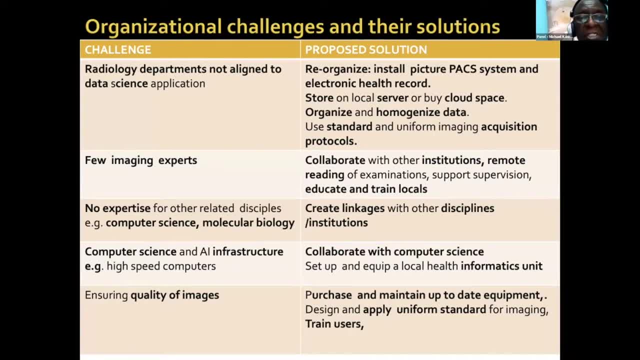 are challenges with radiomic data. We are dealing with radiomic data data from radiology in Africa. The slide displays a table of challenges and proposed solutions- Organizational challenges. on this table we see radiology departments are not aligned to data science application because this is new in Africa, So data has to be reorganized. 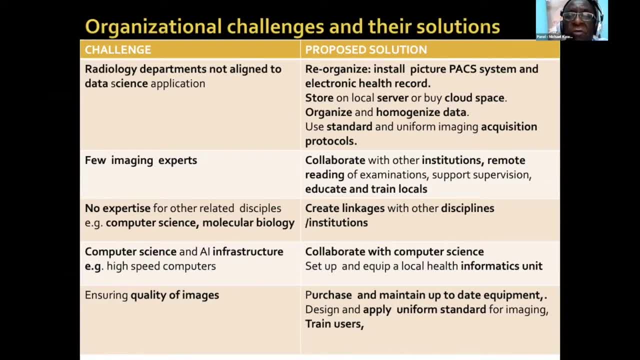 We have to install a PACS system and also electronic health records, And these are not all over the country, all over the continent. Many departments don't have PACS systems. The data has to be stored on a local server or in a cloud space, organized and homogenized. And then it's important that the imaging 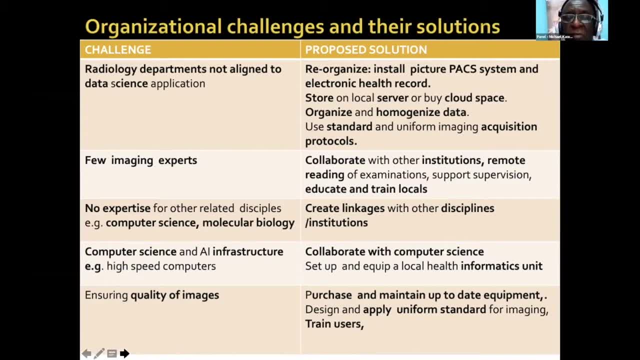 protocols we use to be standardized and uniform so that data from different centers and from different machines can all be processed together. We also have a few imaging systems. We have imaging experts, and this one you can overcome through collaborations or you can use remote reading of images. And also it's important that you train locals to do the work and not 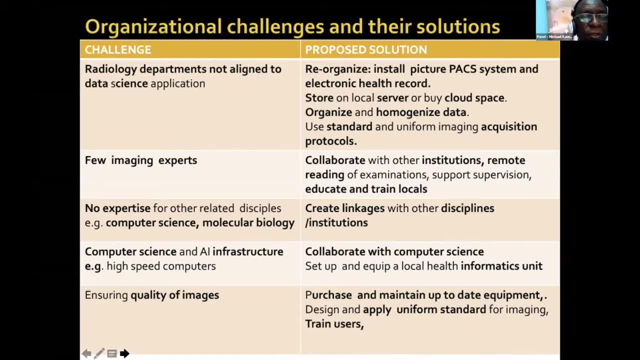 only to rely on remote reading. In many departments there's no expertise in computer science, And so there is need for the department to form linkages and collaborations with computer science departments or institutions where there is a need for that. Thank you. 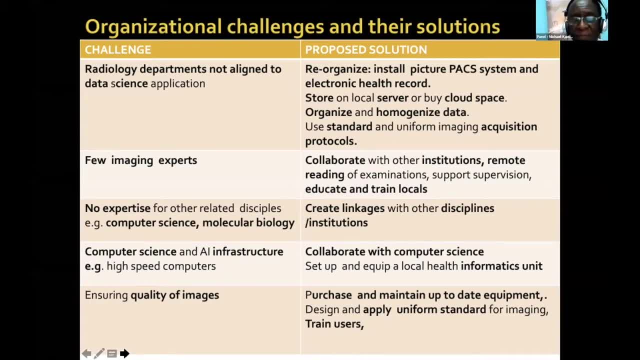 Thank you, Dr Mo. Thank you very much, Dr Tegel. Thank you, Dr Mo. Thank you, Dr Tegel, And now I'd like to look at some of the other questions that have come in. 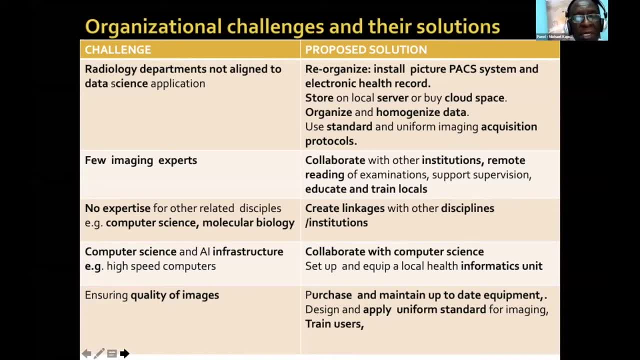 So one of the questions is: what is the role of digital media in the application of computer science? So what is the role of digital media in the application of computer science so that they can access machine learning and artificial intelligence facilities? Now, the computer science and artificial learning infrastructure requires very high speed computers. 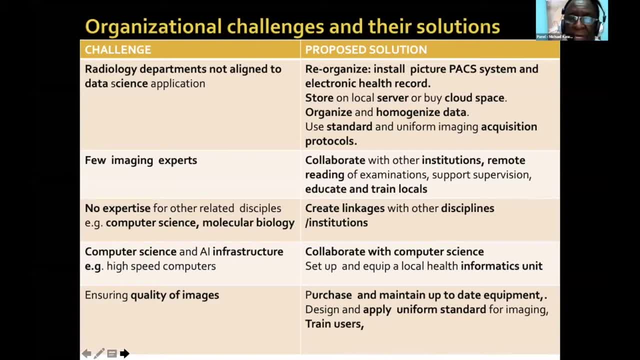 These are not usually found in radiology departments, but you can collaborate with the computer science department, and here one is usually likely to find high speed computers which can process data for machine learning and for artificial intelligence. and the quality of the images in many parts of Africa still needs to be improved, and so there 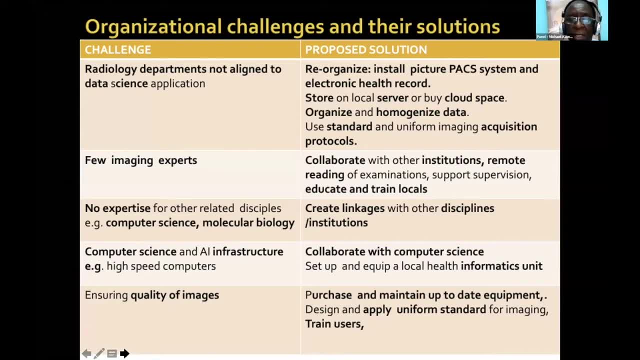 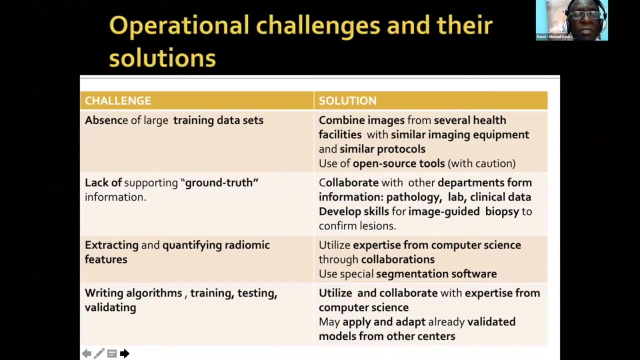 is need to purchase and maintain accurate equipment, and also design and apply uniform standards for imaging and train the users, and this way you can ensure good quality images which you can use in your artificial intelligence systems. there are operational challenges in this area: absence of large training, data sets, and so this. 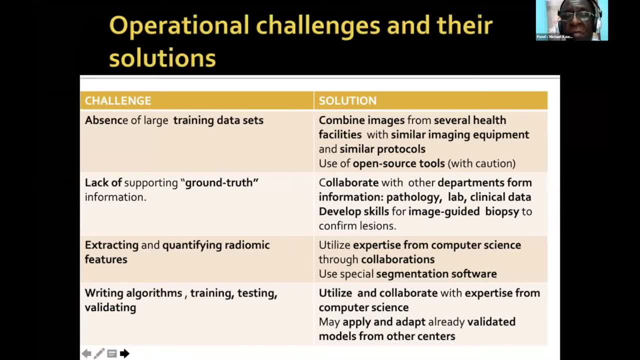 one. you can overcome by combining data or images from different imaging facilities but ensure that they're using similar imaging equipment and also similar protocols. and one can also access open source tools, but these are usually heterogeneous and have several other complications with them. now there is need to leave that data, that images, to the ground truth. 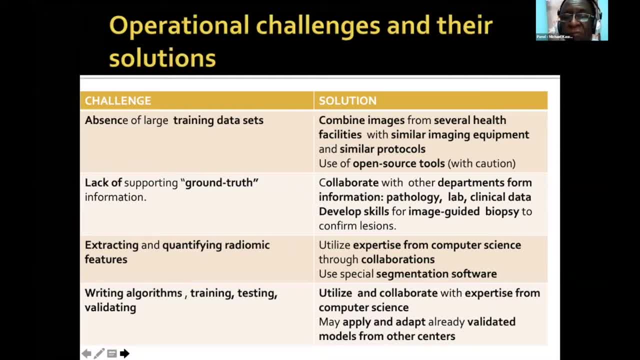 and so here we collaborate with our colleagues from pathology, from microbiology, so that we can, when we see an image, then we can be sure that either this is tuberculosis or this is cancer, through use of either pathology or microbiology. that is the ground truth to our imaging data. 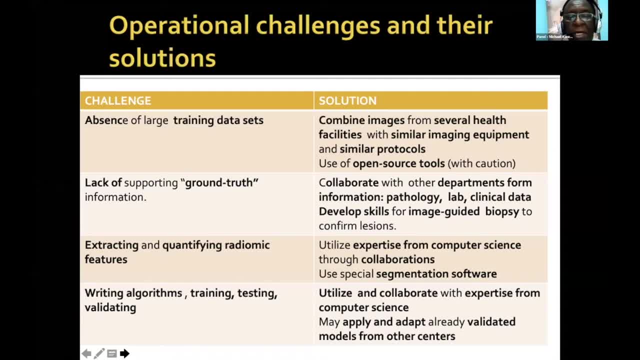 the data has to be extracted and quantified, and here we use experts from computer science who can help us to extract data from these images, and also they can have computers with segmentation software to segment the images and then you can be able to to have this data processing, the machine learning artificial. 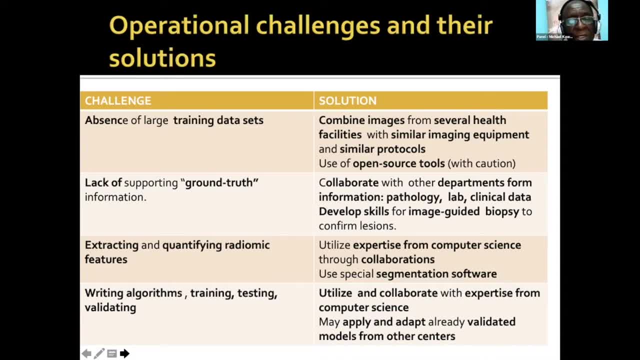 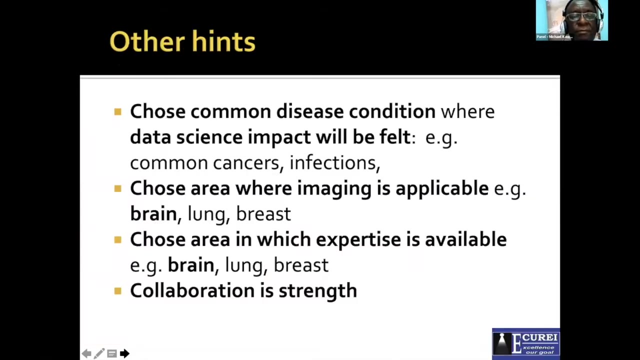 intelligence system. the writing of algorithms, training and testing and validating data is not a skill which radiologists have or people in radiology, but then we utilize our colleagues from computer science who have the expertise to help us to write these algorithms, to train and to test and to validate that data. now some hints. if you want to undertake a project in 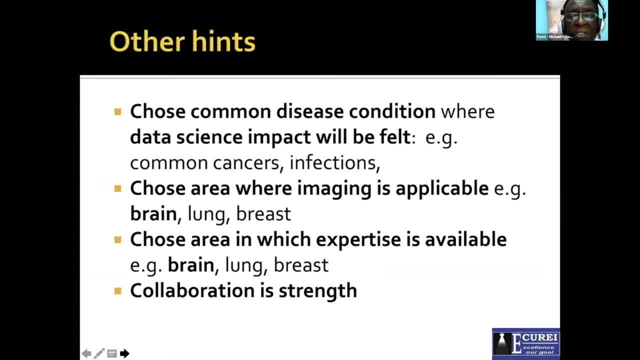 data science. in africa you choose common diseases where the data science will have an impact, for instance, many cancers like cancer, prostate cancer, breast infections like tuberculosis. these are areas where data science may have an impact. we choose area where imaging is applicable, for instance brain, lung, breast. here we can apply imaging for the brain like mri and ct scan. 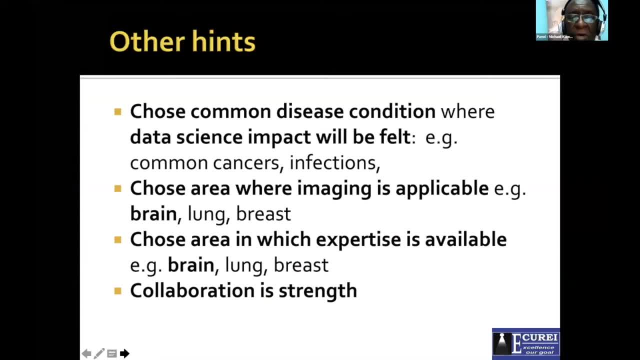 chest x-rays and ct scan for the lung and mammography and ultrasound for the breast. so that okay. so as part of our training then we'll be using the ground data on machine learning for using indigenous statistics for implementing certain estimates in給 cyber intelligence or marketing. that's an area where you are likely to pick a topic to do your research in artificial intelligence or to apply artificial intelligence and machine learning and you choose an area where you have expertize which is available, for example, if you are experts for interpreting brain mri or brain city, or experts for 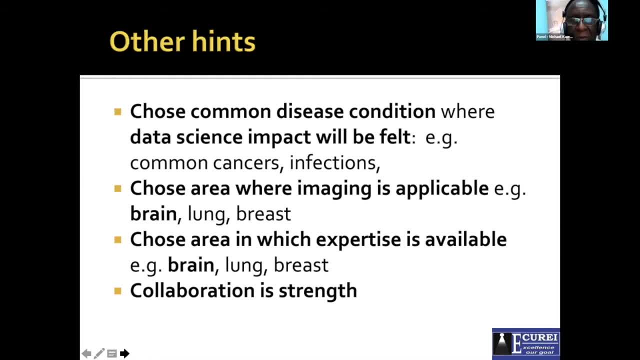 interpreting lung CT or breast mammography and ultrasound. and at times you may also need to link with colleagues from molecular biology for the molecular biology aspect of that of the tumor, also with colleagues from oncology and also with colleagues, of course, from computer science. so choose an area where you have expertise and you can undertake this project when you are have all. 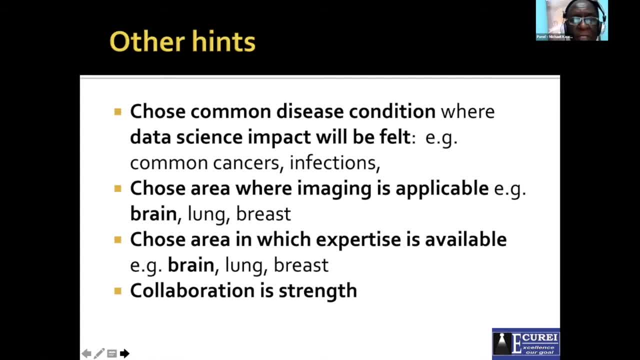 the all, the capacity to do it, and then it's important to collaborate, collaborate, collaborate is strength, collaboration is strength. you collaborate within the facility, you collaborate with other disciplines, you collaborate with other universities, with other centers and also other continents, and then through this you can have all the skill, the right skill mix. 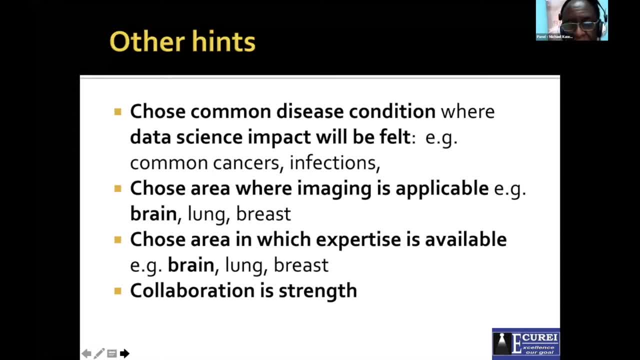 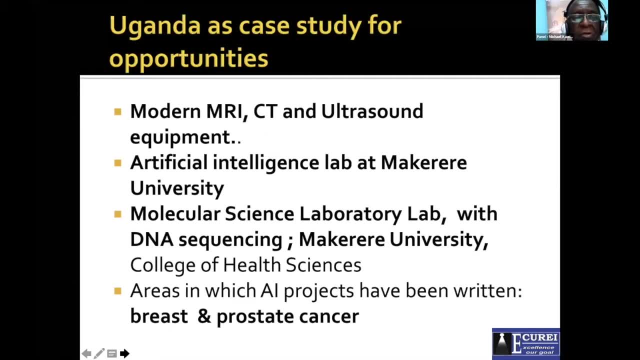 which you need to undertake a data science project. there are opportunities for many countries like Uganda. here we have a modern MRI machine, CT and ultrasound equipment, so this can give you the set of images for you to use in your machine learning or artificial intelligence model. and also in Uganda, we are fortunate- there is artificial 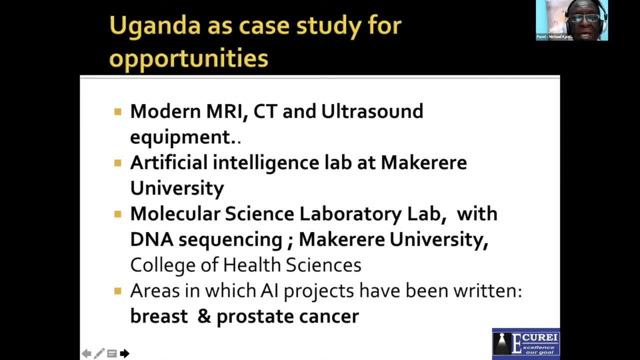 intelligence laboratory at Macquarie University and these are very friendly and they're welcoming and you can have collaborations and do projects with them. and we also have a molecular science laboratory at Macquarie University College of Health Sciences and with very good, modern equipment like DNA sequencing, that can be done and so these are. 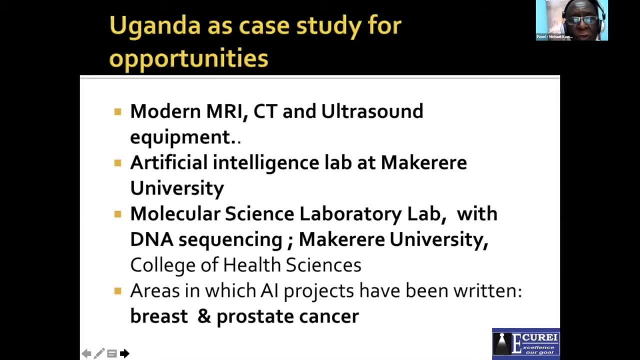 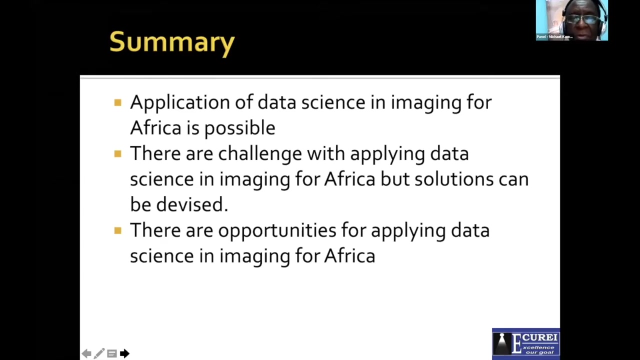 all opportunities and there are areas, a lot of disease conditions in Uganda, common cancers like prostate cancer, like breast cancer, where you can undertake a project in data science application for innovation and and for research and also for clinical applications. so, in summary, application of data science in imaging for Africa is possible. there are 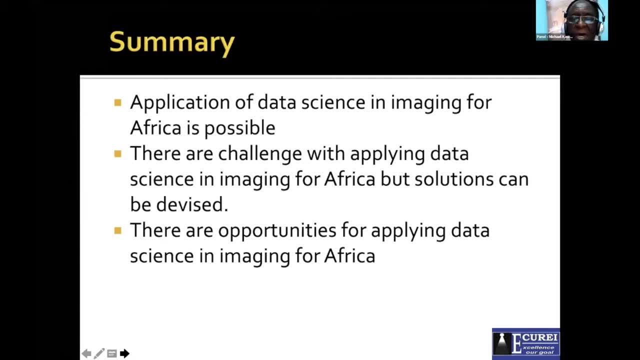 challenges with the applying data science in imaging for Africa, but there are also solutions which can be devised, especially through collaborations. there are opportunities for applying data science in imaging for Africa and this should be taken advantages of, and the ECE INH grant is a great opportunity. so I encourage you, I invite you, to come and join in and see. 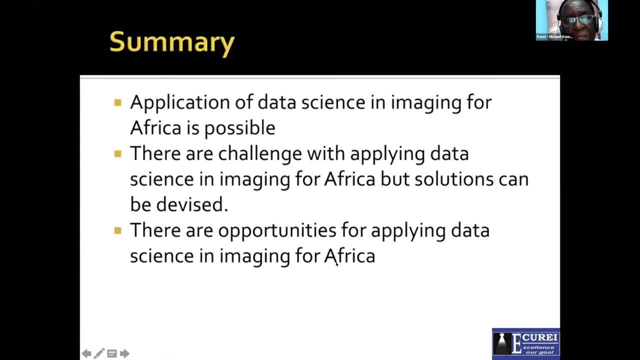 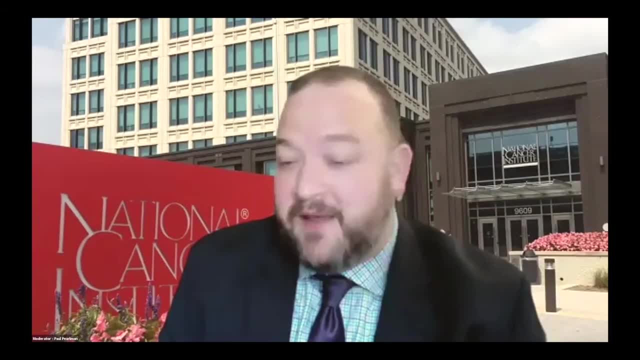 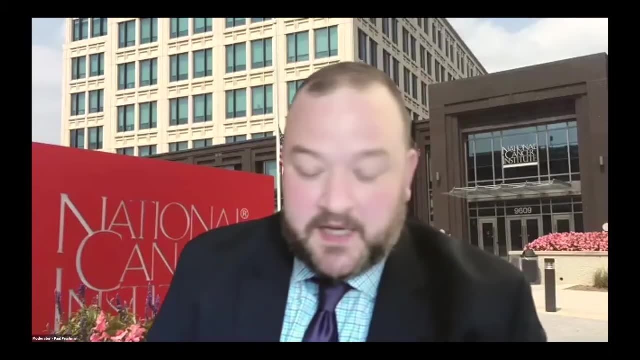 how you can make use of this opportunity. thank you so much. thank you, Professor Kwuya. I want to remind everyone that the Q&A box is live and you can go ahead and start putting in questions as you think of them. so, while Dr Antani is getting his slides up, I want to introduce our next speaker. 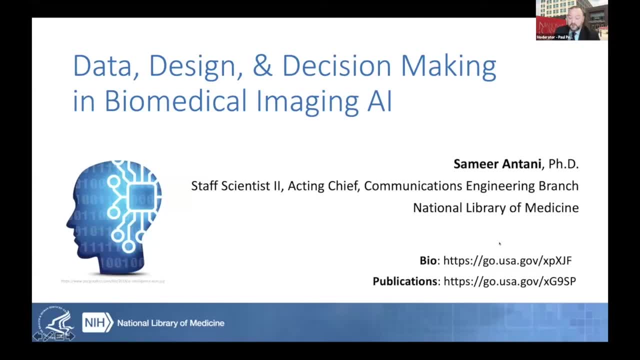 Dr Samir Antani is an intramural scientist at the US National Library of Medicine with research interests in medical and medicine and machine learning for a variety of clinical problems such as cervical cancer, HIV and TB, sickle cell, cardiac myopathy and others. Samir 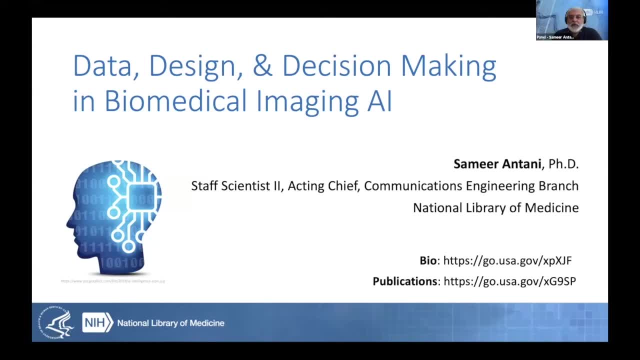 Antani's backdrop as a poster for NIH, he opens his slides. thank you very much for the introduction, Paul uh, and welcome everybody. good afternoon to everybody in Africa and good morning to people in US and other parts of the world, as per your time zones. I'm going to talk about several aspects. 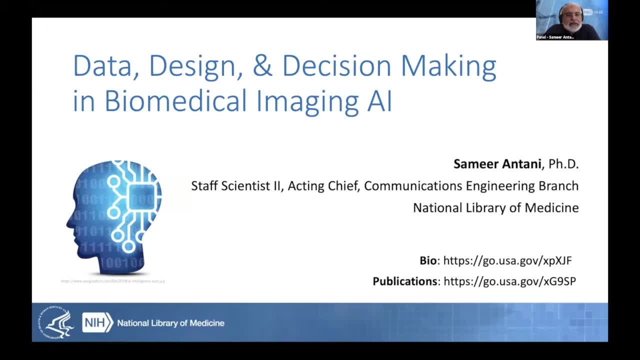 in biomedical imaging AI that relate to data science, to do with data design and decision making and the interactions between them, and I'll draw on some of my experience as an intramural scientist at the NIH working on some of these biomedical imaging AI problems and to help you think about. 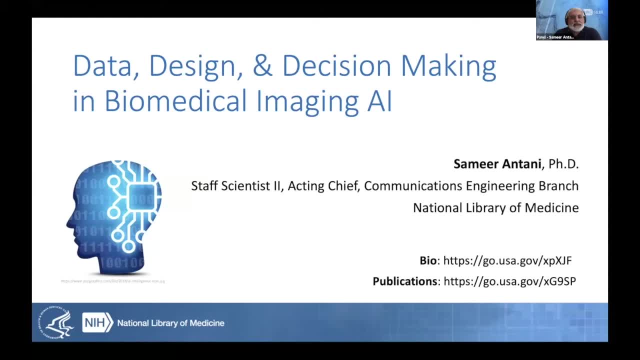 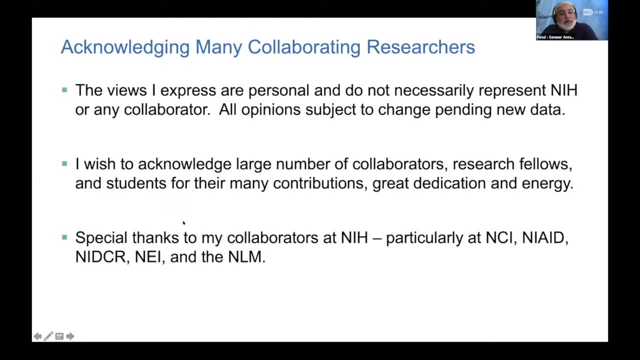 your problems or your challenges as you embark on this journey. So, before I go too far into my talk, I would like to acknowledge that what I'm drawing on are my experiences, that I have derived from many, many collaborations over the past over 20 years, and my views are personal and they do not necessarily represent the NIH. 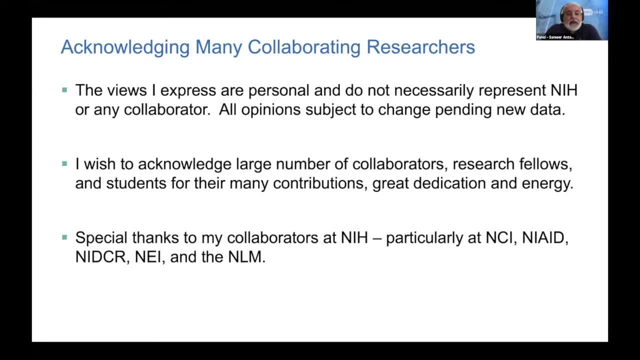 or any collaborator in particular, And as this is a rapidly evolving field, my opinions are subject to change as I learn more and we all learn more in this area, And the collaborators are many and they are varying from students who come from different parts of. 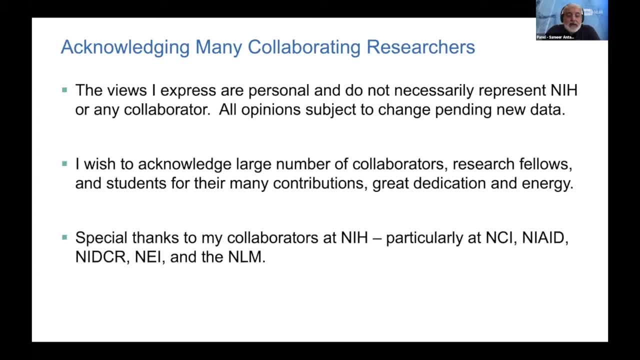 the world, to research fellows and other organizations, And within the NIH, I must acknowledge my collaborators at the National Cancer Institute, the National Institute of Allergic Infectious Diseases, Dental Craniofacial Research, the Eye Institute and the National Library of Medicine. of course, Dr Antani turns to a slide with images of x-rays, MRI scans and ultrasounds. 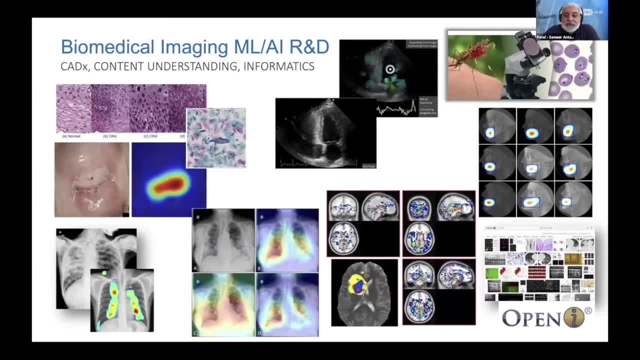 So this is a rather busy slide in images, but I'd like you to think about various imaging modalities that you see here and how one would process these images. On the left you can see, top left, a histopathology image of the. that's a from a. 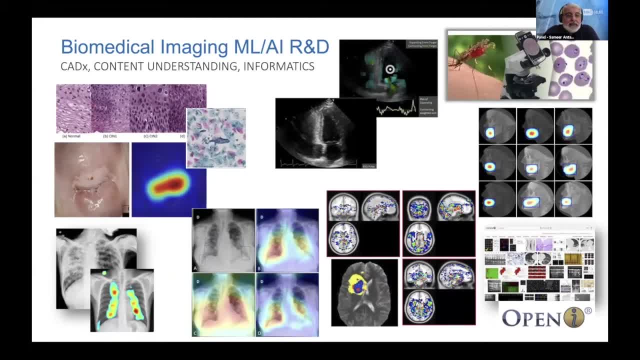 biopsy of the uterine cervix to do with cervical cancer, and I'll touch upon that a little bit. You also see a small swatch of a microscopy image of a from a cytology from a typical cancer, And on the right you can see an image of a pap smear, a liquid pap smear perhaps. 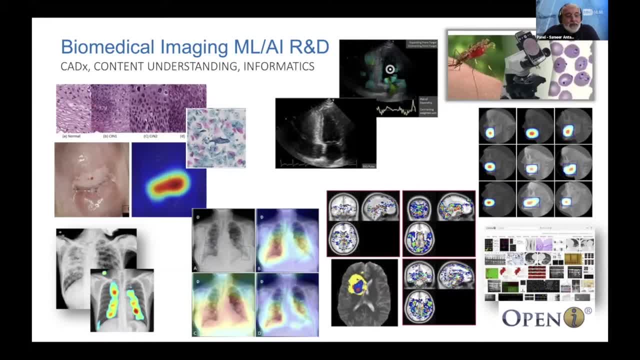 or a traditional photograph of the tissue. You go into just x-rays looking for disease patterns and onto 3D volume images from the brain, The uterine diseases that are exhibiting some kind of change in the substantive matter or in terms of functional responses. 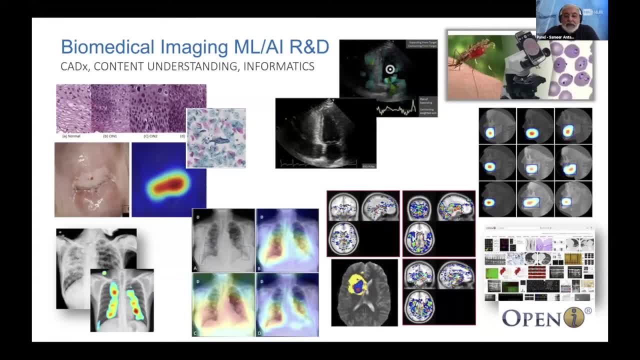 are the brain's process, visual and auditory and sensory data. On the top you can see both. you can see an ultrasound image of the heart where you see not only the ultrasound data, which is sometimes in terms of small snippets. 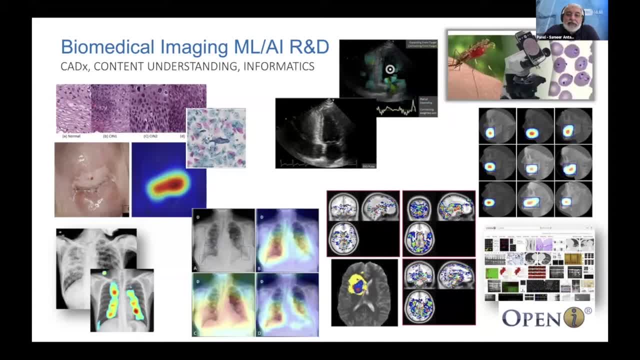 and as the video, but also an EKG that is embedded in there. That would be one-dimensional signal data that one might need to process. So you have a large collection of similar images and you can get a lot of Roux-voult data. 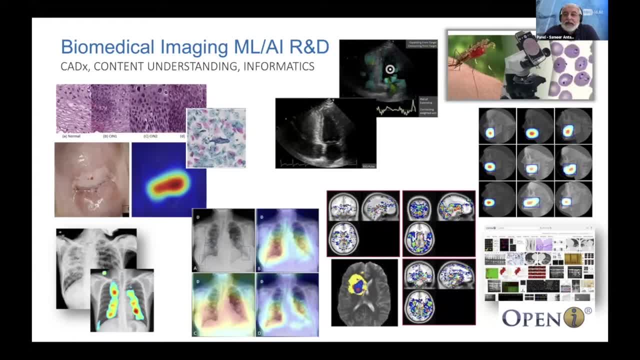 exactly from that, which is this partnership between the brain and the cell. And so, in terms of the tumor disease, as you see, you'll see that there are many small, large, small pieces of data that are spread out, And so I think the important thing to know about that is: does the patient understand the cancer and how they perform. So a lot of these images are the cases that star residents use. you are a patient and I have known these things for over a decade, So I'm going to stop there, I'm going to stop there, I'm going to stop there and I'm going to stop there. so if they understand it, then we're going to go on to the next area, which is ultrasound, which is the treatment case. 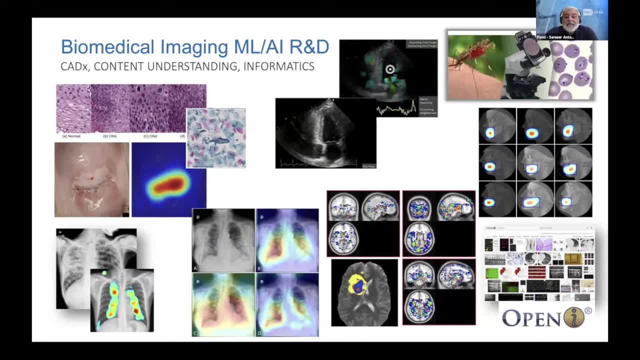 means if you have metadata tags, or you may have patient health records or you might want to recall them by their appearance, you it's very natural for us, as we look at pictures, to be able to recall what something looked like, and that is the field of image understanding or content-based. 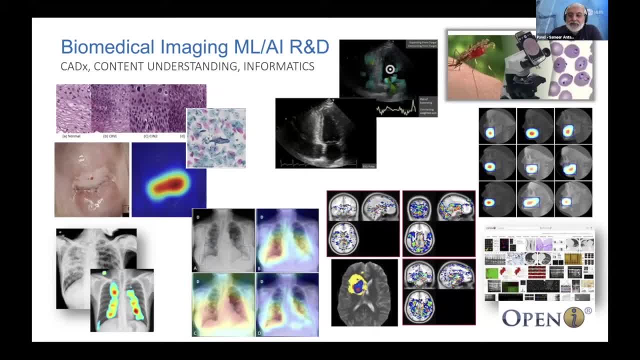 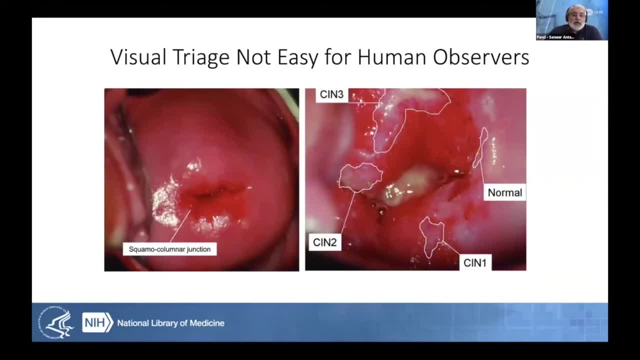 image retrieval, which is something that the open eye system tries to do in trying to connect words and pictures which are natural to us as humans. so, with that background, i'll take you into on a journey, uh, which is to do with detecting cervical cancer or, more importantly, pre-cancer, since that 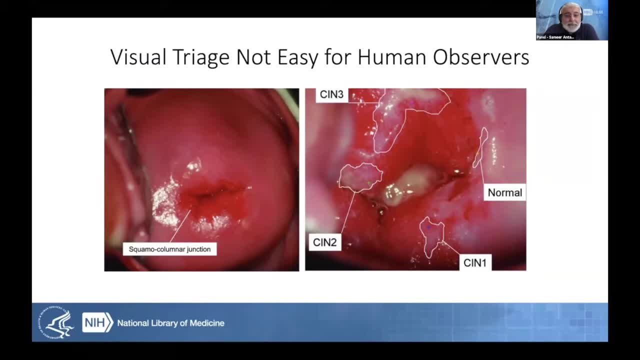 can be treated. the slide displays side by side images of a uterine cervix. now, what you're looking at in the left is the picture of the different cervix as seen by a gynecologist or gynecologist or oncologists, uh, during the routine exam. and uh, what you're seeing there is, uh, the, the dark. 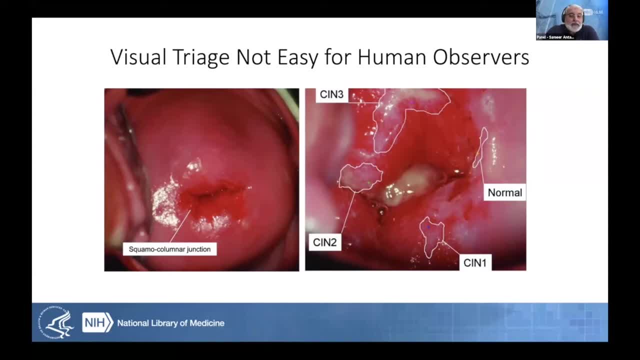 region in the middle is the os, which is the entrance to the uterus, and what you're looking for are uh changes in the epithelium of the squamous uh tissue there, and there are two tissue types: the columnar cells and the squamous cells, and it's at this junction that you, we, tend to see. 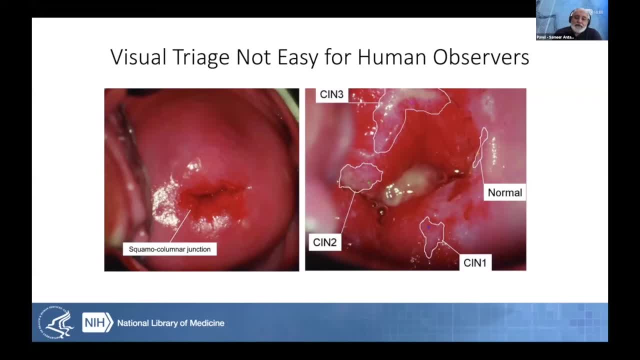 the invasive effects of human papillomavirus, certain types of them that are particularly oncogenic and can lead to cancer. and on the right there are some regions that have been marked by an oncologist for us grading them as stage one, stage two and stage three. it's after stage at stage two and 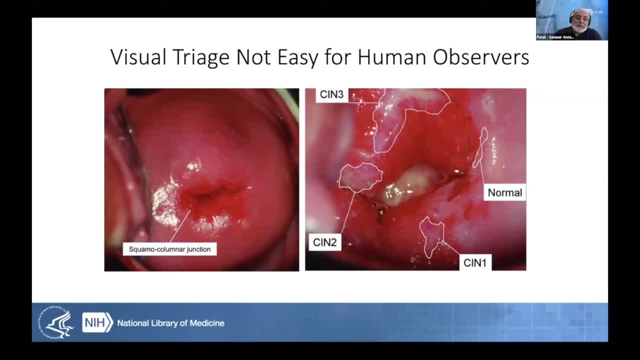 beyond is what we start labeling as pre-cancer, where uh one would want to treat and and uh using thermal ablation perhaps, or cryotherapy, so that uh any further damage is is eliminated and uh, the woman can resume her normal life. uh, but we, this is called visual. 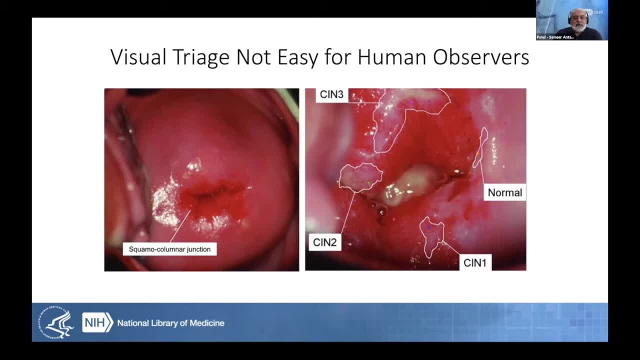 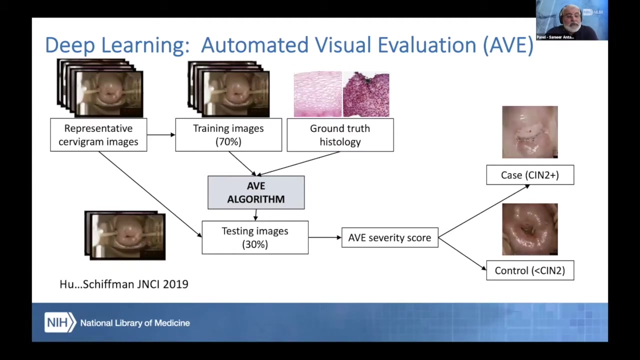 triage, but it's not so easy for human observers and there is great subjectivity. and of course, this presents a good opportunity for computers to intervene and perhaps highlight regions, those who not necessarily know what they know and can be subordinated to computerized smartphones. and these, these fandas have been released on patient and digital platforms. 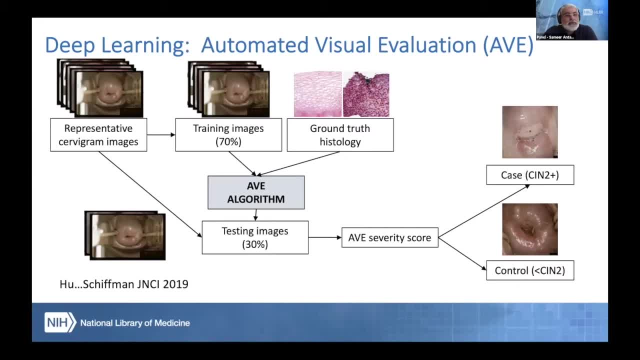 to be able to watch their own movements in the future, but the work that we're doing right now is that we're able to use these spaces on the screen to to provide some objectivity on on how to detect disease and and where they can be treated. 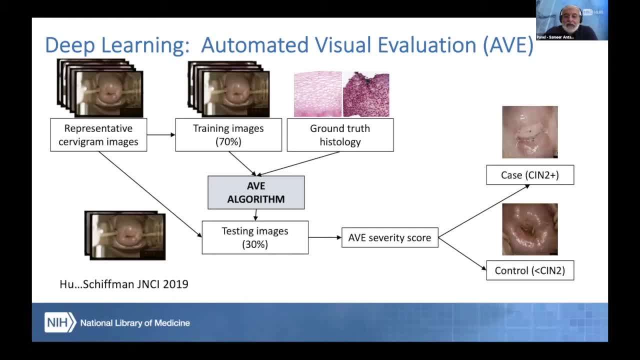 score that predicts that an image is either a control- that means normal- or is a case which is deserving of treatment. now to train this algorithm, of course, we had a large collection from a seven-year study conducted by the National Cancer Institute in CI, in the Guanacaste region of Costa Rica, and several thousand. 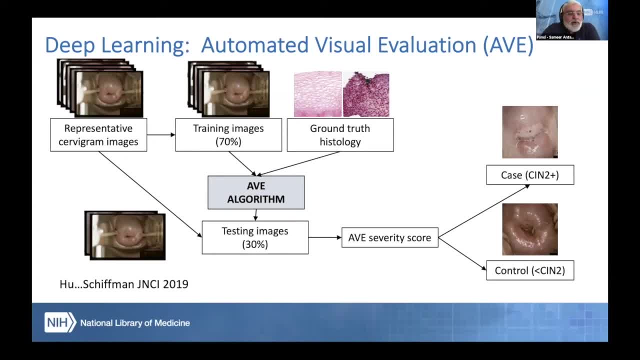 women- nearly 10,000 women were were were followed over seven years and the collection of images from every visit were then grouped into training images that were truth and or there were those that were indeed cases. there were biopsy truth that was applied to them, and those selections were used to train the. 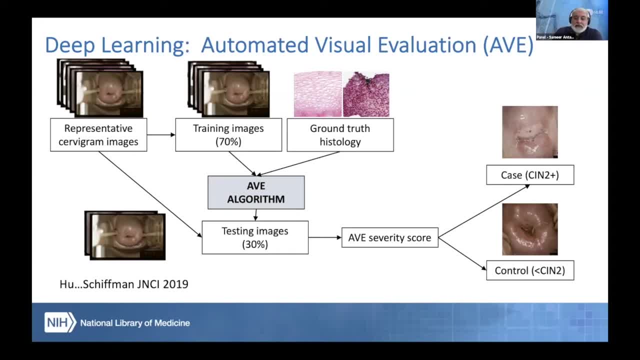 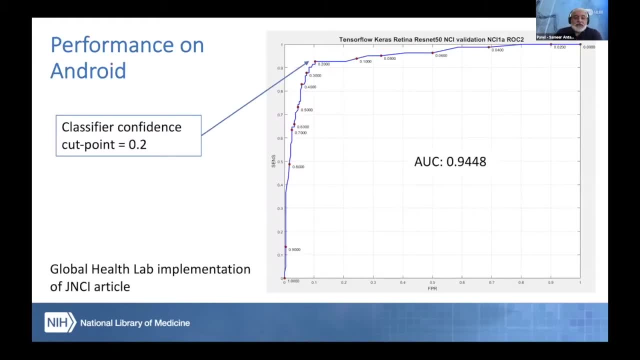 network and tested them so that it has very high performance, and the performance of the exposure to the selected images is very powerful. The performance of the selected images is very powerful. The performance of the is shown on this chart here. This is known as the ROC or the receiver. 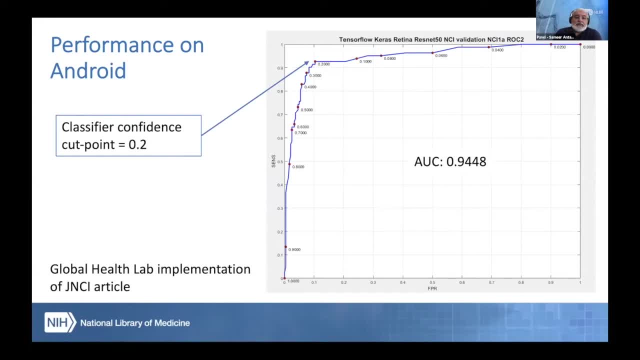 operating characteristic curve which plots the sensitivity of a test versus the false positive ratio on the x-axis, And you want this curve to be as much of a right angle, heading toward the one here on the top left. And, as you can see, this algorithm has a very high area under the curve, or the AUC of 0.94.. 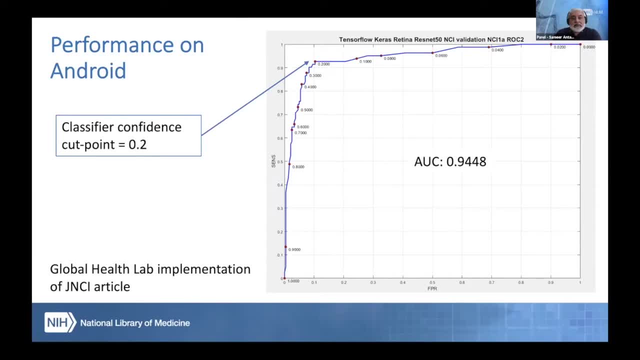 That means it is making very few mistakes. Now. that said, now, this is what if you were looking at many deep learning papers, that what you would be you'll be trying to to track? However it is, this alone is insufficient. It's also. 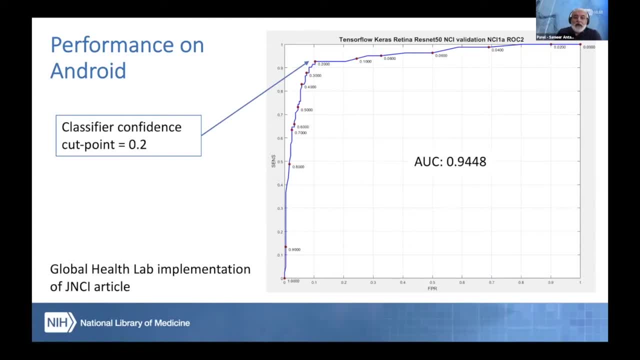 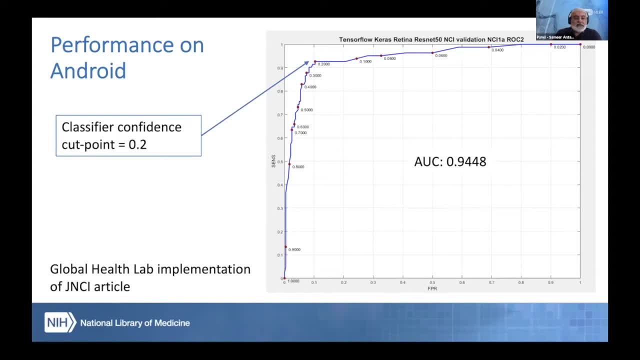 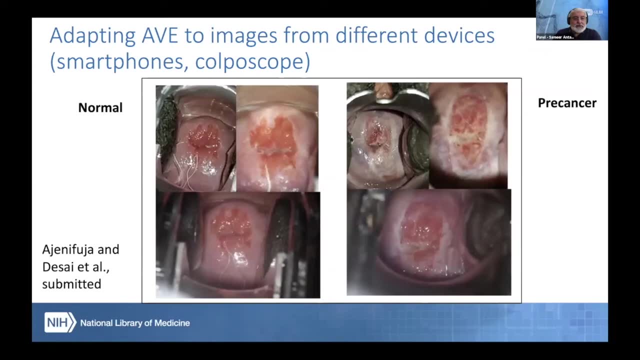 classifier to be very confident to be able to achieve this high a score, And that is a factor that's important. The next slide displays a collection of images comparing normal and pre-cancer cervix. Also important to note is the variety that different cameras can produce on an image, And you would want 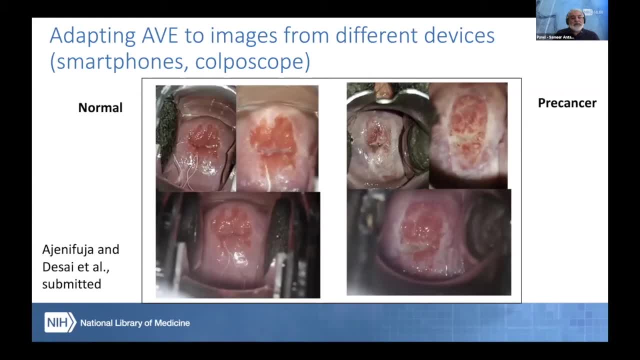 to train your classifier with as many samples from different camera sources so that you have a sense of robustness and reliability in the performance of your AI algorithm, And this also alludes to different kinds of data that you need to use to train your method so that it 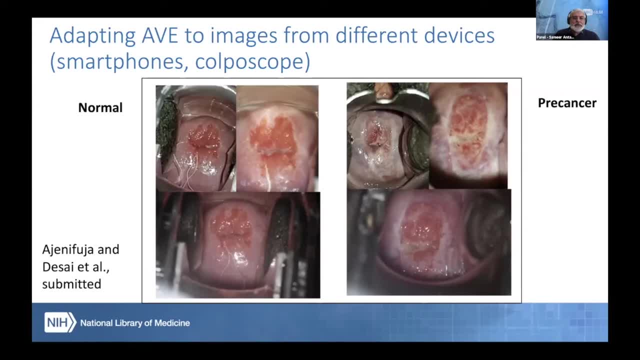 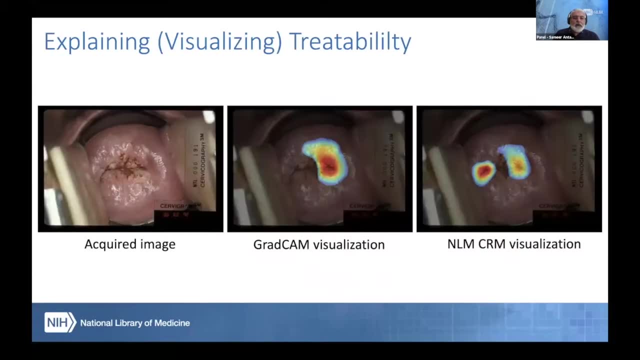 doesn't do very well on a small kind of a set of images, but a broad variety of images that represents the population that you are building the algorithm for. Then you want to be able to explain the to the clinician why the AI thought the image was worthy of treatment In this. 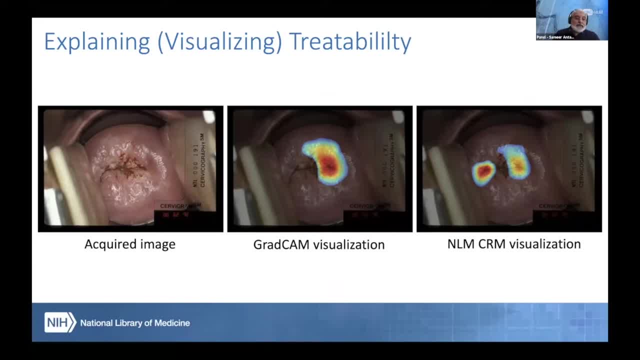 case this is: you're looking at a pre-cancer image. on the left There's a acquired image And the there are two different visualization methods: Grad CAM visualization and NLM-CRM visualization. That means there were two different kinds of algorithm- AI algorithms- looking at this image. both 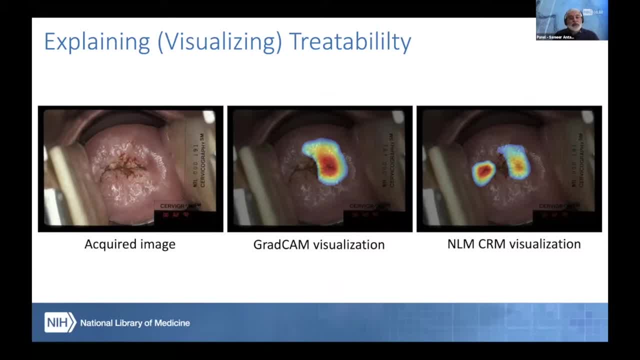 correctly classify the image as deserving treatment. Regions of the image that you're looking at are the regions of the image that you're looking at. The regions on the cervix are highlighted, But, interestingly enough, the each AI algorithm was highlighting a different region of the image, which, of 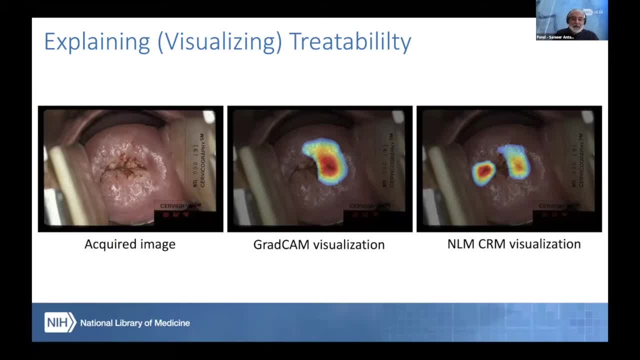 course introduces doubt, and that's why it is still an area of research. But AI can help you classify something correctly, but it's also important for you as a researcher to focus on why it is classifying an image as a case of control, and what region is highlighting that is worthy of treatment. The next: 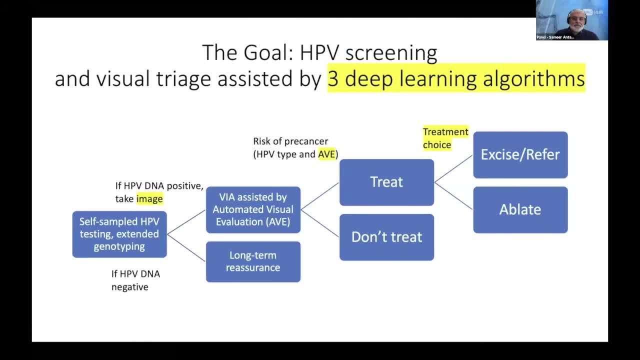 slide displays a flowchart of HPV screening and visual triage assisted by three deep learning algorithms. So if you think about this problem now, from going from the left to the right, you can see an image has been acquired and there is an HPV DNA test done And if the person is has HPV positive, then we would like 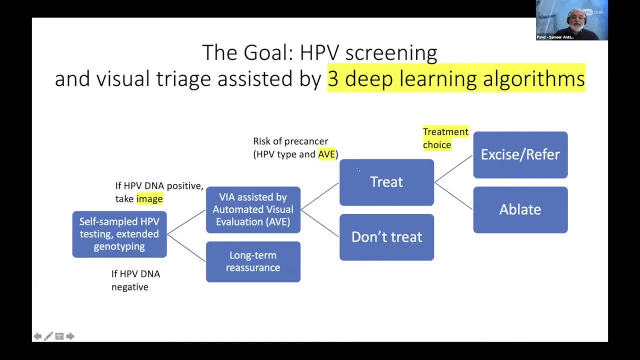 to be able to decide if the person should be treated or not treated. That means the case of control And then, if it is treated, that the process to avoid the Rossi problem. it will take a little six weeks in the next trimester, four weeks. there would be an external algorithm that will be. 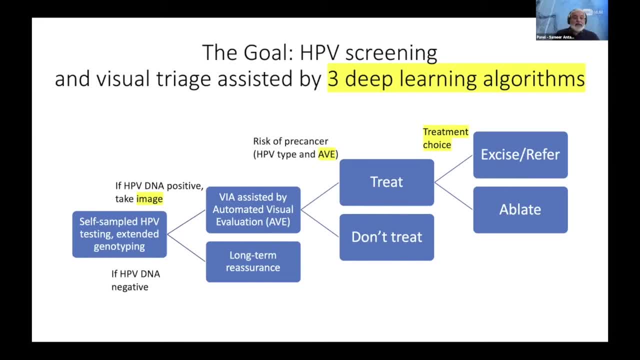 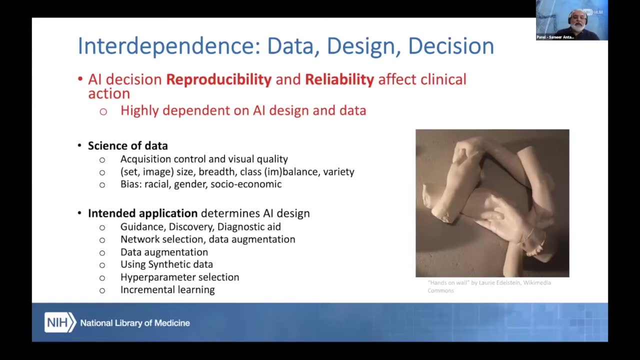 determining if the if the reason should be excised or terminally up later. And so you have different kinds of algorithms that have been trained on different kinds of data: images, as well as HPV data, which may be textual in nature, that are informing the condition to make a better judgement and provide for treatment. So you know, what I'm going to highlight here is the high interdependence in among the data, the AI design and the vision that is used as a secondary ability of the patient to define The platform is as similar as the IQ on this model. In an analogy it is similar, But that means that is apparently not investigate by the tummy, soybeans and also the hair science and everything done to� comes in the whiteward spirit. so data is essentially rather compatible with seniability. 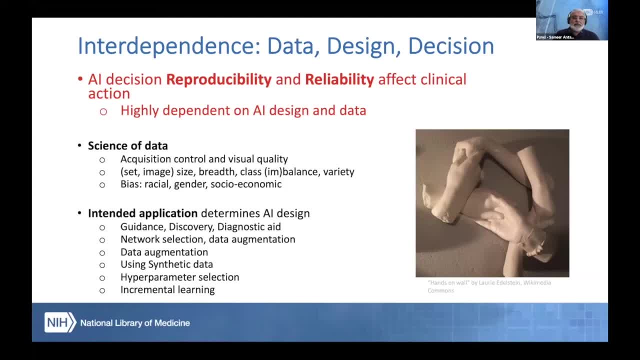 the decision that's produced so that you have a highly reproducible and highly reliable outcome from the AI that can help affect clinical action. and in thinking about this we use the word data science, but I like to try to think of what is it? the science of data, it's acquisition, control and the visual. 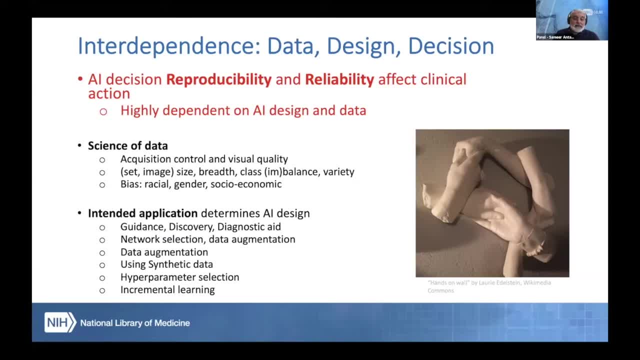 quality of data, how large your set sizes for training. larger the set size, larger the breadth, the variety and this Q in the data. if you have too many controls in too few cases you might not get the representation necessary, statistically speaking, to get the reliability and robustness from the 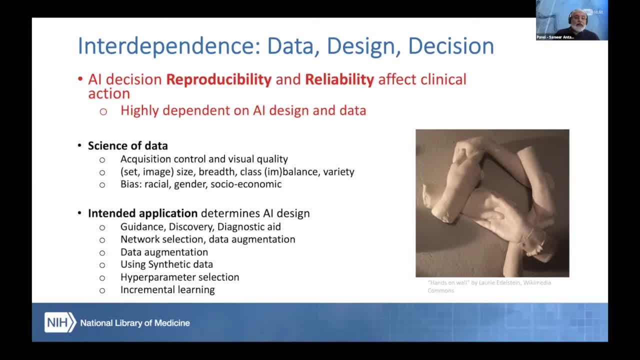 algorithm. you also want to think about any racial or gender or socio-economic variety that might be introduced there which can affect the quality of images. and, in terms of thinking of the AI design, what is the intended application for the AI model and the properties of the AI models? so, 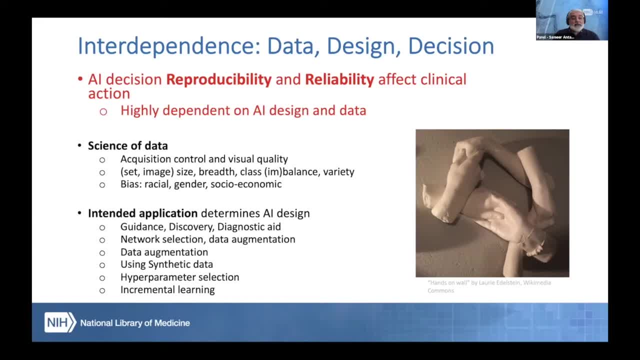 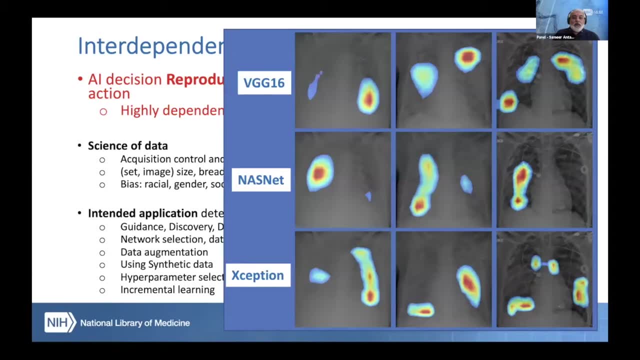 that you can get the right interpretation and the purpose of the technology, and Is it for discovery, which is research, or is it a diagnostic aid? What kind of networks I'm going to use? And this is an example. Dr Antani opens a chart displaying a chest X-ray examined by three different algorithms. 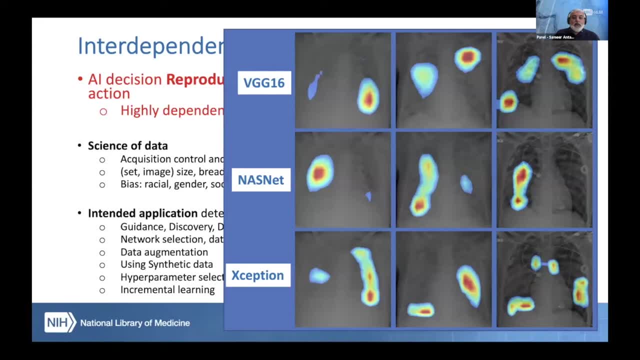 Each algorithm highlights different regions of the X-ray Where you have different kinds of networks. looking at chest X-rays in this example, how each network or each AI algorithm ended up showing different, highlighting different parts of the image. All had disease, yes, and all were correct, but they all were highlighting different aspects. 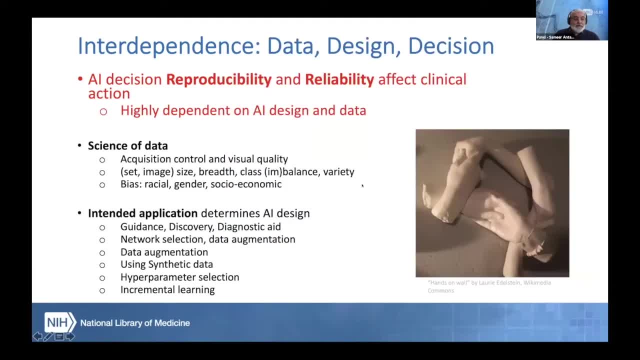 And so the application is extremely important as well. If you're going to be using synthetic data, does it really represent reality? How are your hyperparameters trained for your deep learning algorithm, And would you learn incrementally? That means humans correct machine and the machine learns to adapt and evolve over time. 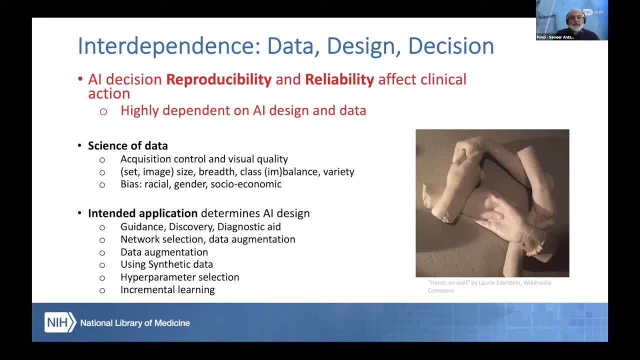 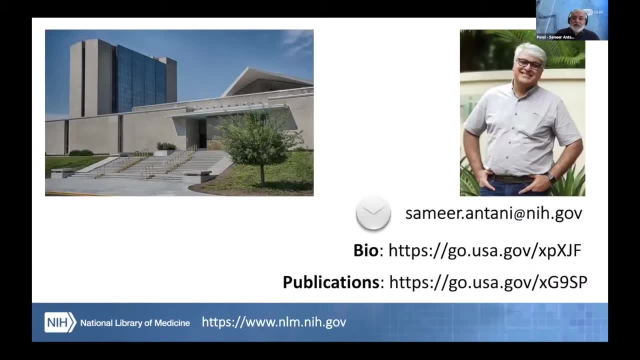 is also a technique that needs to be used. It needs to be researched and considered in designing an AI algorithm. So I'll leave it there And here's my contact information, But before then I invite you to join the network lounge and interact and have a chat. 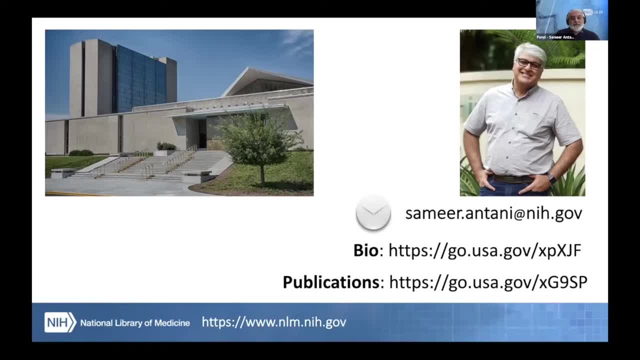 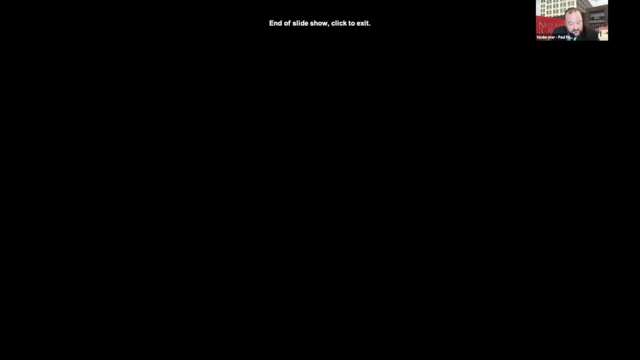 Thank you for attention. samirantani at nihgov bio. gousagov slash- xpxjf publications. gousagov slash- xg9sp. Thanks, Samir. As Dr Sintas is getting her slides up, I'll go ahead and introduce her as well. 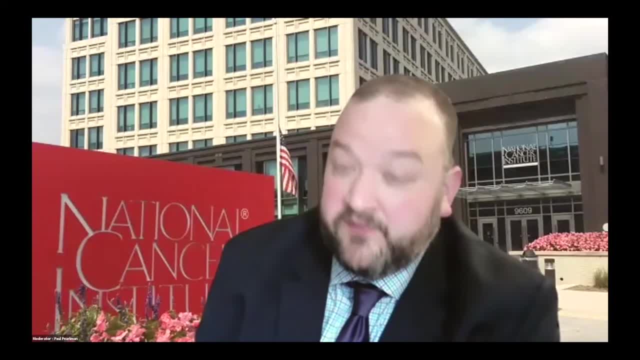 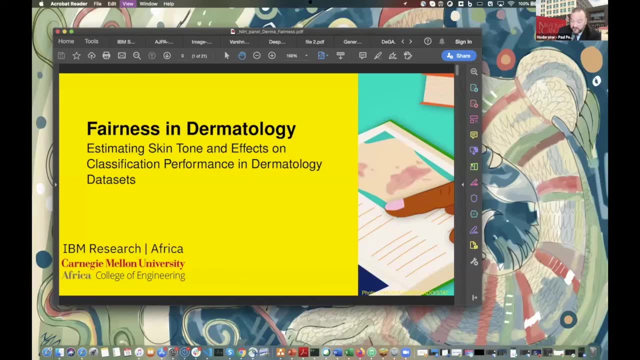 Dr Celia Sintas is a research scientist at IBM Research Africa in Nairobi. She's a member of the AI science team at the Kenya Lab. Her current research focuses on the improvement of machine learning techniques to address global health challenges and exploring subset scanning for anomaly detection on regenerative 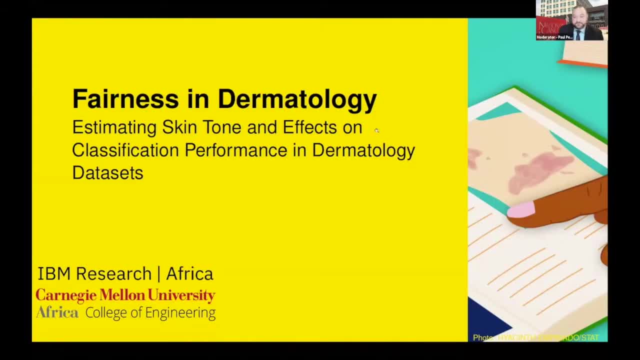 models. Celia Dr Sintas sits in a home office. She opens a slide presentation. Thank you, Paul, Thank you, Thank you. Thank you for the introduction, Good morning, Good afternoon. In this talk we want to discuss fairness in dermatology and how machine learning models. 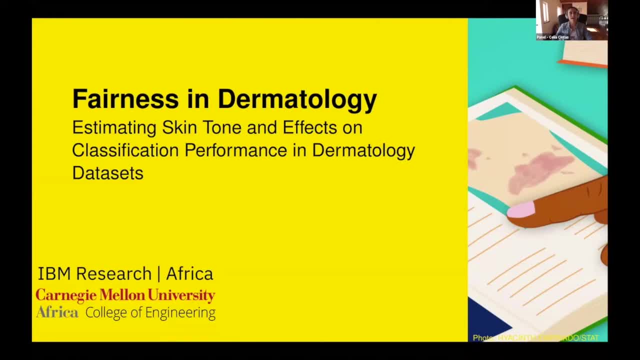 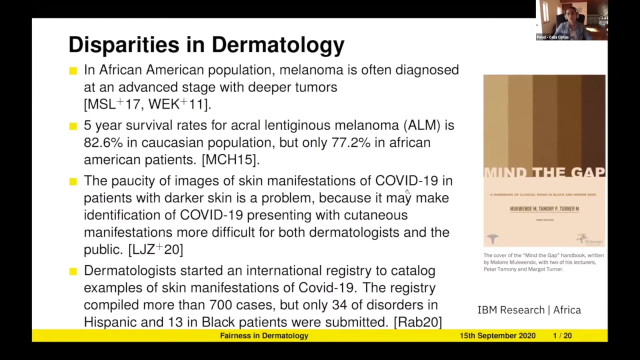 are built for skin disease diagnosis and to see if there is an equal skin tone representation in these data sets. This work was jointly done with the College of Engineers of CMU Rwanda, IBM Research, both Yorktown and Nairobi Labs. We know that in dermatology, as in other medical fields, disparity exists across ethnicity. 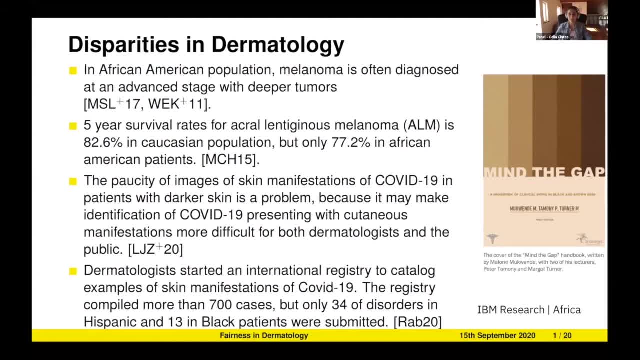 For example, in Black African American population, melanoma is often diagnosed at an advanced stage. Survival rates of ALM are in African American classification populations Due to COVID-19,. dermatology is not a new trend And yet it can be found in many countries. 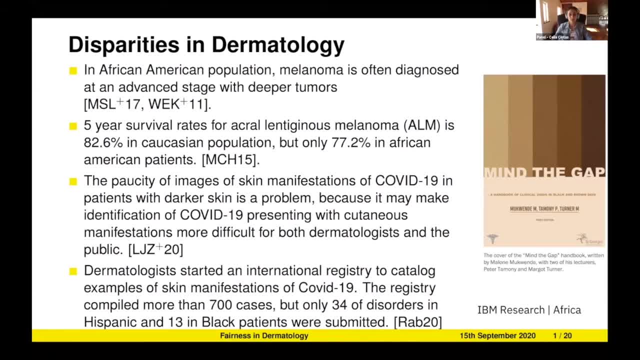 However, many medical institutions and agencies have started an international registry to catalog skin manifestations of this disease. This registry compiled 700 cases, but only 34 of them were Latinos and 13 from African American patients. Professionals are raising concerns regarding the issues in the medical space. 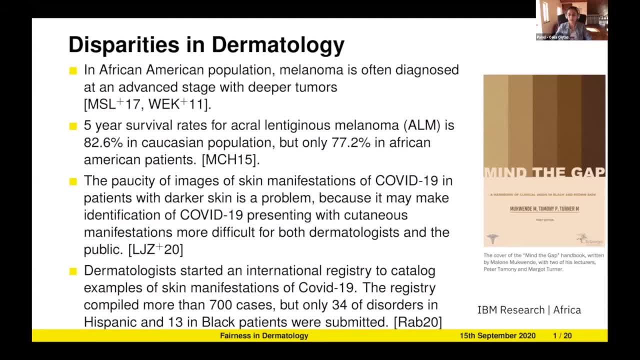 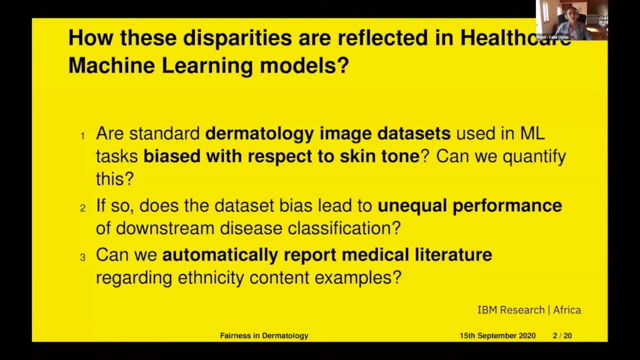 An excellent example is Mind the Gap, a handbook for clinical science in black and brown skin. As we know, machine learning systems may place searching groups of people at systematic disadvantage due to the bias of datasets, So we want to see how these disparities are reflected on the healthcare machine learning 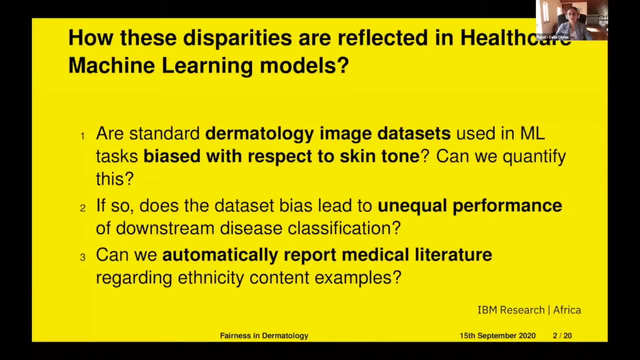 models. First, we want to check if the standard datasets used for machine learning tasks in dermatology are biased with respect to skin tone, and can we quantify this? If so, does the dataset bias lead to an equal performance of the disease classification? 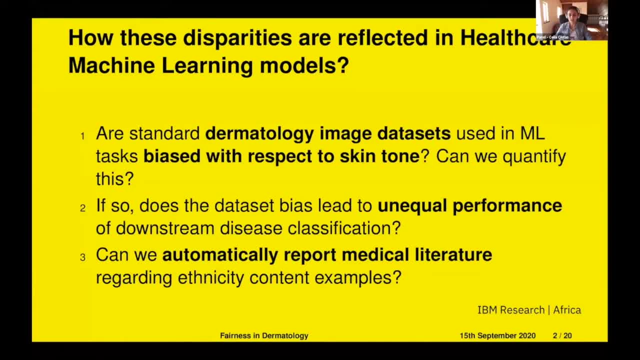 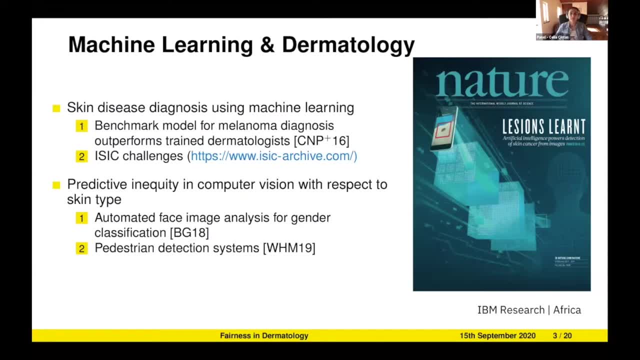 And can we provide an automatic report of medical literature regarding these ethnicity examples? From the machine learning perspective, recent advantage on computer vision and deep learning led to breakthroughs In the development of a new technology. machine learning is a new technology In the development of a new technology. machine learning is a new technology. 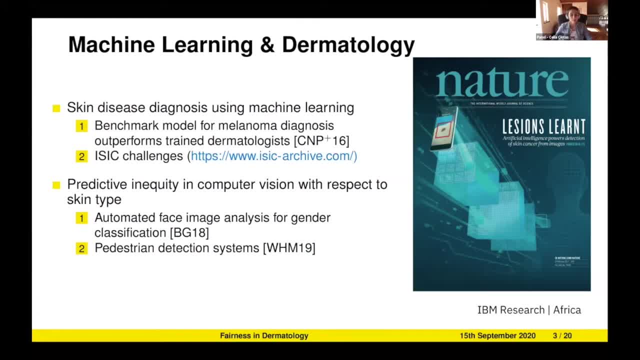 In the development of a new technology. machine learning is a new technology. We have skin image analysis and diagnose, For example in melanoma. we have benchmarked models that all perform training in dermatologists Since 2016,. we have the ISIC challenges that show problems on lesion segmentation, clinical. 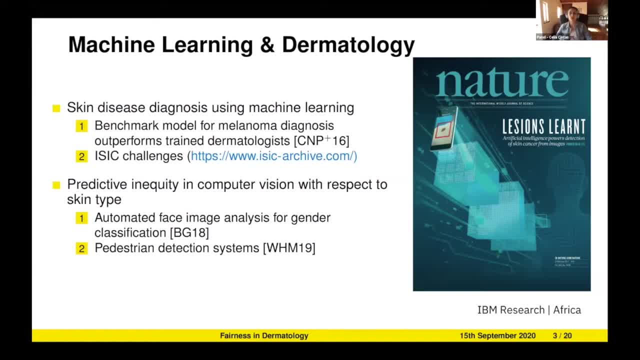 diagnose pattern and lesion classification. On the other side, we leverage work on predictive inequity in computer vision regarding skin tones. This was proposed by Joe Barber. So what we want to propose is a framework to estimate the skin tones and their effects. 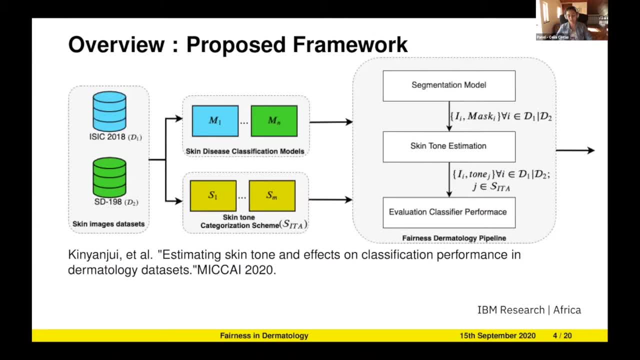 on classification performance in dermatology datasets. This work was led by Tim and Newton. They will be presenting in much more detail at MICAI 2020 next month. But the main idea to have this framework ongoing is based on three steps. First, we need a segmentation model to be able to extract the non-disease skin reactions. 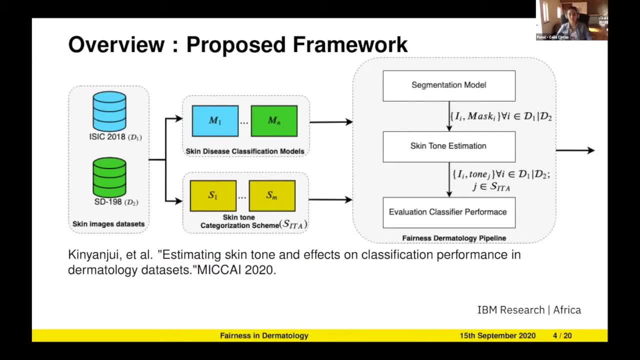 to be able to estimate a skin tone metric And after we have this information we can do a stratified evaluation to see that the skin disease classifiers are working correctly across all the skin tones. So to evaluate the skin tone, we need to use a stratified evaluation to see that the skin 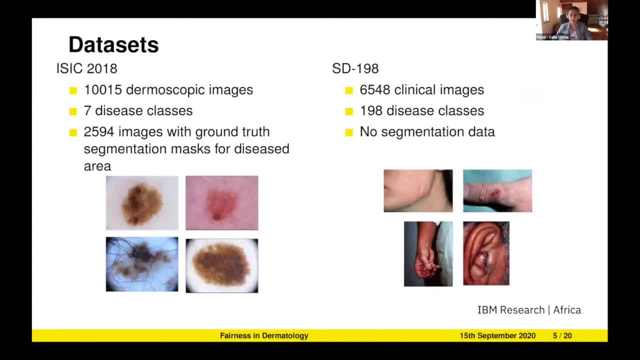 disease classifiers are working correctly across all the skin tones. So to evaluate the skin tone we need to use a stratified evaluation to see that the skin disease classifiers are working correctly across all the skin tones And after we have this proposed framework, we use two common datasets in dermatology. 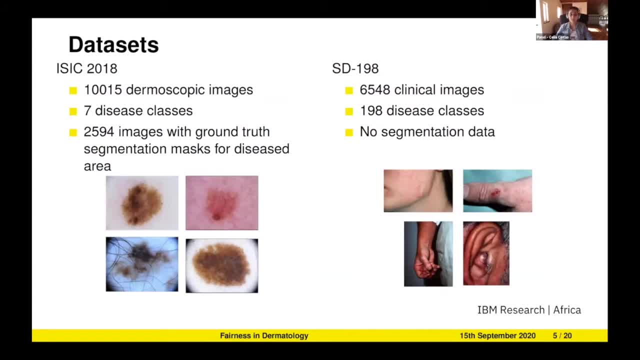 ISIC 2018, with multiple thermostatic images across seven different diseases, labels and a subset of images with ground truth of segmentation masks. In the other hand, we have SD198, with multiple clinical images over close to 200 disease classes, but with no segmentation data. 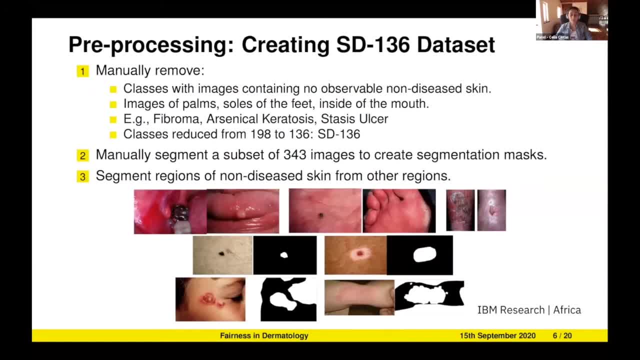 For our purposes we need to be able to estimate the skin tone, to run some manually preprocessing before using them, such as removing classes with images that we don't have observable non-disease skin area, as you can see some examples in the slides over here. 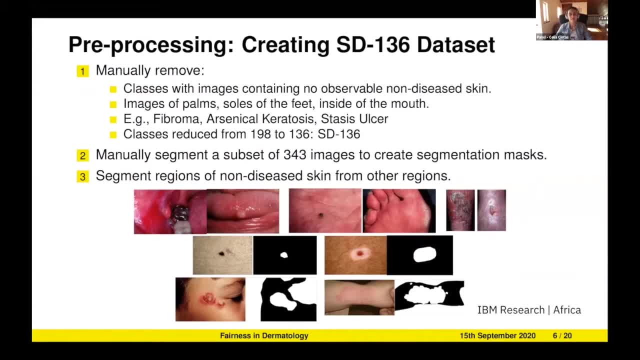 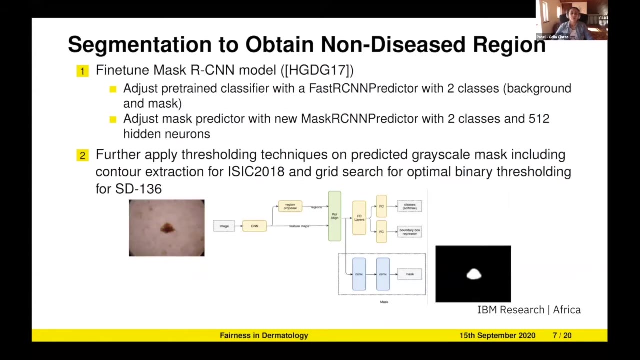 We also remove specific body parts, such as inside the mouth, as you can observe here, And we manually segmented a subset of these images to create our segmentation mass ground truth First, our module for segmentation to obtain the non-disease region is using a mass RCNN. This is 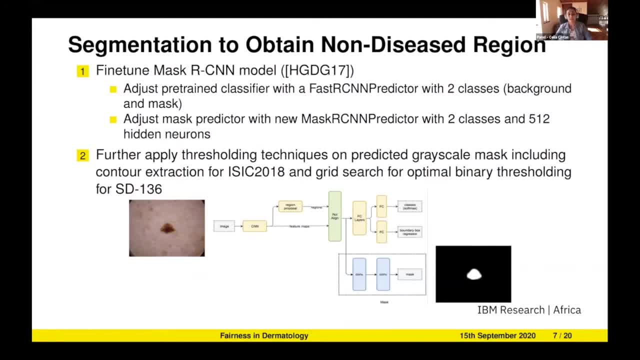 a particular deep learning model that takes as an input an image as an output is going to be a binary class for us giving information of which pixels correspond to the non-disease and which pixels are from the disease area. As our datasets are small, we need to use 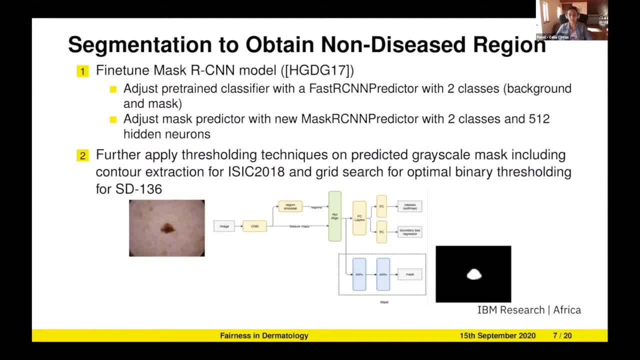 pro trinit models as we can find for mask RCNN. We only need to fine-tune this to our both current datasets. As the output of this network is a grayscale mask, we actually need to apply some thresholding techniques to extract a binary sample. 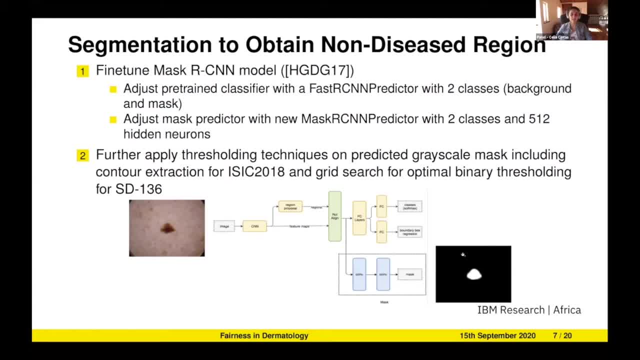 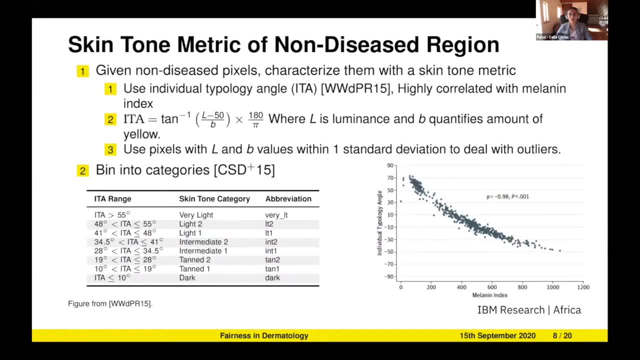 For example, as we see in the bottom right, A photo of a skin mark is transformed into a black and white image highlighting the non-diseased region. After we have our non-diseased region of pixels, we need to characterize them with a skin tone metric. 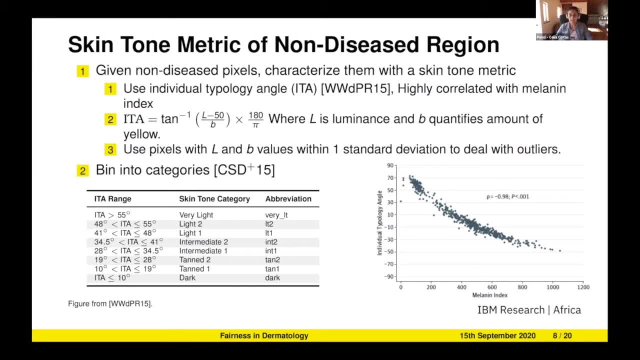 Particularly. we use individual topology angle that is highly correlated with melanin index. as you can see in the bottom scatter plot to the right, The graph measures individual topology angle against melanin index. ATA is an angle metric, so we need to move from pixel information, transform it to another color space and extract luminance information, a bead that quantifies amount of yellow in that pixel. 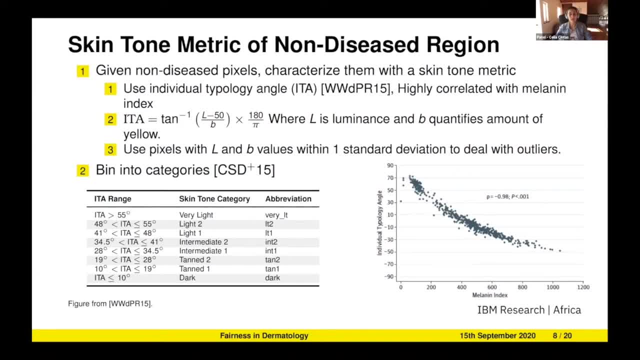 We transform these to an angle and, after we have these ATA values, we can bin them into ranges. Previous work used five different categories to bin these ATA values, but we extended to eight to have a more fine granularity of different skin tones. 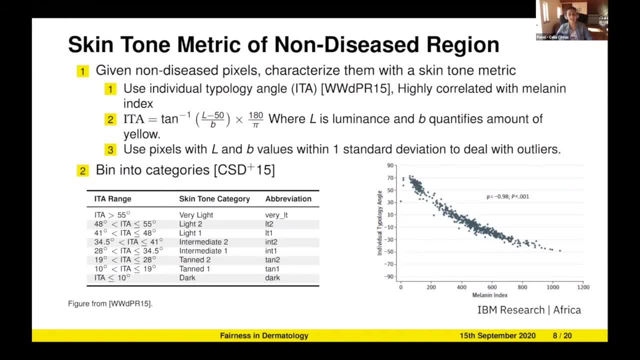 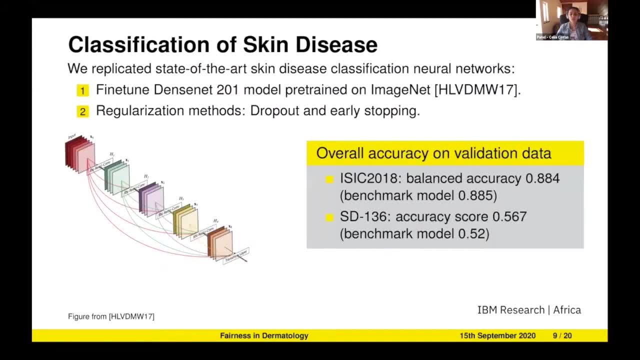 As you can see, lower ATA values go to tanned and darker skin and higher ATA values go to lighter skins. So now we have our skin tone information. Now we want to see if the Skin Disease Classification Model performs well. The Skin Disease Classification Model performs equally across all the skin tone spectrum. 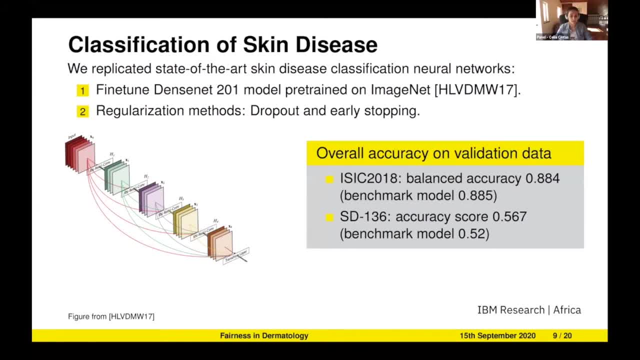 For this we replicated state-of-the-art models. Particularly here we're looking at DenseNet that we use for a pre-trained model on ImageNet and basic regularization methods such as dropout and early stop. You can see that across both datasets we have similar accuracy to the ones in leaderboards or reported in other papers. 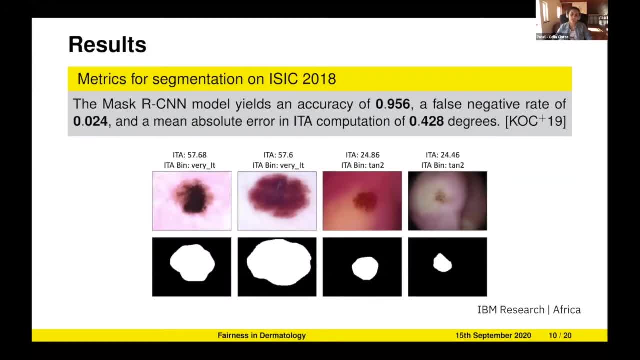 Let's look first at results on segmentation on ICICC 2018.. Here we can see a high accuracy and a low mean absolute error ATA computation. What this means is how good is our method to detect which pixels belong to a non-disease skin area against the other ones? 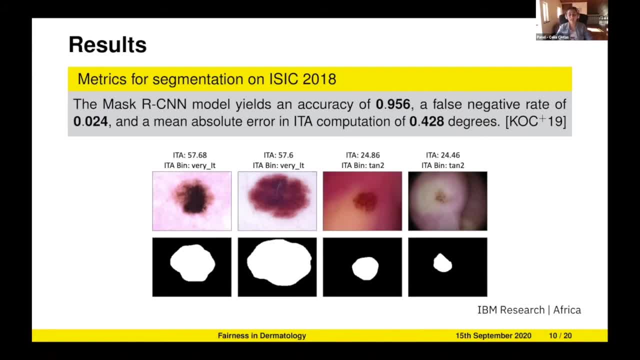 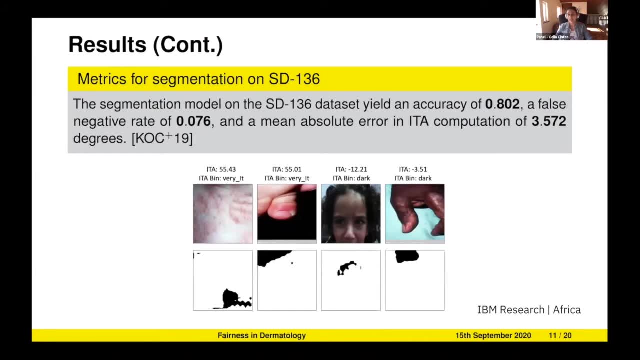 and how well can we compute or estimate the skin tone based on these pixels? For the second dataset, we can see that our accuracy goes a little bit low- 0.802, and our mean absolute errors for ATA computations go high. Some explanations are that this dataset doesn't have any standardized way- 3.572 degrees- to collect data. 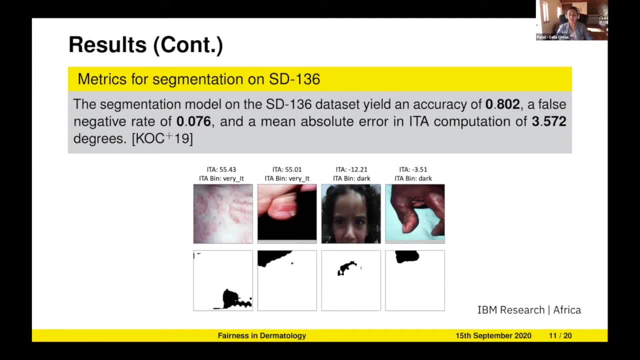 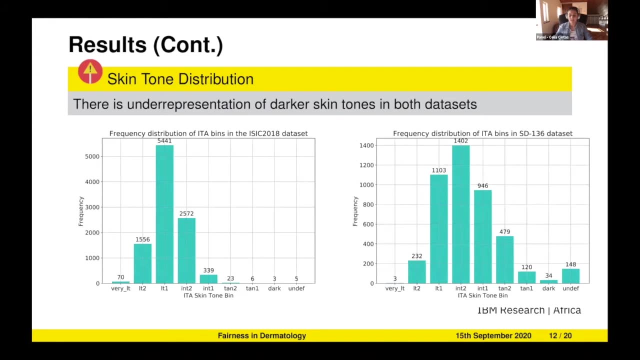 We also have different body parts here, A foot sole, a toe, a forehead and a thumb, And very heterogeneous illumination settings. So further work can be done around this type of dataset. The two skin datasets are highly biased towards lighter skin tones, as you can infer. 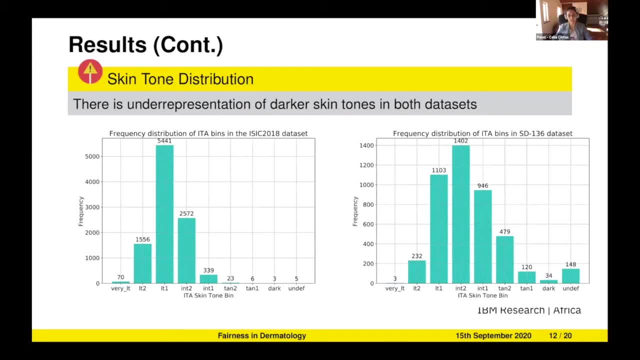 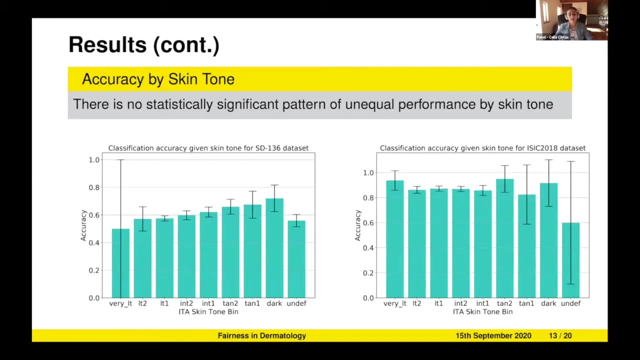 Only a few samples for tanned and dark skin in both available datasets. So all the dermatology algorithms that are being trained currently are heavily on these ranges of skin tones, But the bias in the datasets doesn't seem to affect the classification results for each of the skin tones. 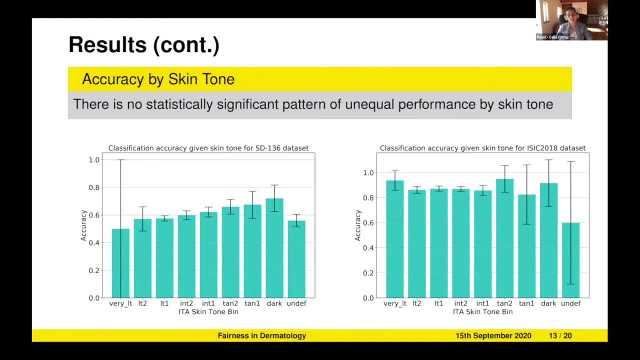 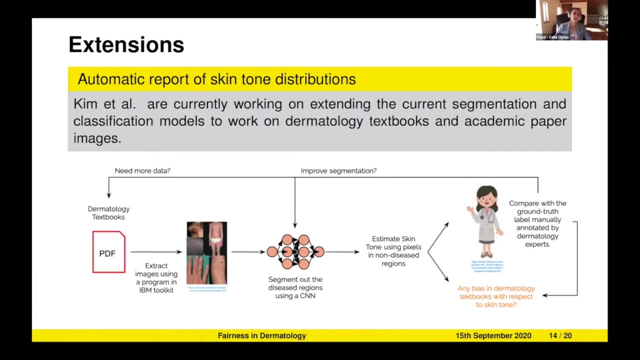 But the caveat to these results is a very small sample size for darker skin tones. So further research should be done, augmentating this part of the dataset and re-running some experiments. Some extensions that currently Hannah, one of our members, is working on, is: how can we use the same framework but to dermatology textbooks? 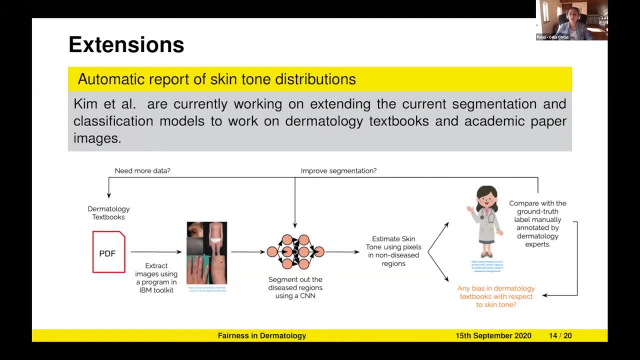 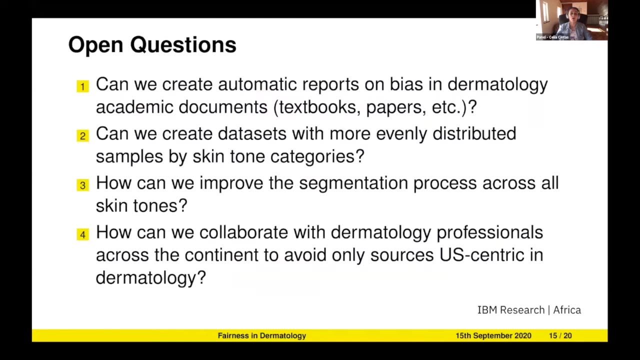 So currently our framework runs for dermatology datasets, But we want to expand these to textbooks or academic papers So professionals can have information on the representation distribution of examples in these documents. We still have a lot of work going on. We are wondering how can we create datasets with more heavily distributed samples across the skin tone categories. 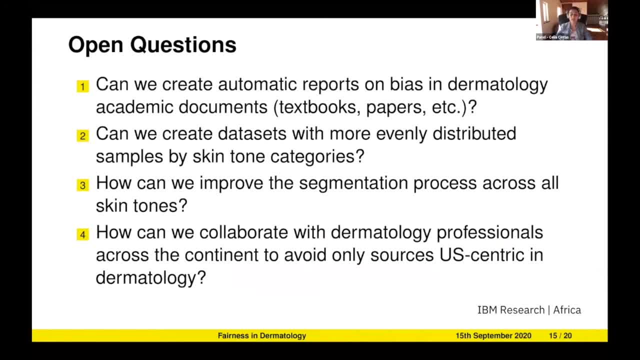 How can we improve the segmentation process in the wild images such as textbooks or papers, And how can we collaborate with dermatology professionals Here in the continent to avoid only sources for US centric in dermatology? Here are all my colleagues that are working on fairness and different health care applications. 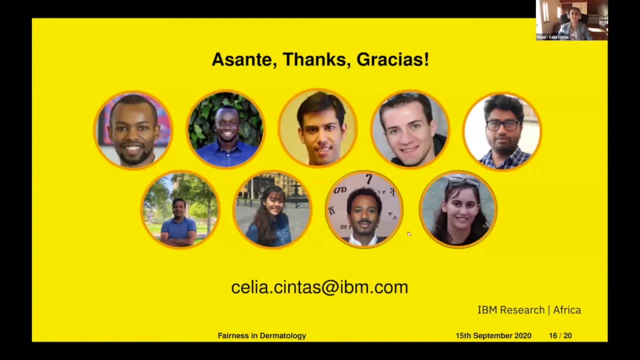 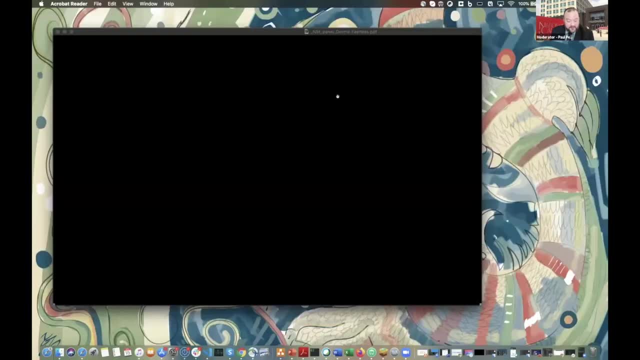 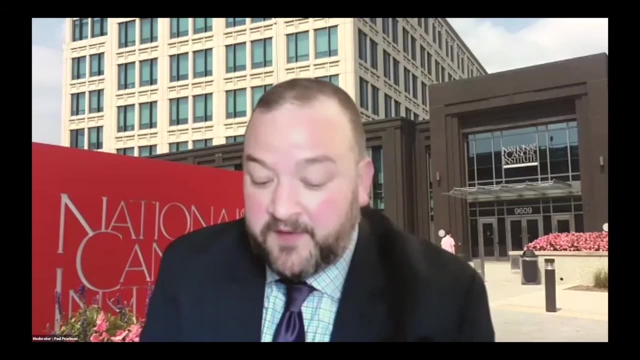 Thank you so much for your time. Thank you, Celia. While Dr Milner is bringing his slides up, I'll go ahead and introduce him as well. Dr Dan Milner is the chief medical officer for the American Society for Clinical Pathology, based in Chicago. 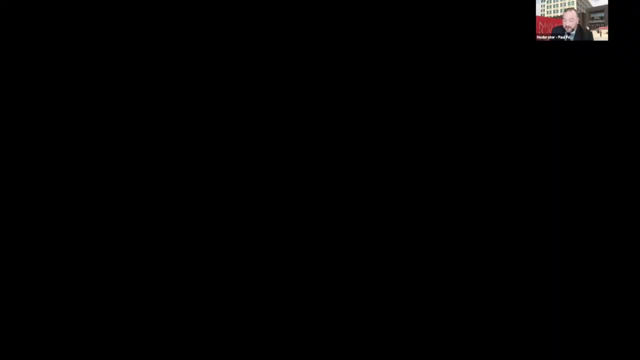 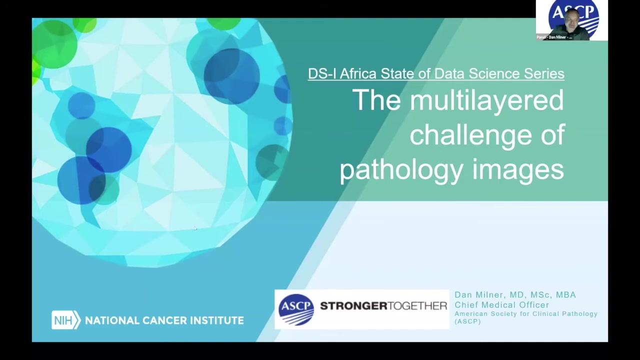 And works with more than 20 countries on pathology capacity building, including telepathology, and personnel. Dr Milner's backdrop is the ASCP logo. He opens a slide presentation. So this morning, thank you so much to my fellow speakers who have set a wonderful stage for what I'm going to discuss. 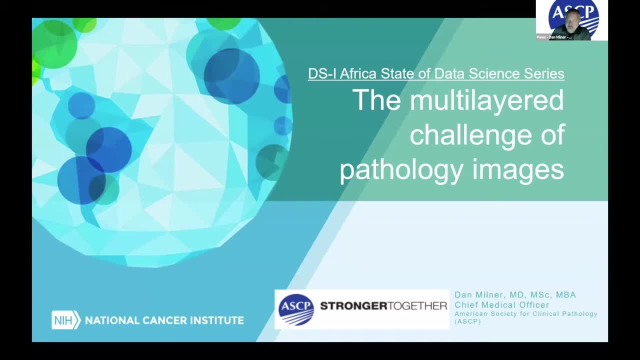 And what I'd like to do is dive really deep into pathology very briefly, because this is a rich source of images. Someone in the Q&A has already asked or pointed out that, So I just wanted to go into that in a little bit more detail. 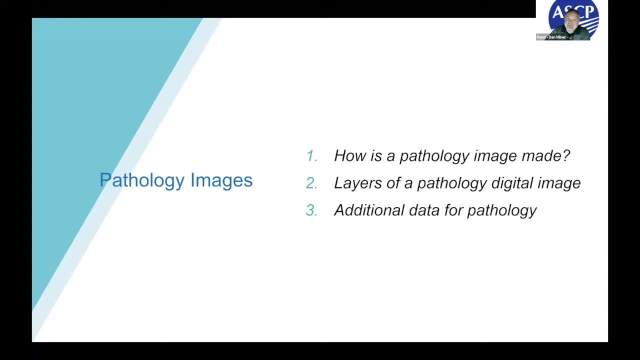 So to begin, I just want to talk about pathology images, And first how is a pathology image made, Which I think is important for everyone in the audience to understand the complexity of that process before we actually get to that image. Then talk about the layers of a pathology digital image, from the lowest level resolution to the highest level. 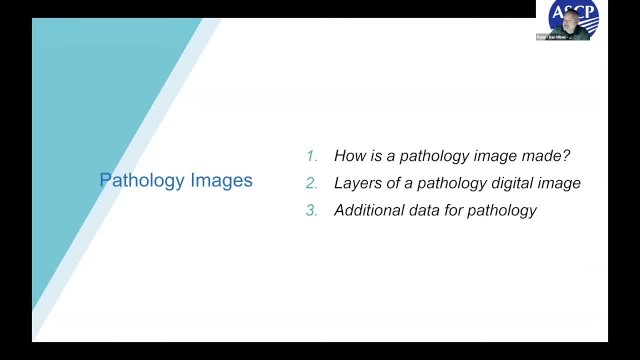 And what that means for research implications, And then, lastly, talk about additional data, which has been touched on briefly by my fellow speakers. So let's talk about a pathology image from a patient to a data file. So, for those of you who are familiar with pathology, this will be a little bit of a review. for those of you who are not, 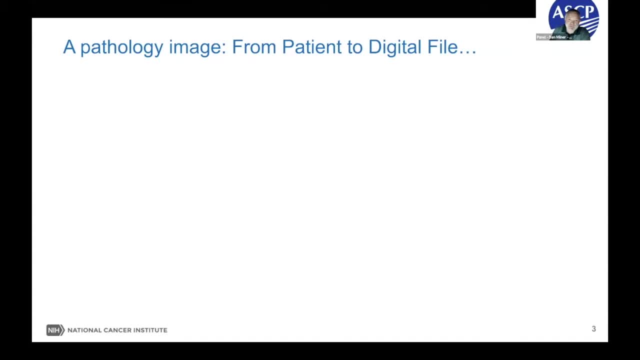 Keep in mind that there are three main sources of, or three main types of samples that you may use in Africa for pathology. Those are: cytology, which is the study of cytology- This is the study of cells. Surgical pathology, which is the removal of tissue from a live person to make a diagnosis of cancer or an infectious disease. 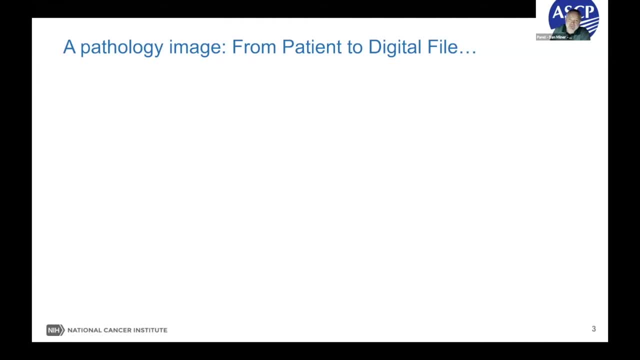 And then autopsy pathology, where you remove tissues from a dead patient in order to make an anatomic diagnosis after death. And that whole process- here illustrated by an example of taking a sample from a breast tumor- is not dependent on pathology. It's dependent on the clinicians, the proper way that the sample is taken, handled, processed, labeled. 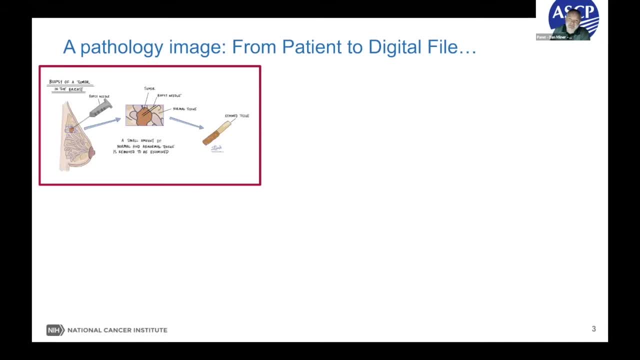 It's dependent on the pathology lab, And so the way that the sample is fixed before it is sent to the pathology lab can have massive impacts on the quality of the image that's produced at the end, And so this is a component of research or a program that has to be well understood and documented. 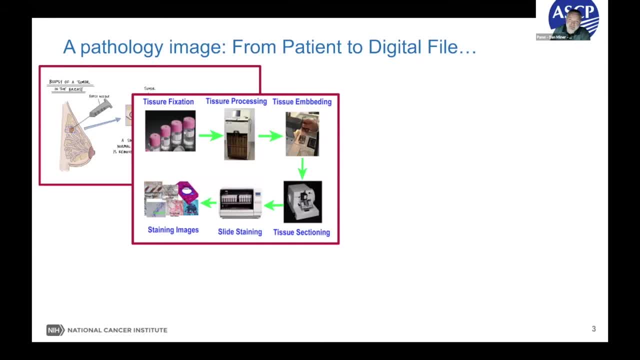 Once that sample is collected and sent to the laboratory, it's in a fixative which has to be of a certain type. It's put on a tissue processing system. It's then embedded in paraffin wax. That paraffin wax block is then cut with a razor to produce a slide. 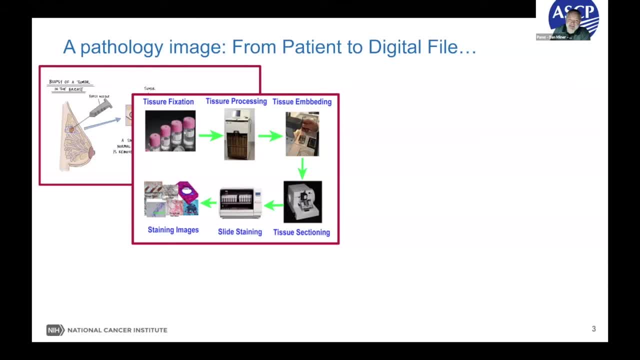 It's then stained using a variety of different staining techniques And then you have a stained image And this is the classic histology slide or even cytology slide that a pathologist would look at under the microscope and read. And, as you can see, there's already a lot of steps in this process that can go wrong: if fixation is wrong, if the tissue processor isn't functioning properly. 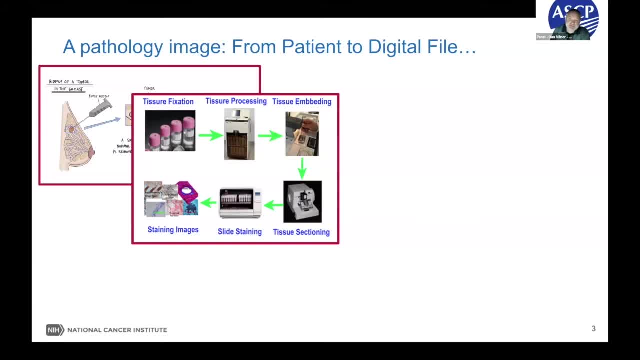 If the tissue embedding isn't done with highest quality, these images are not going to be ideal. Now we have our glass slide And we need to scan it to create an image. We need to create a whole slide image or a digital image that we can then analyze with a computer. 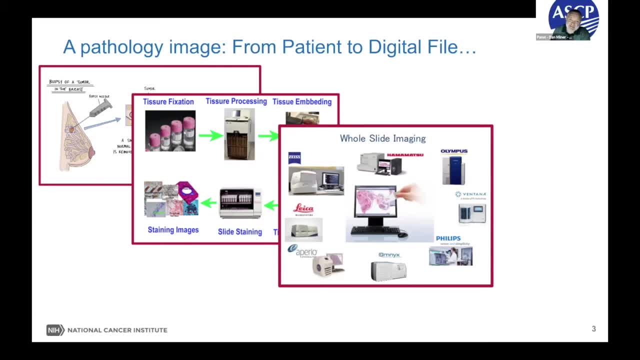 Well, at this point, we have lots of options. There's not just one way to scan a slide. There are at least a dozen different companies that make whole slide imaging systems, Such as Zeiss, Hamamaru, Olympus, Philips, Omnics, Aperio and Leica. 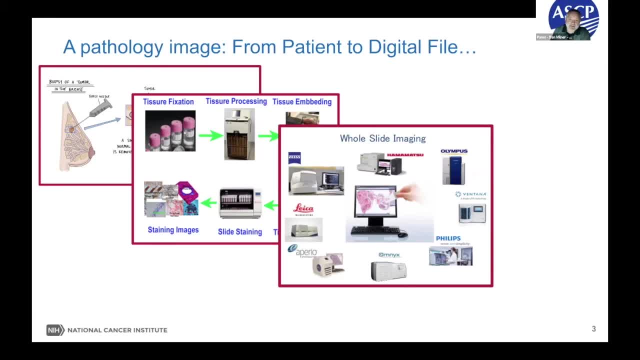 They use different background processes. Some of them, like Philips, use Blu-ray technology. Most of them use basically a microscope inside the system That scans either by moving the slide or moving the microscope objectives, And they can scan at different resolutions. They can scan at 20x or 40x and have optical zoom up to 80x or 100x. 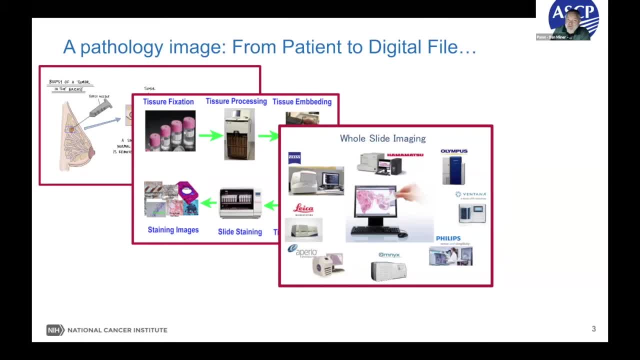 But all of that is variable and needs to be understood before you try to use this for research. And then, lastly, once you have scanned that image using that system, you now have to look at that image or study that image, And there are a variety of viewers at that point. 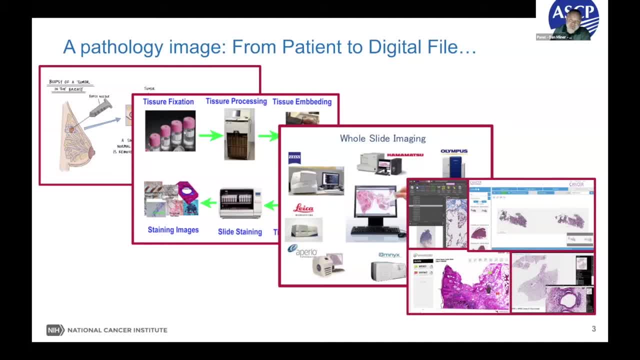 Each company that makes a scanner will have a different software viewer. There are some agnostic viewers that are available as open source software, And all of those use different file formats. They process the image slightly differently when they open it, And so those are other aspects that need to be understood. 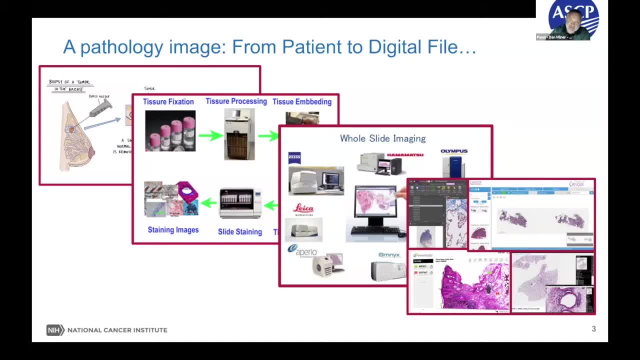 So, just to recap this, as we go from the patient to a digital file of a pathology image that we want to analyze in our research, there are, all along the way, steps around quality, around assurance That you want to make sure you're keeping up with and accounting for in order to make sure that that final image you're looking at is of high quality. 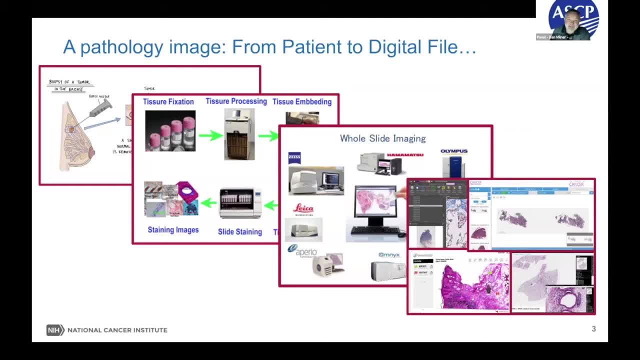 And this is not something you can take for granted. If I had the time, I could talk to you for hours about the challenges of pathology in Africa. This is what ASCP works on. We work with multiple laboratories to help improve their quality, to provide equipment, to provide immunistic chemistry. 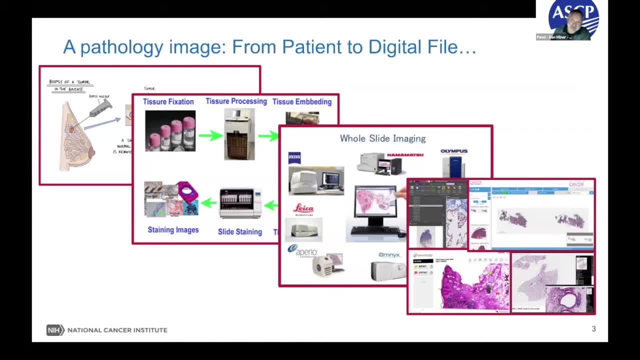 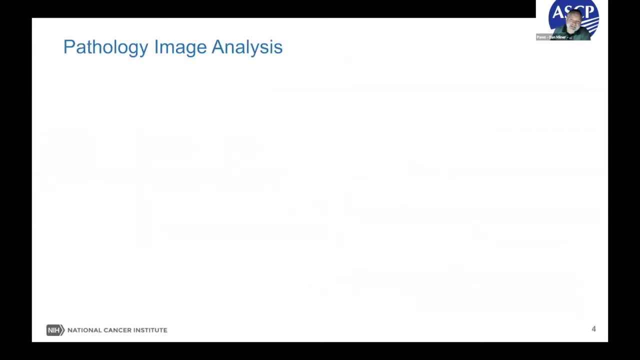 And the goal is to produce high quality images for diagnosis, but also high quality images for treatment, High quality images for research. What about pathology image analysis? Now, my colleagues have shown you radiology gross image of the cervix as well as skin. 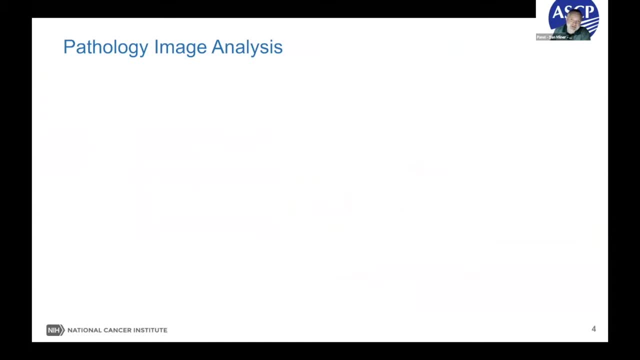 And those are very complex, as you can see, the process that they were using And pathology is slightly more complicated than all of them for a couple of reasons. So if we think about the image that I'm showing you here of four boxes- two red, one blue and one black- 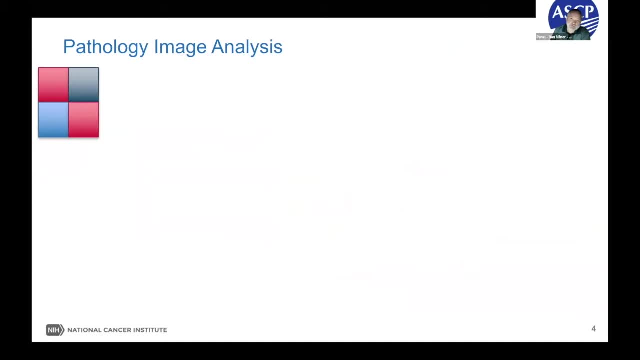 and we want to teach a computer how to figure out what those are, the orientation, et cetera. it wouldn't be that complicated, And this is very similar to trying to understand a radiological image which is in black and white. 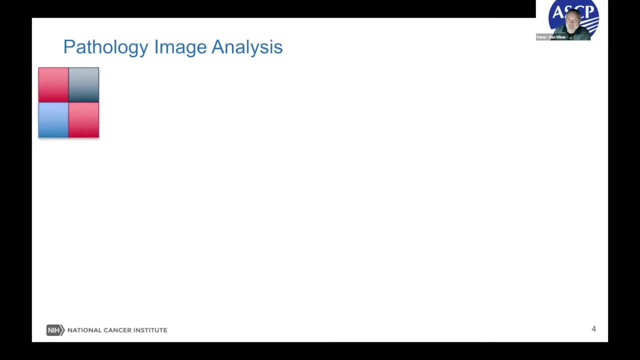 or possibly even a skin image which is almost two dimensional the way that you look at it. But with pathology we have all those different colors, but we also have layers. A histology slide or even a cytology slide can be many microns thick. 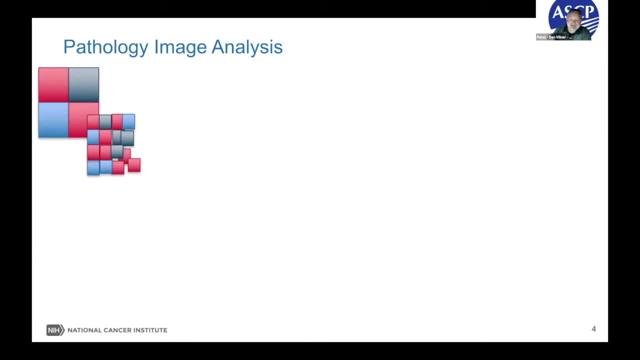 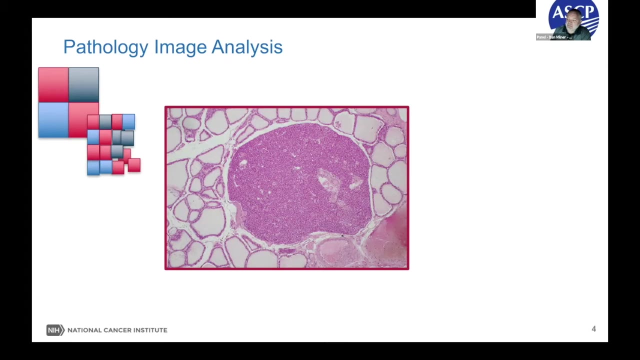 And so from a given image, the camera can actually take multiple layers and have multiple slices or Z stacks that we have to look at And in research you may need to account for that. Then, when we finally look at our image, for example here, this is an image within the thyroid of a parathyroid- something very simple. 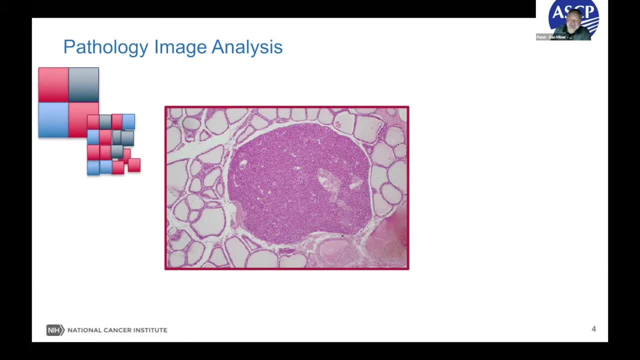 You can see at this low power that the surrounding tissue is different and the tissue in the middle is unique or is of one type. And for a pathologist, they look at this slide and instantly think, oh, that's thyroid with a little parathyroid in it. 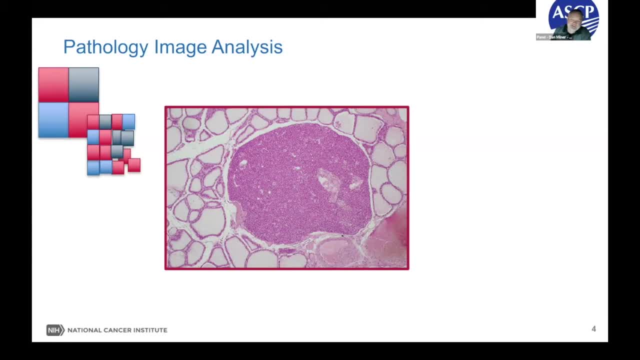 But for a computer it first starts and says: oh, there's a light area, there's a dark area, And then it does pattern recognition to figure out where it is, And then it can finally say this is likely a structure within a thyroid gland. 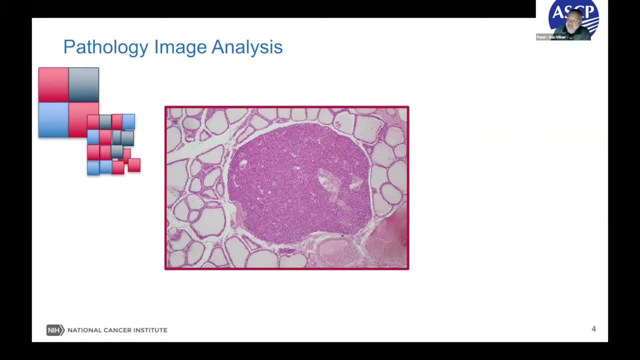 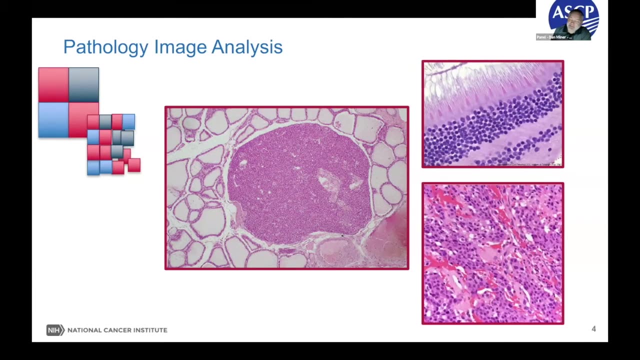 And looking at the color of the nuclei, et cetera, it can determine, using AI or comparative metrics, that this is likely a parathyroid or some other structure. But this is at a low power. If we now zoom in to a higher power, as in these two images, these are from completely different cases. you can see that in the top image there's a lot of structure. 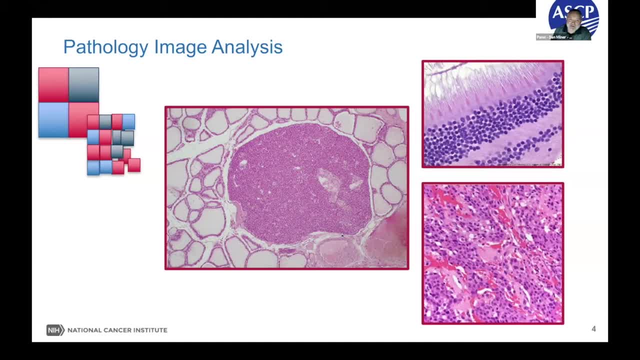 This is a very structured structure. It's got orientation, It looks very unique and almost like something that anyone should be able to recognize with a little bit of training, And this is, in fact, part of the retina of an eye, And so you can see the rods and cones and different parts of the eye. 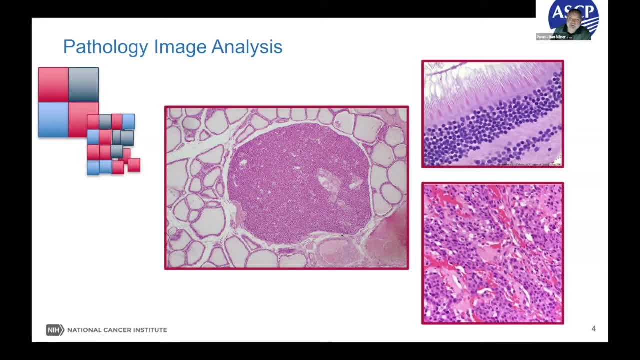 But the lower image of histology is just from a random part of a tumor And what you notice is that there are some blood vessels in there. That's the red stuff, There's some purple nuclei, There's some pink material, But it's completely disorganized. 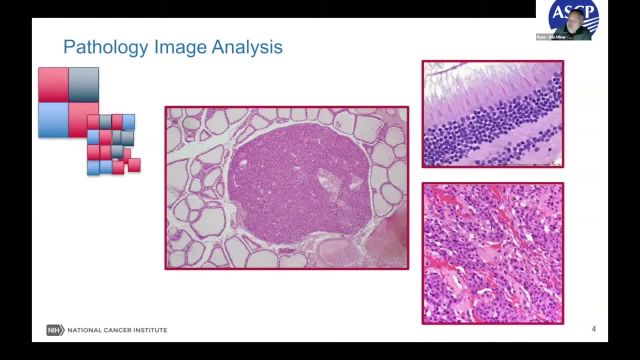 We don't have that structure that we see above, And it's very high power. This could come from the slide in the middle, but it's such a high power that we don't have a lot of context around it, And so when a computer or an AI algorithm is trying to learn, it can learn at low power, but does it have that same learning, or using the same learning techniques, at higher power? 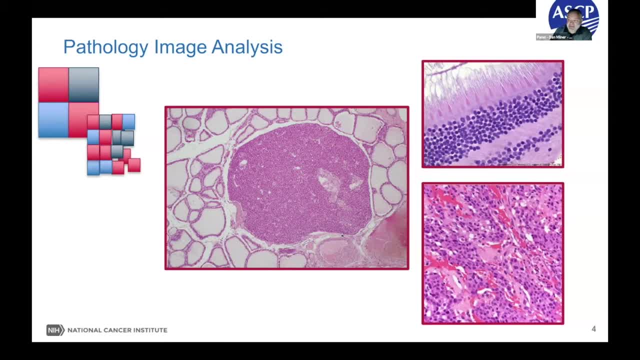 It's very important to understand how you're going to sort of approach a case and what you want to learn from it. So just to recap that, If we just wanted to have our computer or our AI algorithm recognize that this was a parathyroid within thyroid tissue, you can imagine that it's not as complicated as trying to teach it to recognize, for example, the orientation of the rods and cones in the retina. 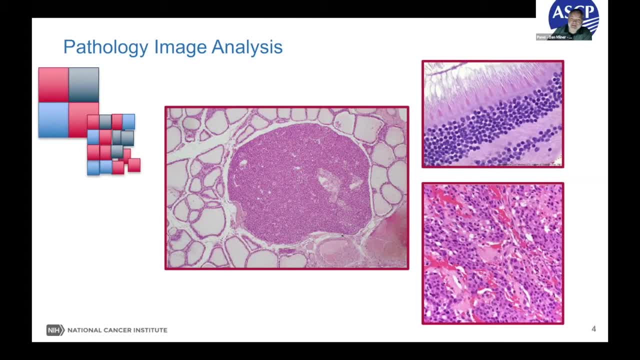 Or even to tell you what kind of tumor that is on the lower left or the lower right, because of the lack of orientation, the lack of structure. The AI really needs to study those cells, to study those nuclei and even look for details that we may not know about. 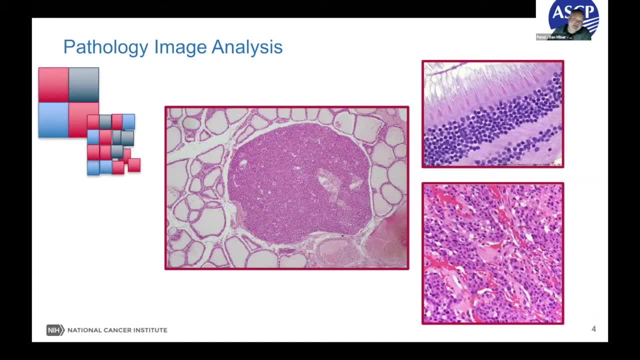 And even look for details that we may not have in what my colleagues have been calling the ground truth. That is, a pathologist may look at that slide and say, oh, that's a- you know X tumor and I recognize that from morphology. 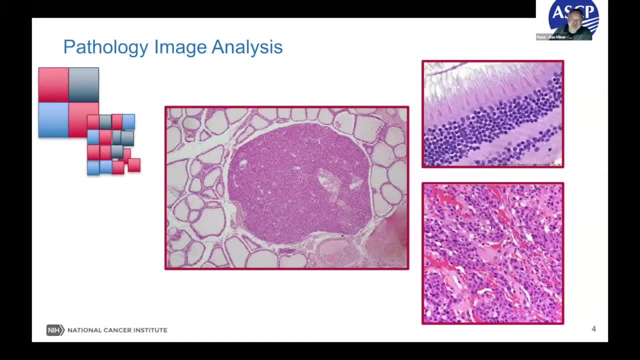 But they may be incorporating all the information about the patient- what the low power view looked like, what the high power view looked like, But AI is only looking at this one image and has to be able to also integrate that data. And then, lastly, there's all of the additional data that goes along with the pathology. 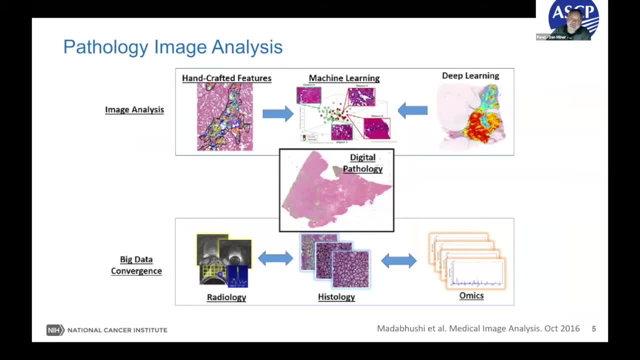 So we've got that digital histology in the middle which I've just walked you through, But then there's all the ways you can analyze it. You can do handcrafted or hand annotated features, where a pathologist or a technician goes in and marks off different areas. 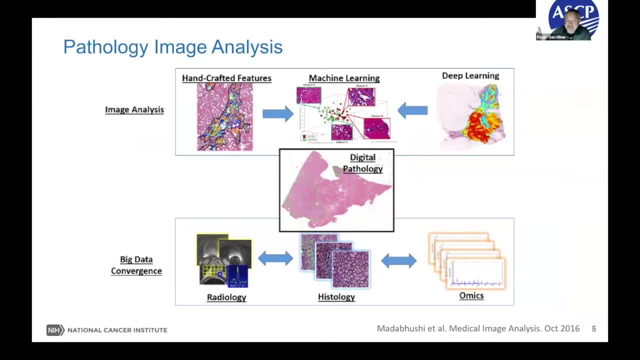 You can use machine learning, where you, as Celia was describing, where you feed the machine thousands and thousands of images which have already been annotated And then it learns to interpret new images that it's never seen before. And then you can do deep learning or neural networks. 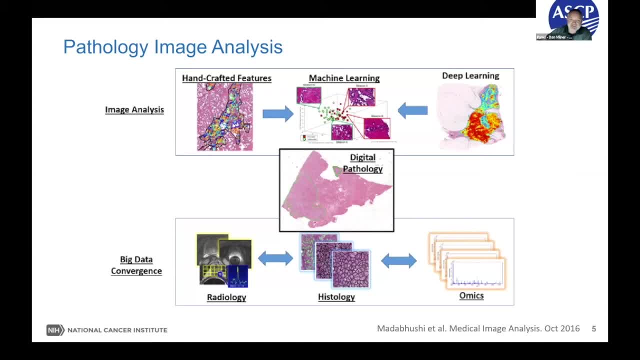 Sameer was talking about where you teach it to understand the interactions of cells on a slide using multiple different layers of information, For example, different stains or different color techniques. And then, as we were, Michael was talking about, you may have radiology data that you need to correlate back with histology. 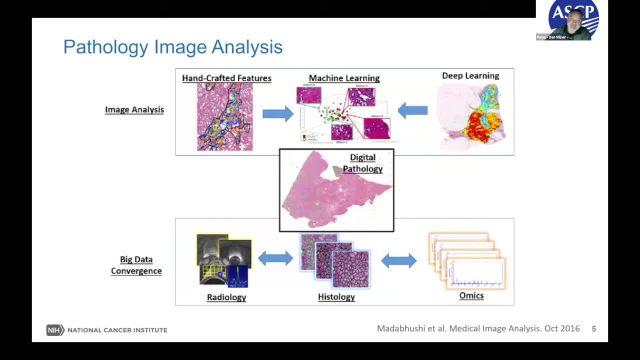 And he was referring to histology as an example of ground truth to base on radiology, But understand that histology also needs a ground truth or a basis to understand exactly what's going on there. And then there's all the omics data. 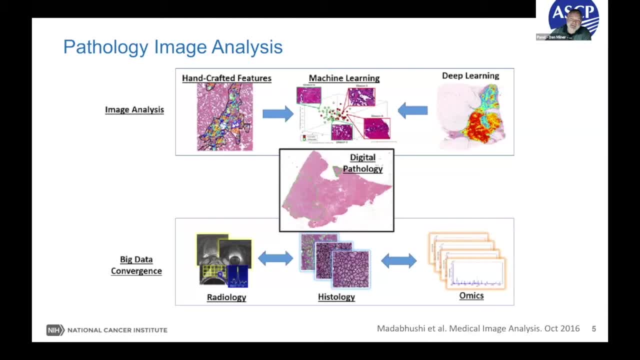 There's transcript, omics, any other kind of proteomic data, et cetera. It has to be related back to that histology. So there's two aspects of that. One is that histology must be high quality and absolutely perfect for all of these things to be integrated correctly to give you the best result. 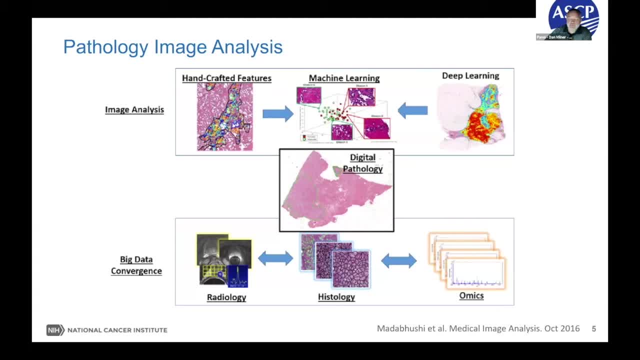 But then when it is really exactly what you want it to need, or what you want or need it to be, it needs to be integrated correctly to all of this data using annotation and tags and case tracking. And then the second aspect is that your omics data on RNA expression is matched to the proper set of histology images. 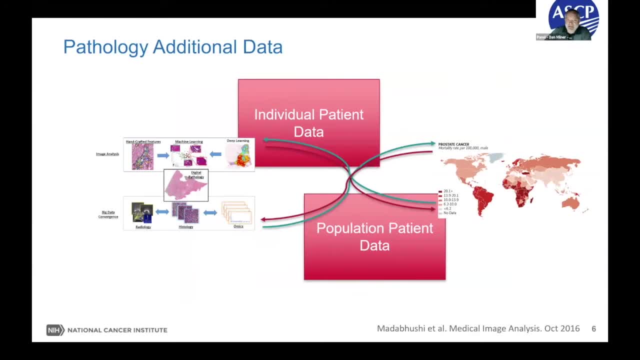 And then, when we think about all of this, there are two ways that this data can sort of come together, especially in data science or big data projects. We can think about individual patient data where we have, you know, 10,000 patients from multiple countries that all have a same cancer or similar cancer or infection. 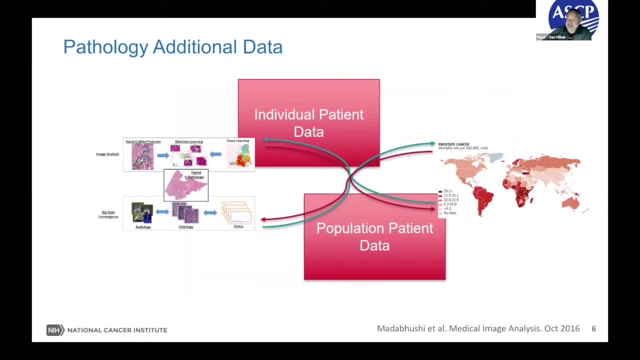 And we're feeding all the data about those patients into a database And that's sort of creating working models or AI models for how to do things. Then there's also population, patient data, the demographics of the population, epidemiology, cancer registries, et cetera, which may be anonymous data. 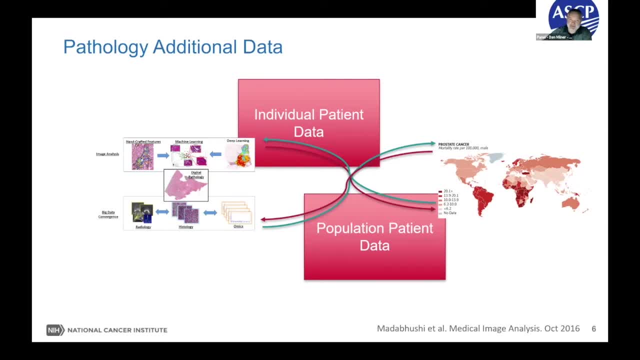 It may be more about a region or a population than it is about individual patients, And that's important because, for those of you that are thinking about projects that are going to have impacts for policy, or how you are going to inform the government of spending money, et cetera, you want to think about population, patient data. 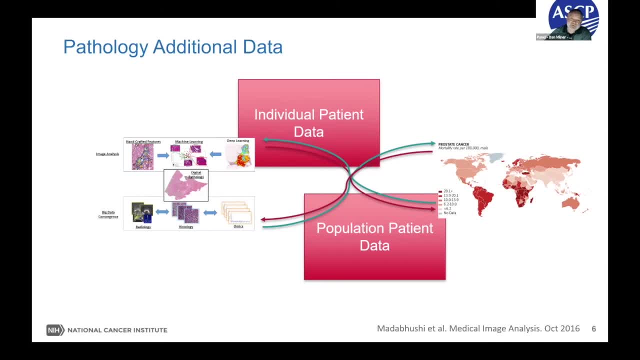 Because you're trying to do what's best for the population. But if you're in a program or you're doing a clinical trial or you're trying to treat patients, you're going to look at individual data to say what are we learning from this system, to go back and help that one patient as we move forward. 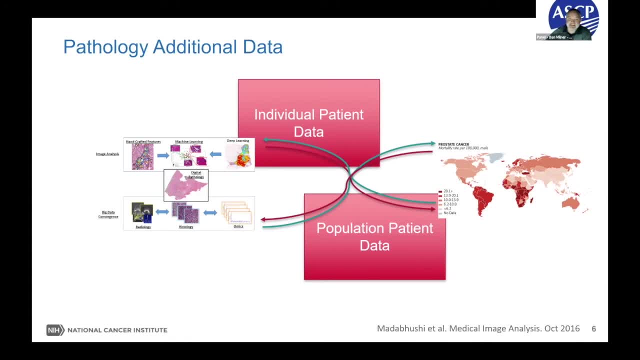 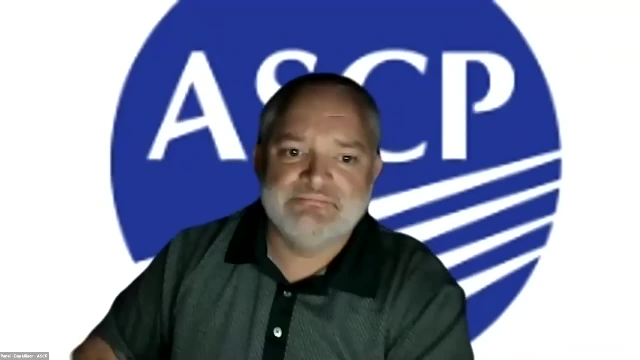 And that uses very similar techniques and integrates the data in a similar way, but it's just a different level of analysis and a different level of understanding. So I think with that I will close and turn it back over to Paul. Great Thanks, Dan. 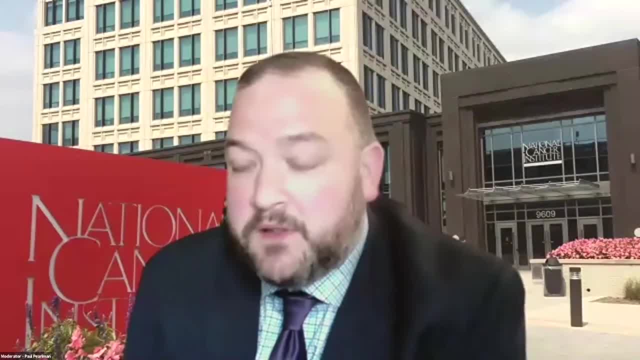 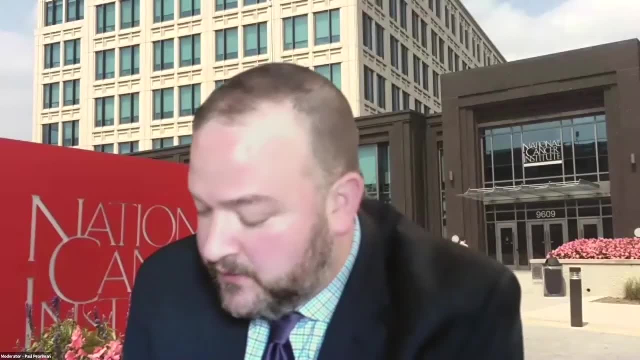 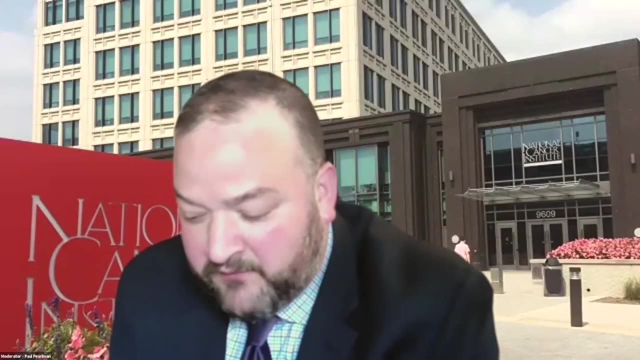 So we should be bringing all of our speakers up right now for the panel discussion. I'm going to go ahead and kick it off with maybe a couple questions that were hinted in the talks, So this one is initially for Professor Kuya, but I think was relevant to everyone. 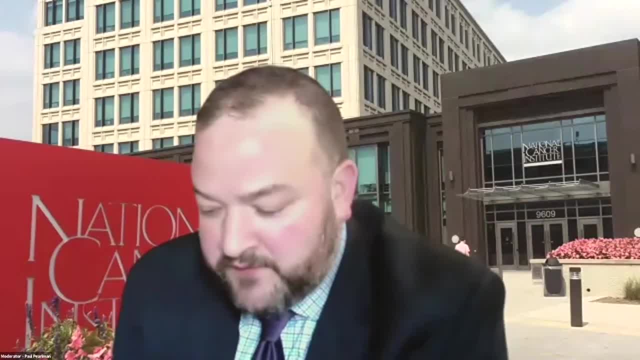 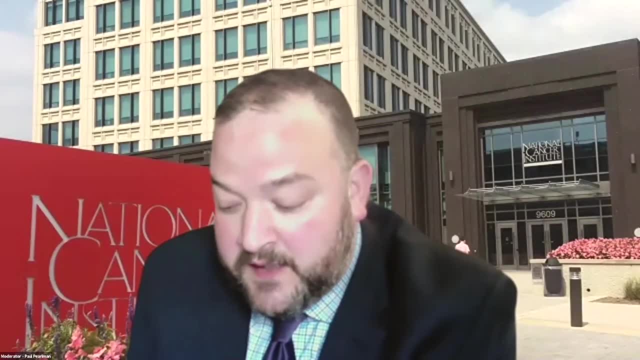 How should we think about applying machine learning and artificial intelligence when our data sets may be small or, as Professor Kuya suggested, some of our data sets may be small? How should we think about applying machine learning and artificial intelligence when our data sets have poor image quality? 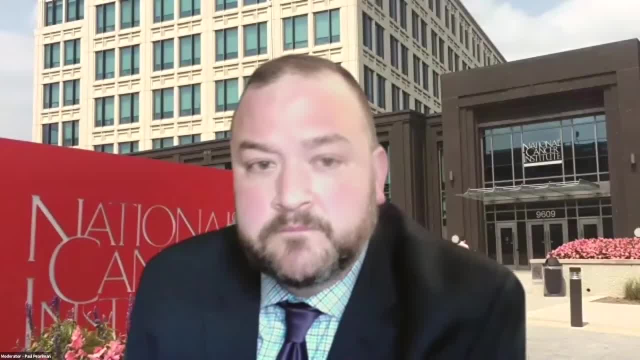 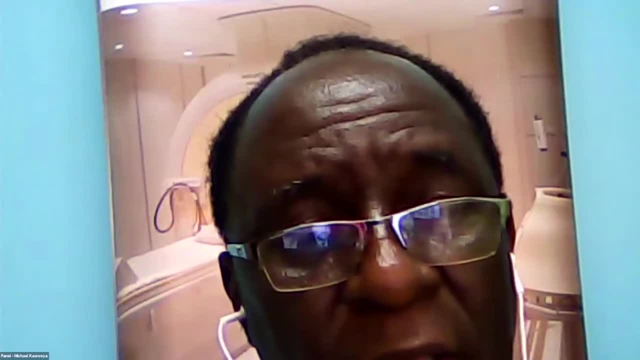 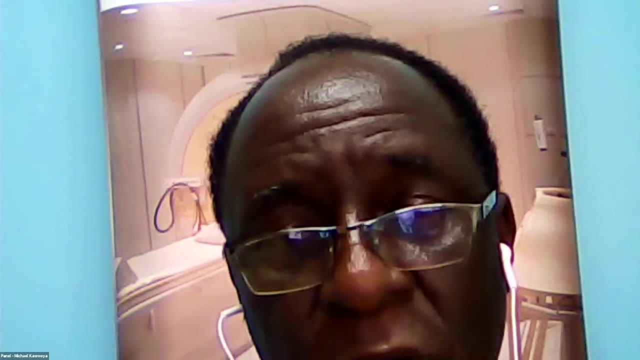 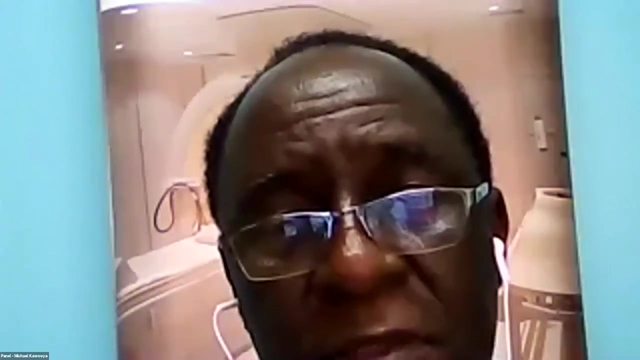 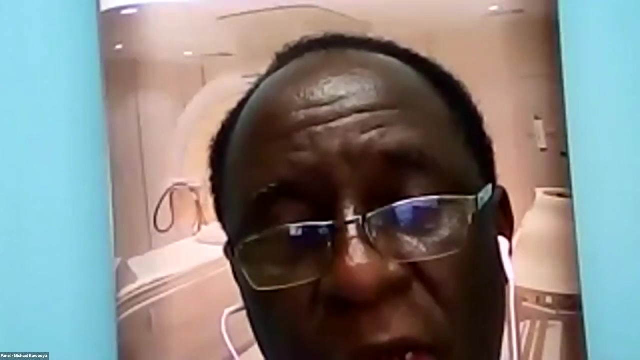 Thank you, Paul, for that. When our data sets are of poor image quality, it becomes difficult for us to apply machine learning, because it will be difficult to train the algorithm with images of poor quality. So I think it's very important that even as we begin, we must ensure that our quality is uniform and that the method we are using is also standard and homogenized. 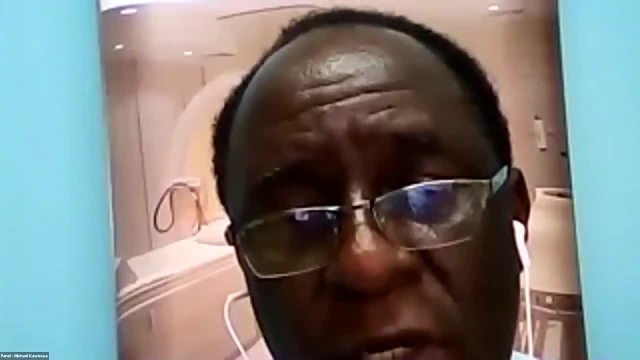 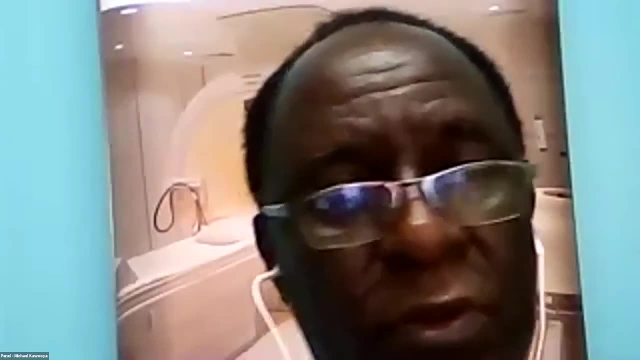 That's all that I can say, because I mean, the algorithm will just get confused with images of poor quality, And I can also comment, Paul, I think one of the things that is really important for our audience to understand is that we need to be able to apply machine learning. 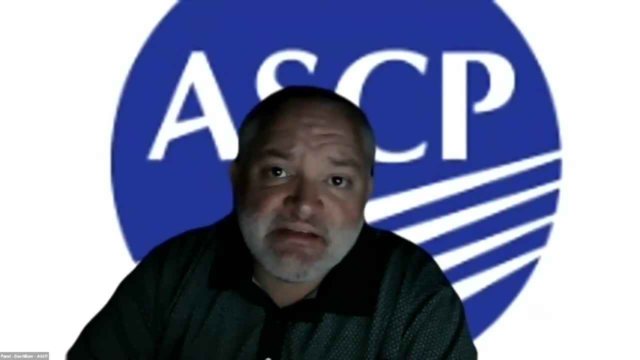 So myself. we trust that it's real, But if instantly it's useless, Countermeasures, areemy bind as a vorачить. So one thing that it's really important for our audience to understand is the state of the disease they might be wanting to work on. 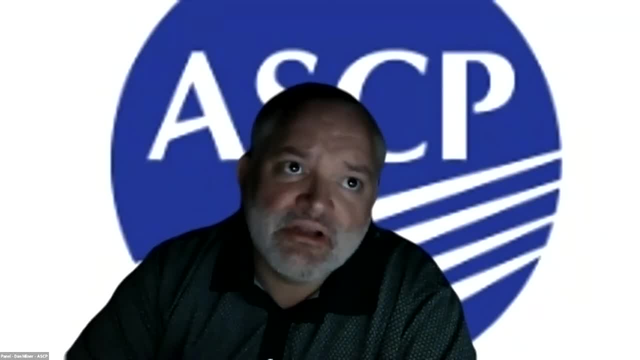 So if you want to do a project on the data science of tuberculosis or HIV or malaria or breast cancer, one country or even one center may have more than enough cases to produce a big data set, especially if you think about sequencing or other omics that are going to go with it. 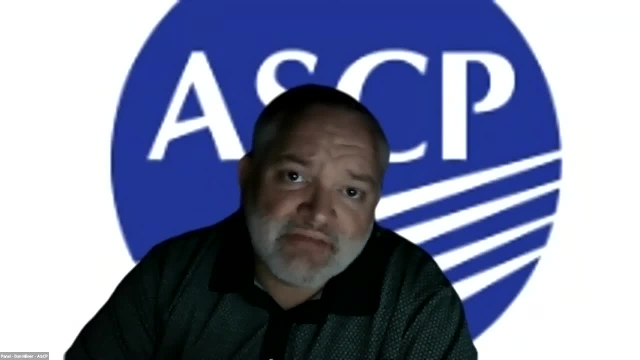 But when you start thinking about rare cancers, for example, or rare infections, leads online rare infections, multi-center or even multi-country data sets may be needed in order to have enough images of a given disease in order to actually do that work. And so I think, as you are embarking on 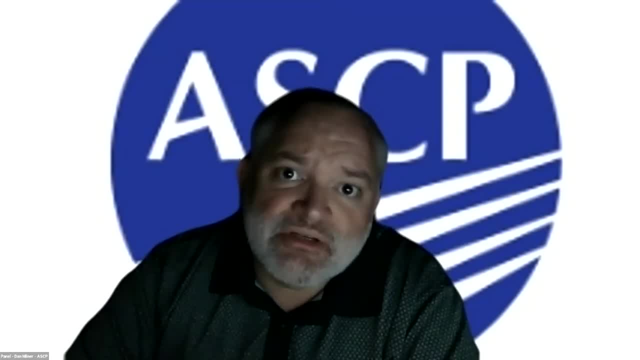 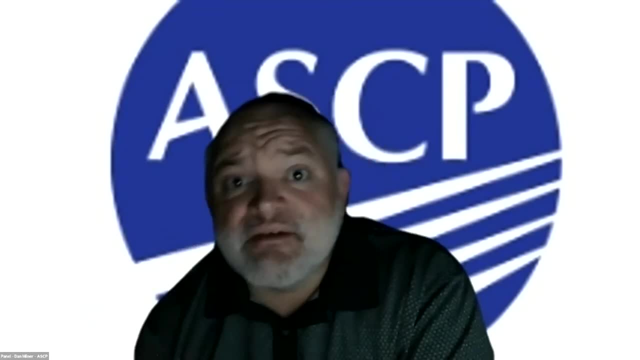 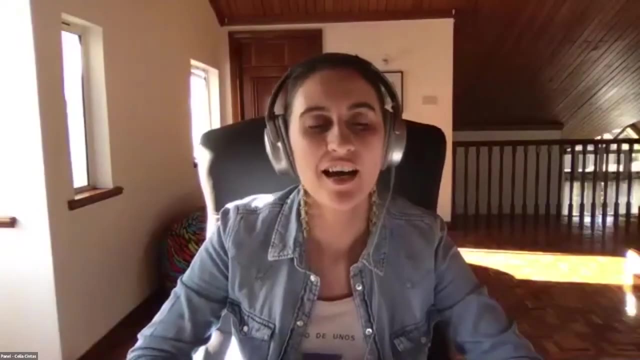 what you want to work on or what you're thinking about. consideration of the epidemiology of that disease is really crucial for sample size, as well as the amount of money that you have for these particular grants. Also, on the machine learning side, as you saw in this talk, we use 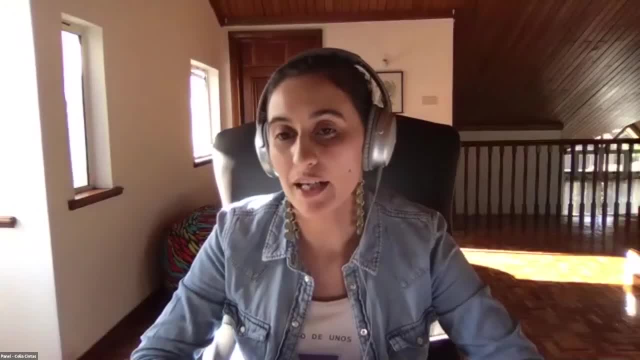 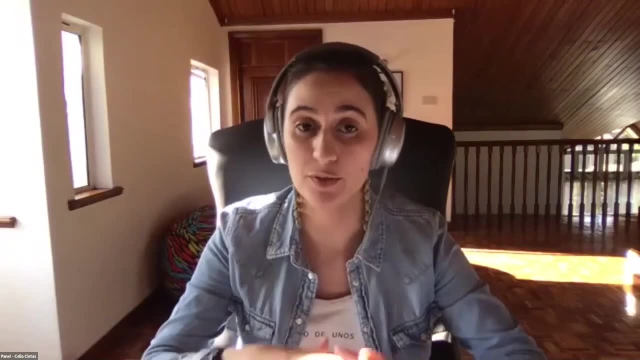 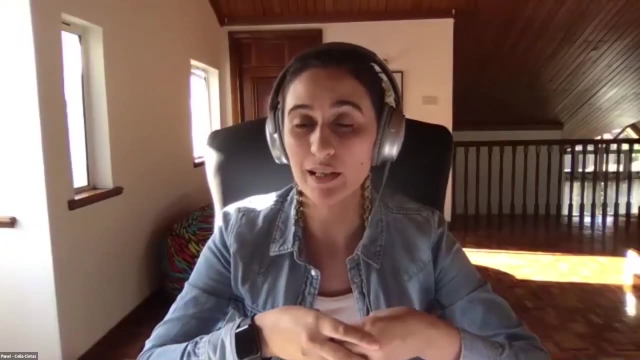 pre-trained models. If you are using image-based data, you can actually use training models to base on other data sets more large, and you fine-tune to your small data sets. So this is a technique that works very well on images, because usually these 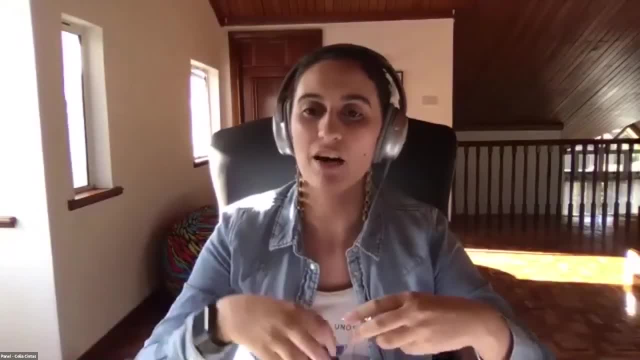 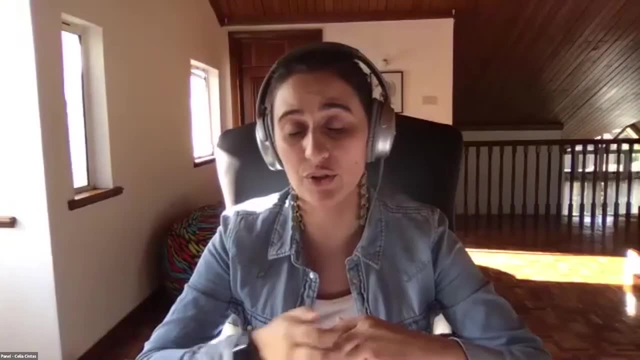 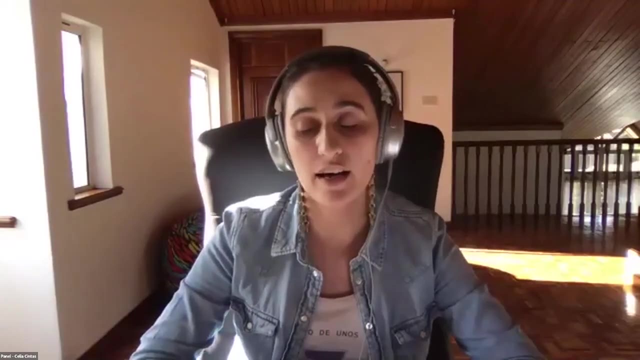 different neural networks work on the same idea of finding edges or finding features that are common across all images, So you can fine-tune your models when you work with the small data sets. Regarding quality-wise, if you have a matched set of low quality and high quality samples. 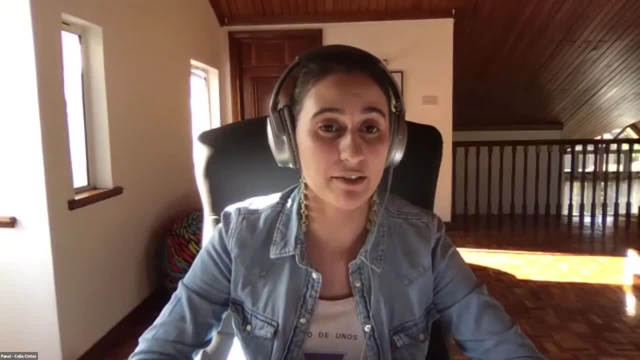 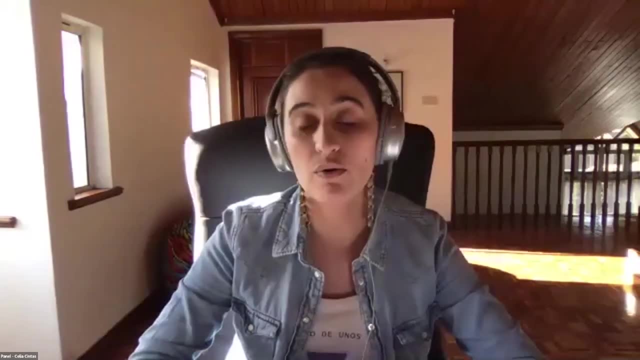 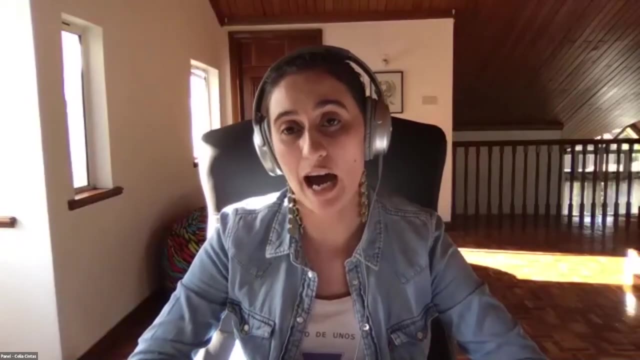 this will be an ideal setting. You can actually train generative models to learn what a high quality image representation looks like. So any low image data set quality can actually be transformed to high. but for this you at least need to have the pair of good and high quality. 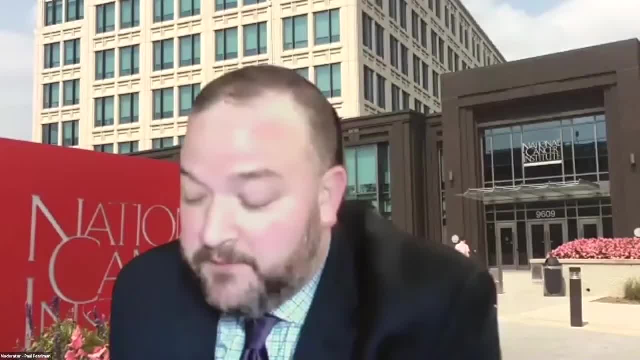 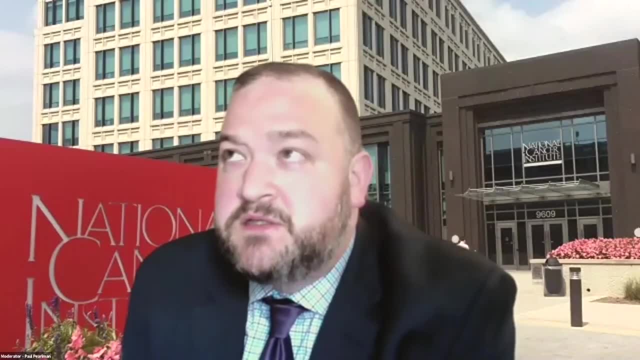 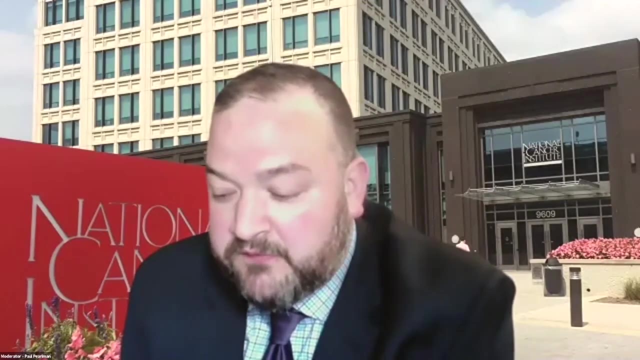 Thank you. Potentially, another one that we get in most technology-related panels is, you know, as we started to talk about the need to develop sort of new cloud infrastructure and as people start to think about these grants is: are there what opportunities exist for sort of leapfrogging over? 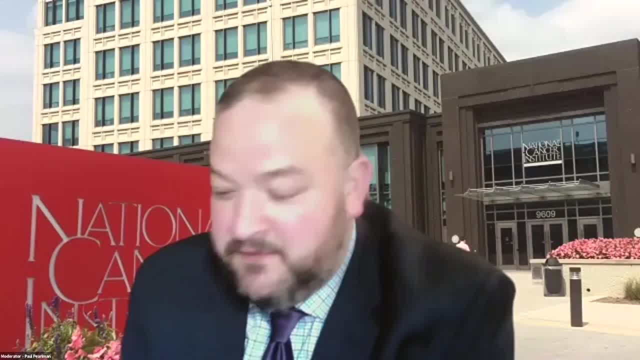 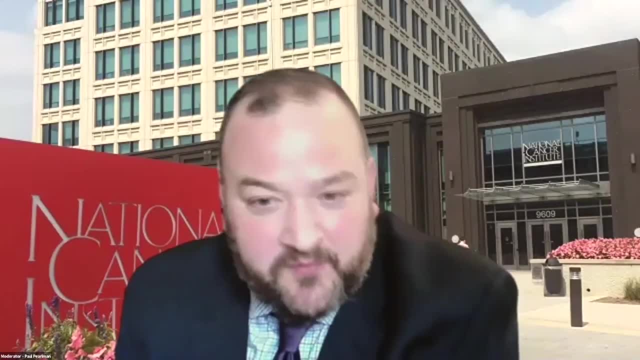 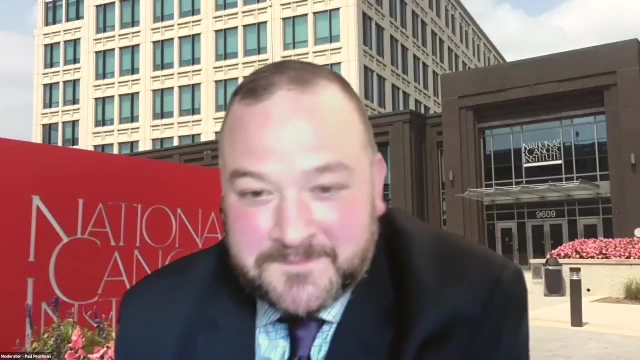 some of the fits and starts we've seen in sort of developing standards and other issues in terms of generating large data sets. Are there opportunities to learn from our from past mistakes elsewhere? I'll key off on the word generating data sets there. Okay, 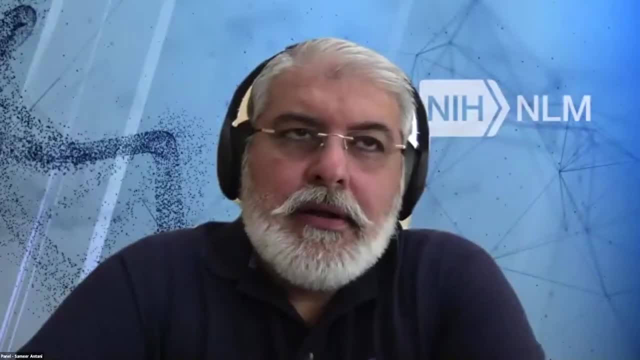 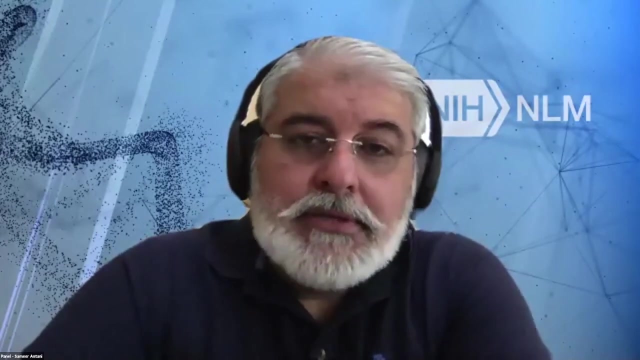 is that if you are embarking on a new study and you have the opportunity to acquire new data, then establishing protocol- I mean, I'm speaking not, as Dan alluded to, scanning Mr Pathology's slides, which is there are many standards in place. 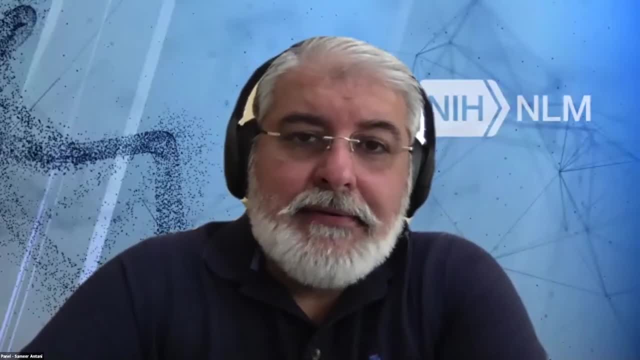 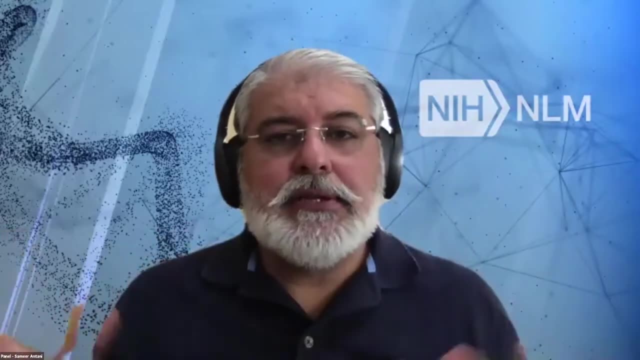 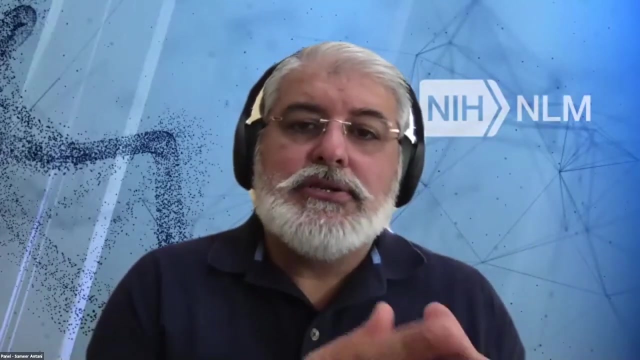 and selecting the appropriate scanner and scanning technology may address some of these challenges. But if you're thinking of acquiring pictures, or you're thinking of sampling the population and considering the epidemiology aspects and then considering the clinical protocols that are in place so that you don't have the variety, 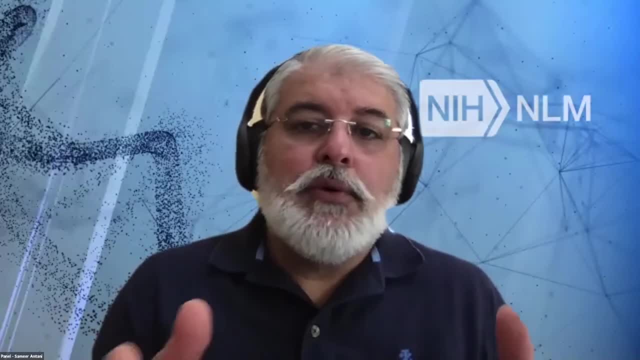 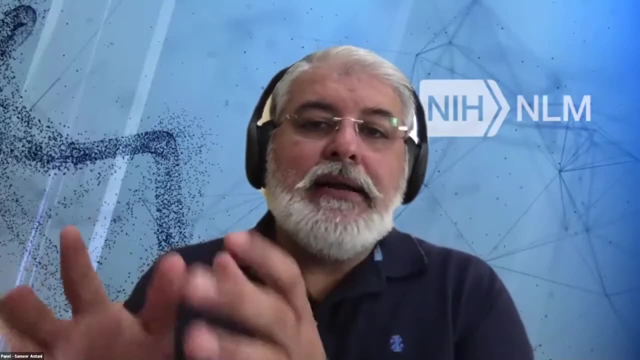 that would disturb your training. At the same time, you don't want to make it so artificial that when you revert back to a natural setting you have a highly skewed and perfect in air quotes data set. that is not a representation of reality. 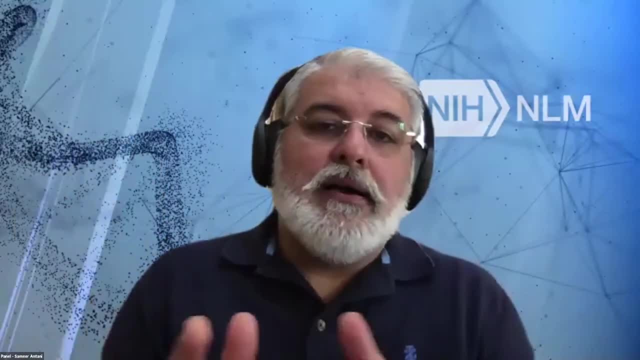 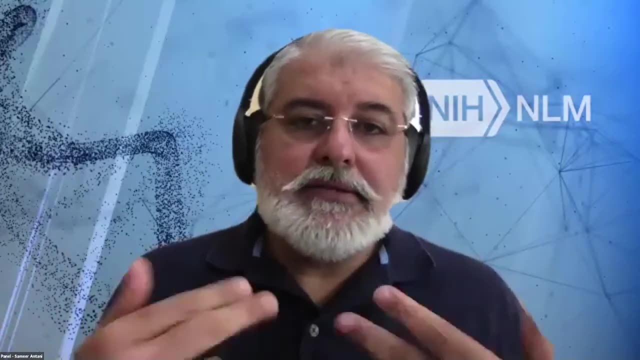 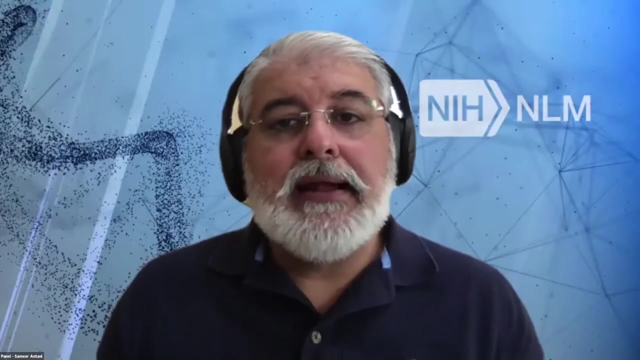 So striking a balance between the two. yet if you are pushing the technology forward so that you have a good quality set giving consideration to this. And one thing we notice is different imaging devices tend to have different imaging characteristics, and lighting conditions will influence how the picture appears. 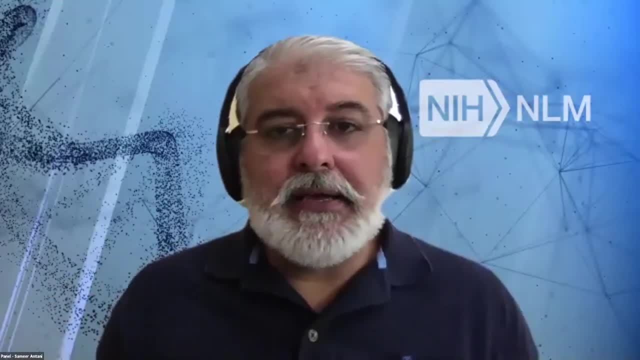 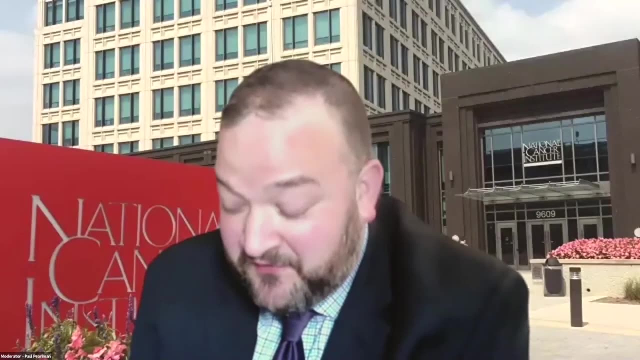 And human eyes are amazing at adapting at all the variety, but computers are still a ways away from it. I think, initially, this one's going to be for you, Sameer, as well. I want to re-ask one of the questions that was answered in the chat. 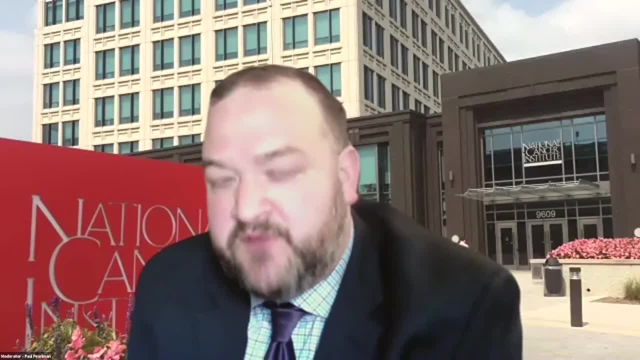 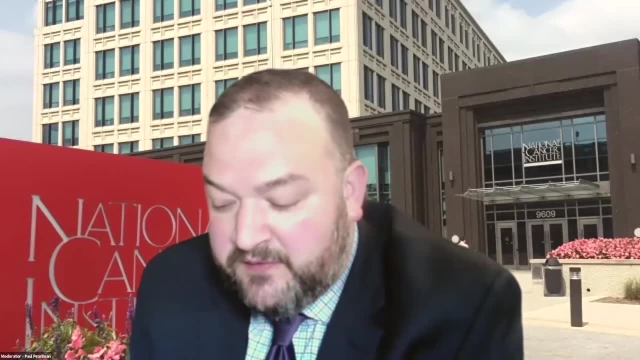 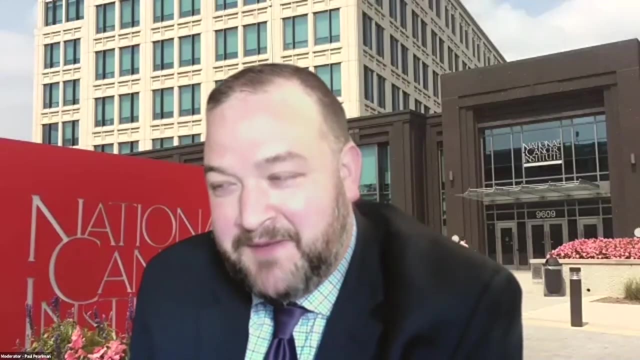 And that's what are the major limitations of deep learning you described. And I'll add to that: when we think about deep learning, how do we think about some of the issues associated with the fact that we don't always understand why our algorithm is making a certain decision? 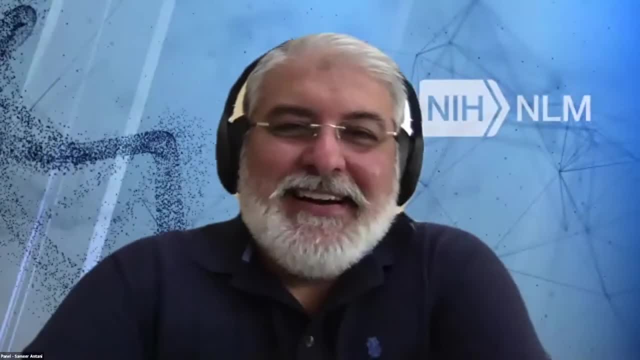 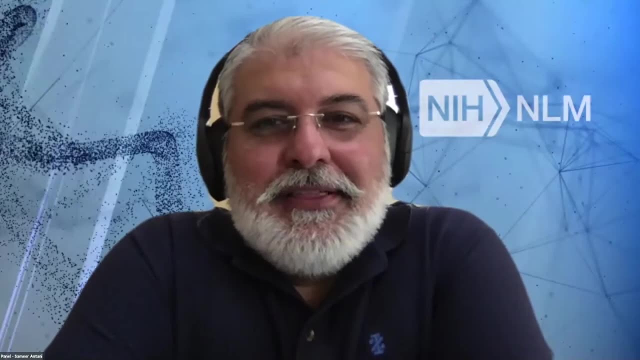 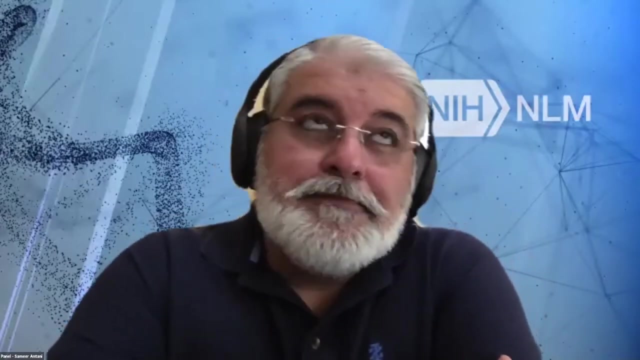 That is to say the question: How do we think about some of the issues associated with deep learning? Right, that is almost entering the space of deep learning art than science In the sense. there is science there. You have to visualize what the network is looking at. 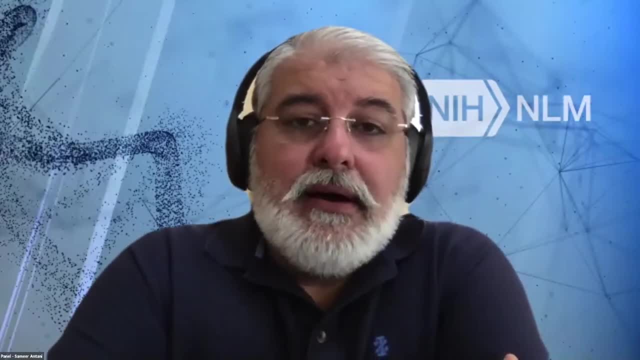 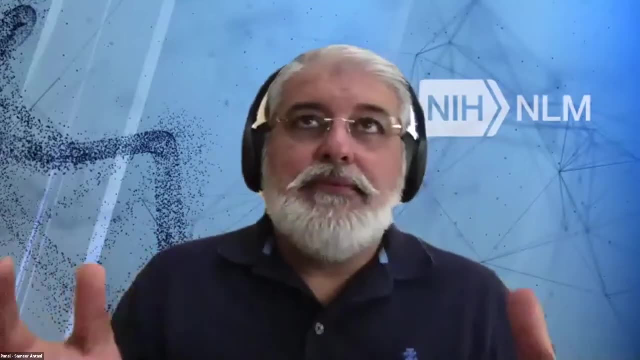 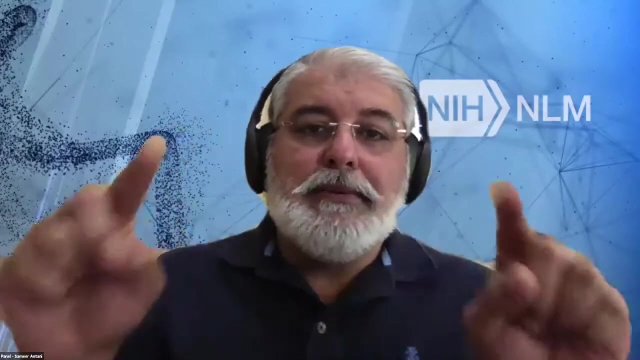 and what it's focusing on. Now you can artificially influence the network to look at certain regions using other deep learning networks. So every We think of deep learning networks as decision makers, We can cast segmentation, which is drawing a boundary around an object of interest. 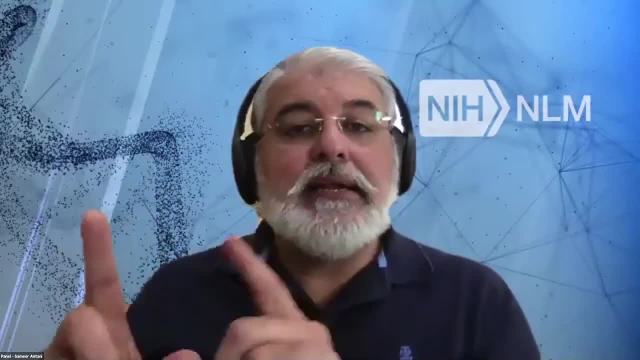 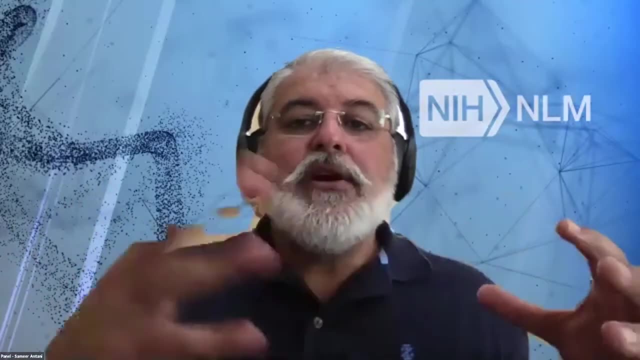 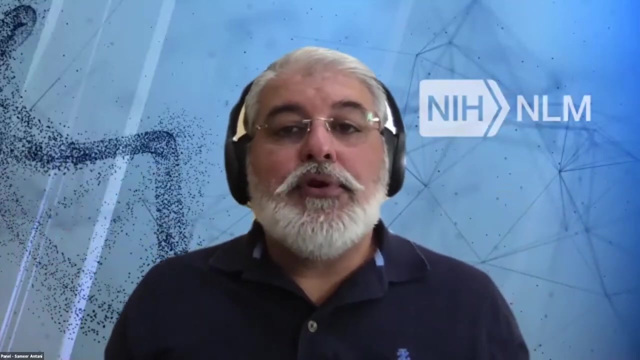 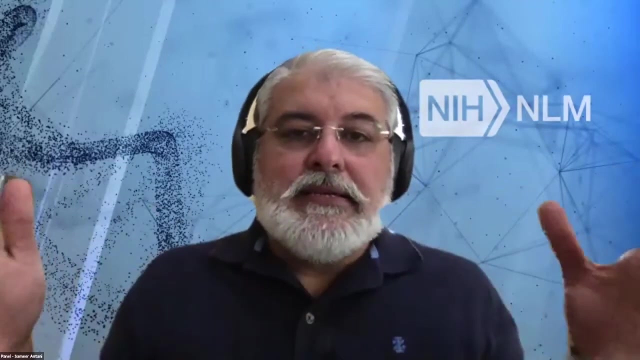 or recognizing an object in an image as classification tasks. They also are selection tasks. So, having a chain of deep learning networks, one can influence them And therefore you are sort of handcrafting a little bit, helping it along and, in a sense, building an end-to-end system. 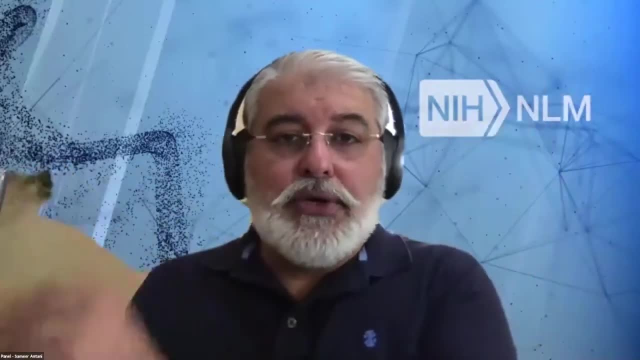 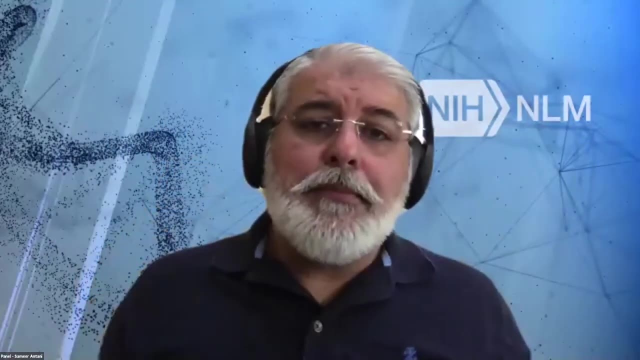 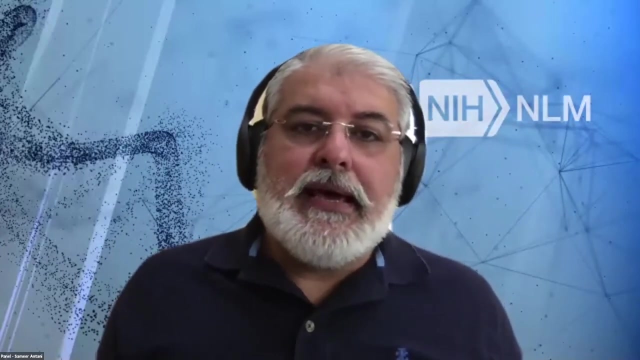 that, given an image, it would percolate through your various networks, resulting in an answer. But if you think of each individual network, one can put in probes to see if it is being disturbed or distracted from looking at the object of interest and not what you want to look at. 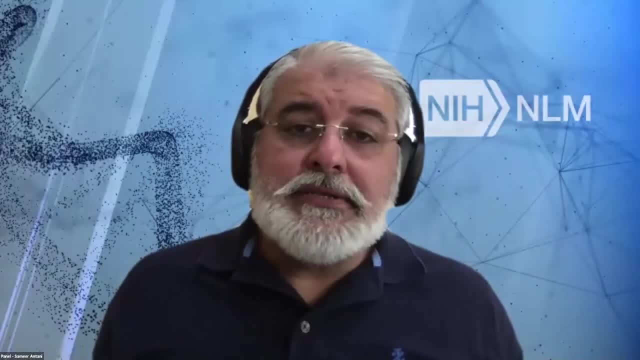 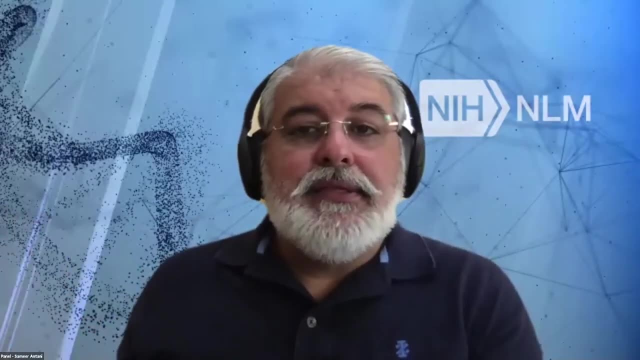 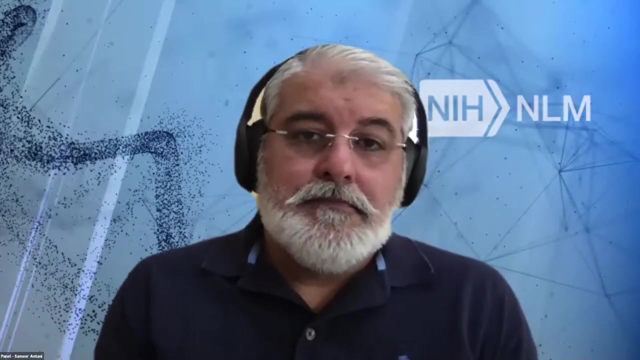 The only caveat I'd put is: if your goal is to look at the object of interest, if your goal is discovery- that means you have an existing collection and you want to find outlier patterns- then this strategy might be the best strategy. So we have. 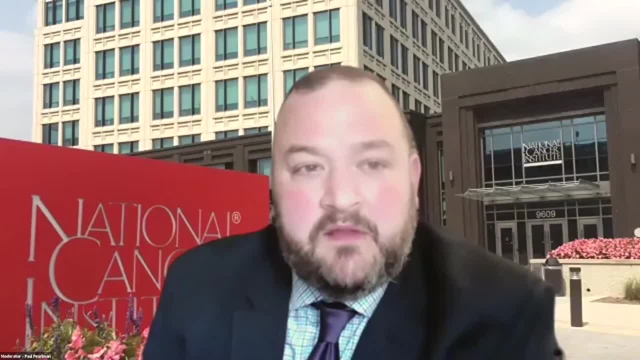 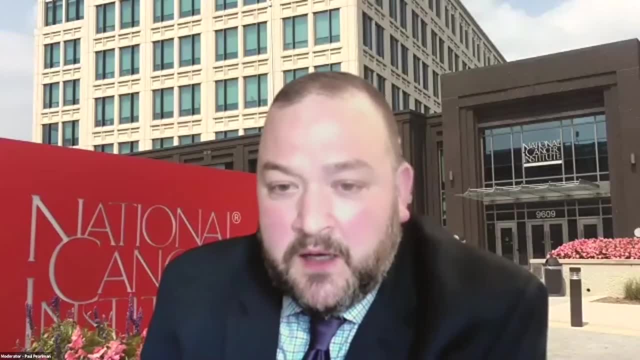 A couple of questions have come in looking at the intersection of multi-omics data and imaging and understanding sort of the value added through adding multi-omics data. I think this is a good time to start. I think this is a good time to start. 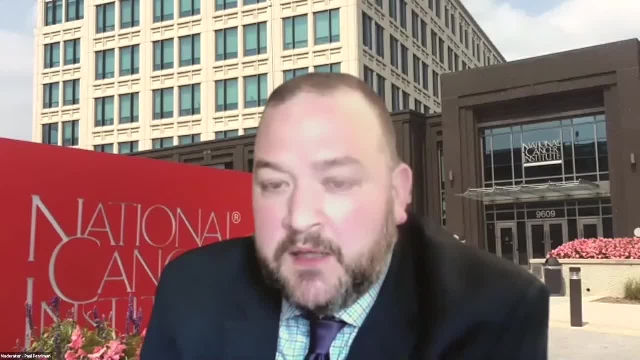 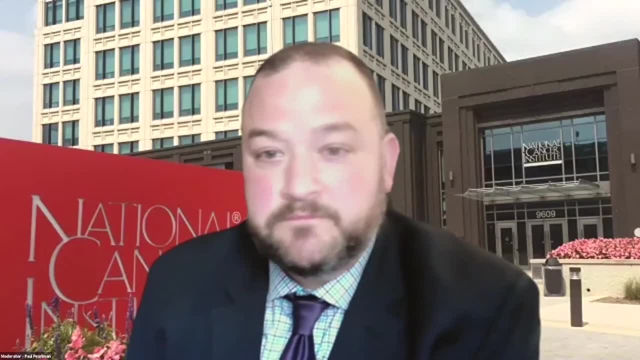 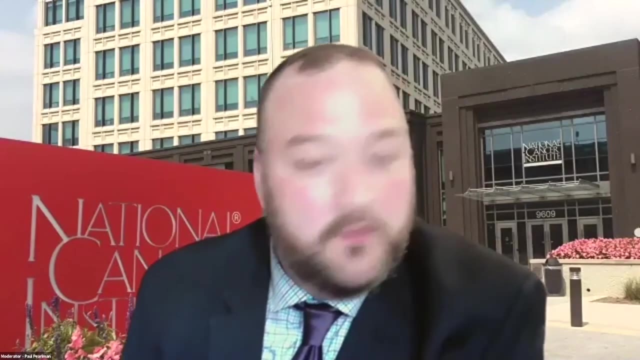 I think this is a good time to start. I think this question could really go to almost any of the speakers- Anyone, So okay. So potentially Could you repeat the question? I'm trying to look at it in the Oh yes. 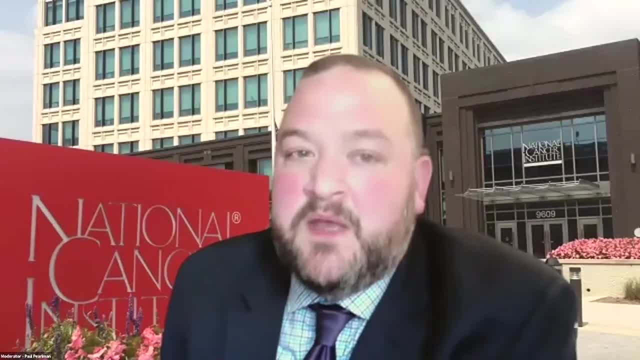 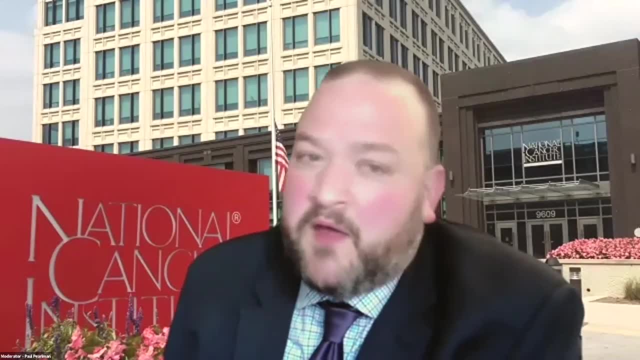 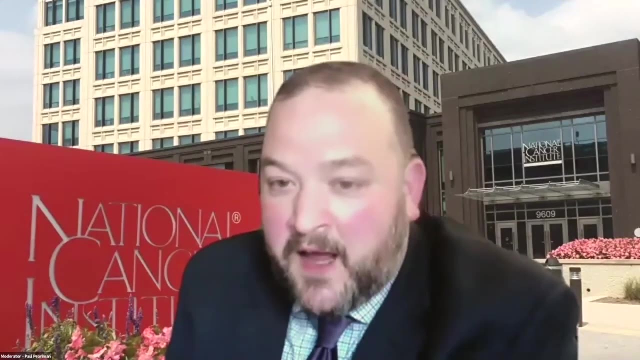 So the question is what sort of multi-omics data has been used in the context of imaging and what is its sort of value added? And then sort of what other omics data would be a priority or valuable to increase the prognostic value of sort of a machine learning or AI tool. 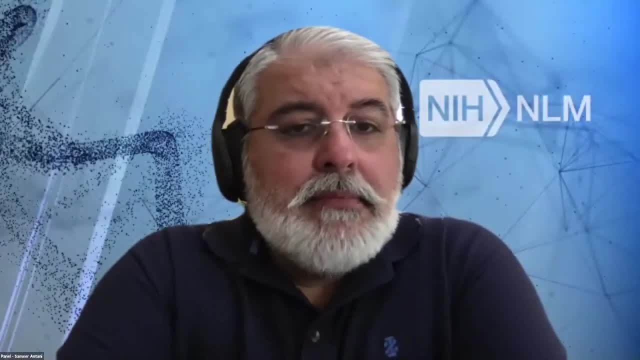 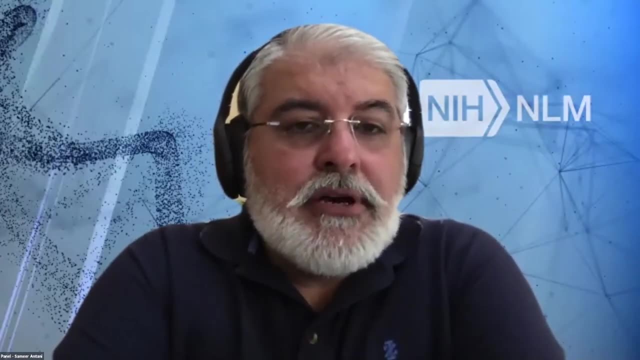 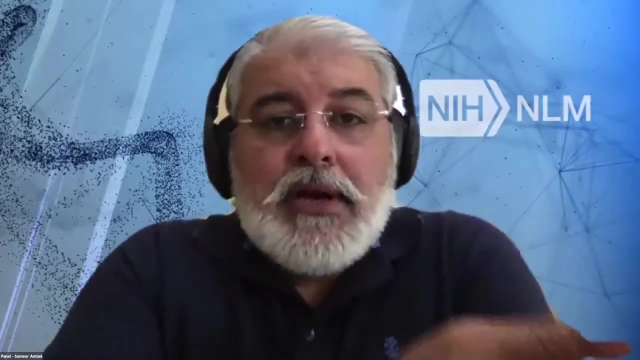 So let me start off and maybe I'll prod Dan a little, if you can jump in, But I think he was alluding to this toward the end of his talk where, for us at least, omics data, as in terms of coming from radiomics and genomics or proteomics. 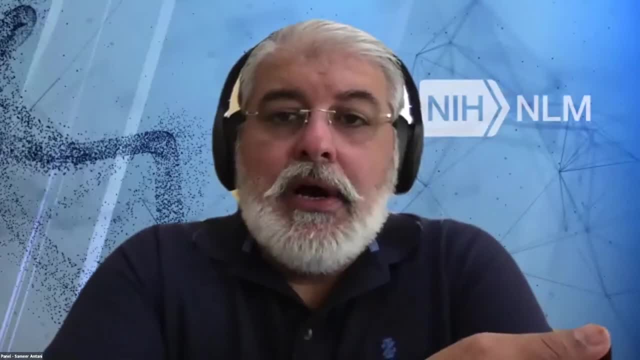 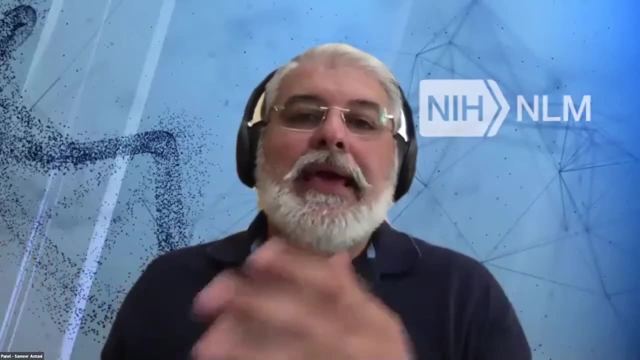 probes and so forth, But I think it's really important for us to provide a sense of truth, absolute truth that helps us train an image. So, looking at an image alone, you want the AI to step in and provide a high standard. 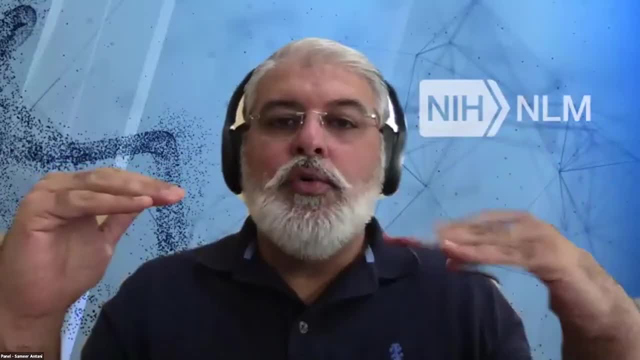 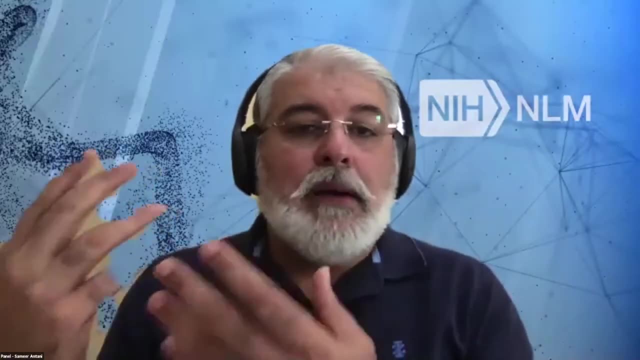 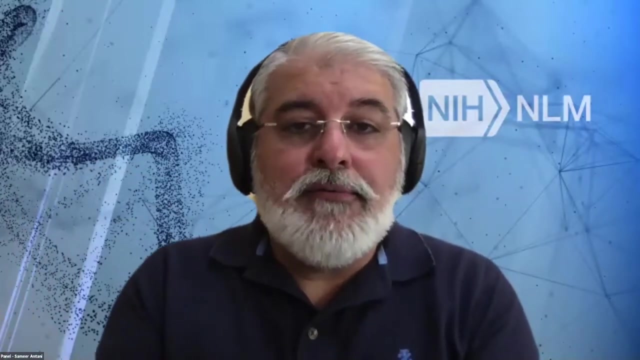 of truth at a very low cost point, entry point. So, if you think of the cervical cancer problem, where I would like to use a common handheld mobile phone, let's say, To be able to determine if a woman is in a precancerous, or a stage at least where she 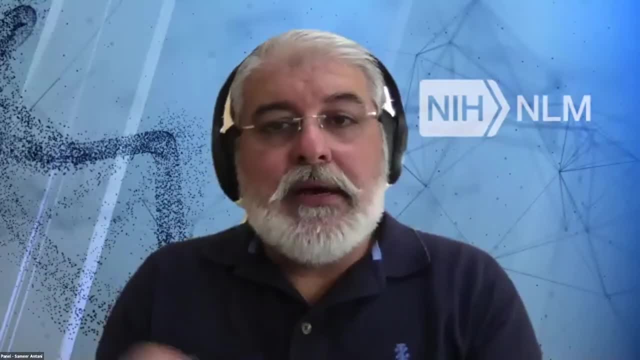 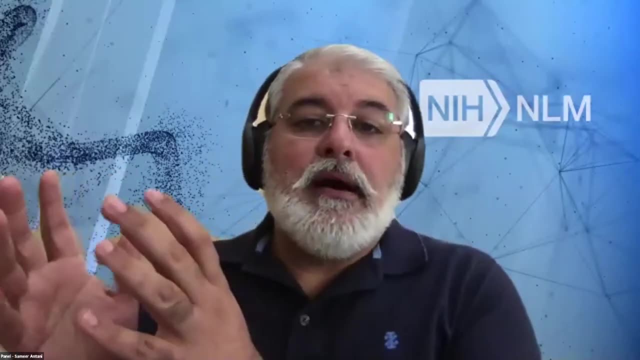 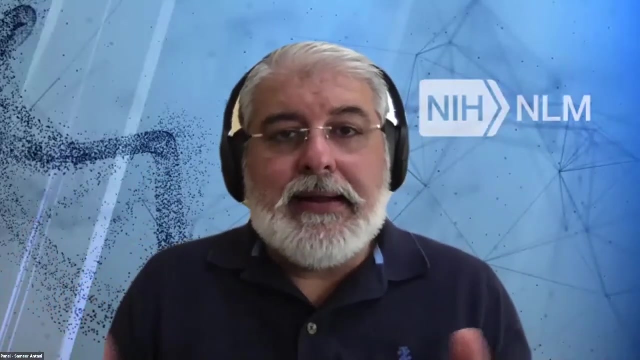 needs more repeated, frequent visits so that the disease is progressing. Now, the only way that we learned that was true in…. Now we know that the images themselves don't provide this truth. Humans are gloriously bad at looking and classifying this, and if you throw the same sort of images, 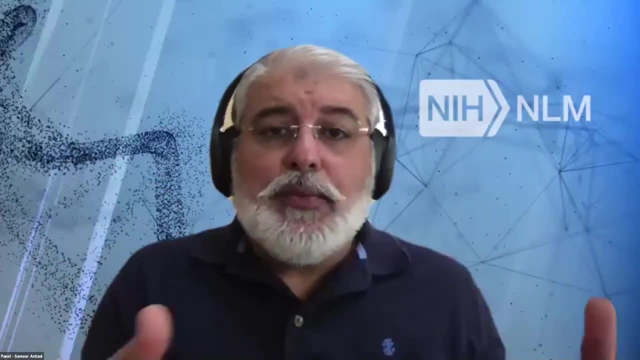 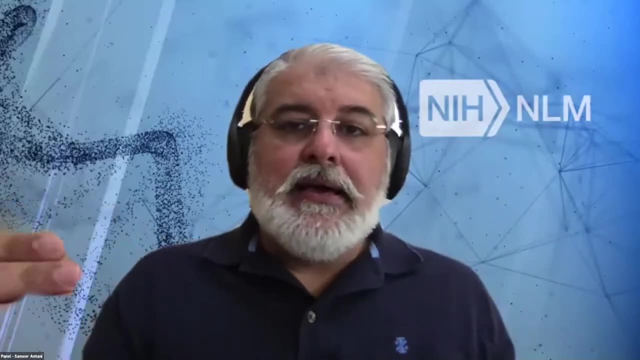 with the same human… Dead human- truth standard added in AI, it will arrive at the same level, or slightly better perhaps, than human performance. But if you want to advance the AI, then the idea of introducing other omics data as truth standards. 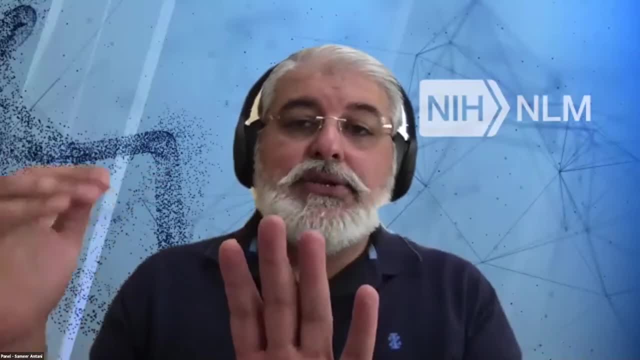 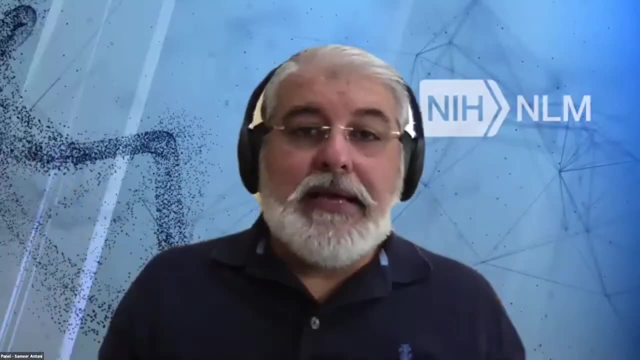 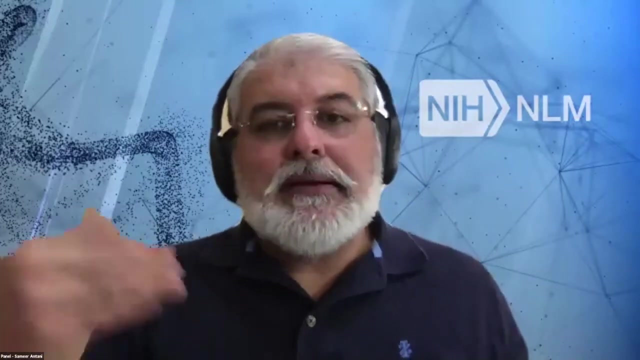 So we are not showing the truth standard to the machine. They're saying that this image truly is positive. And now figure something out, see something more in the pixel patterns that we are sort of abstracting away from so that we can help it. 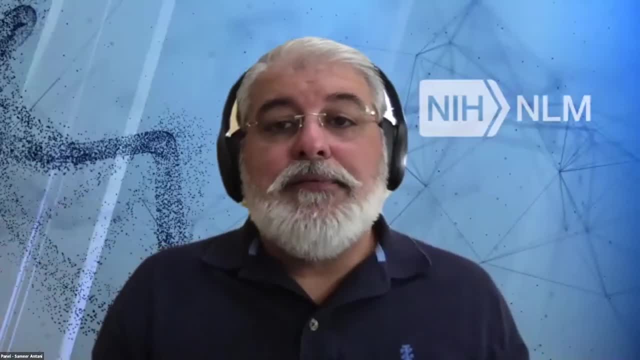 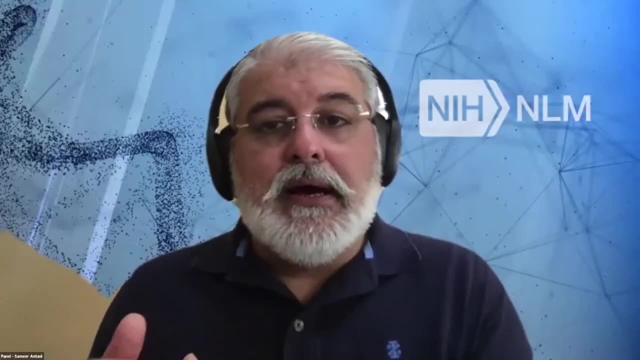 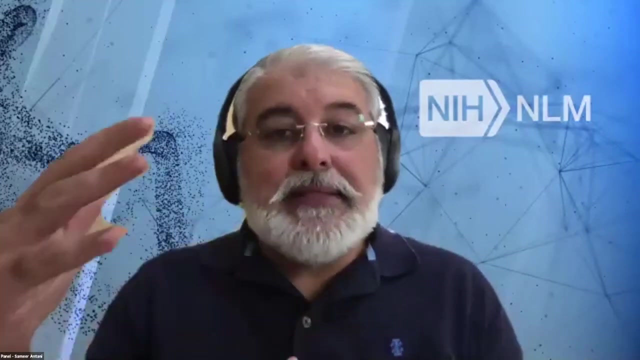 So that's one way- is providing absolute truth standard. If you're going to now expand this further and include other health record data along with other omics data, then you are expanding the kinds of inputs to a much more glorified deep learning network set. 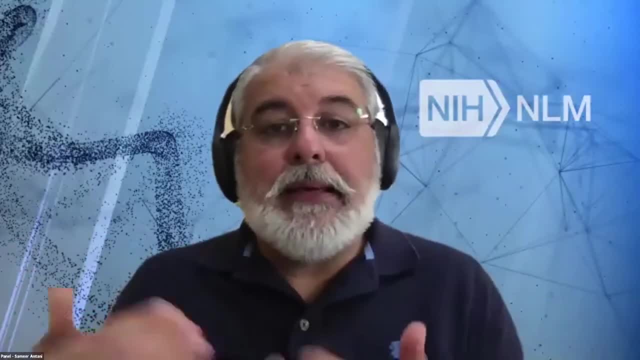 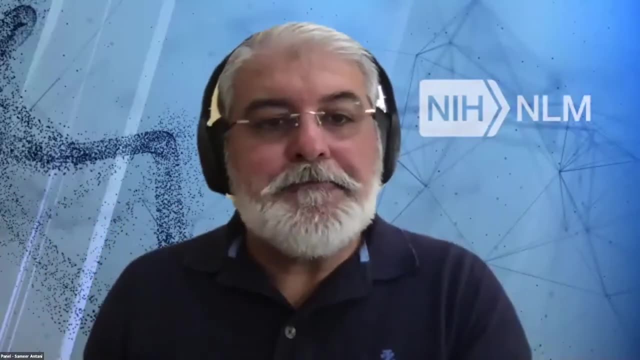 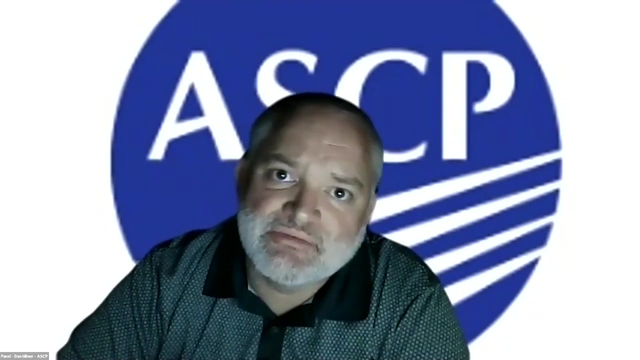 so that it can take in multiple input sources and provide a better level of decision. the other end, That's one slant out, Yeah, and I would just add that pathology images, for example diagnoses of cancer or subtypes of cancer. 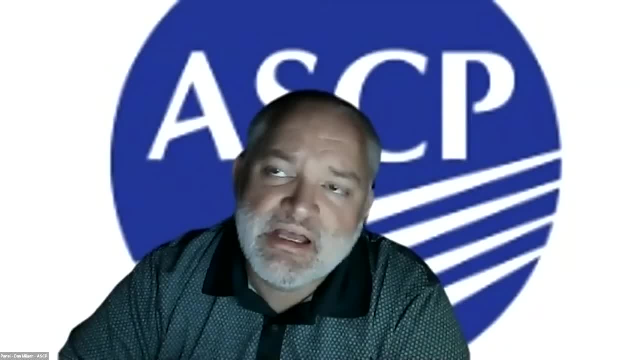 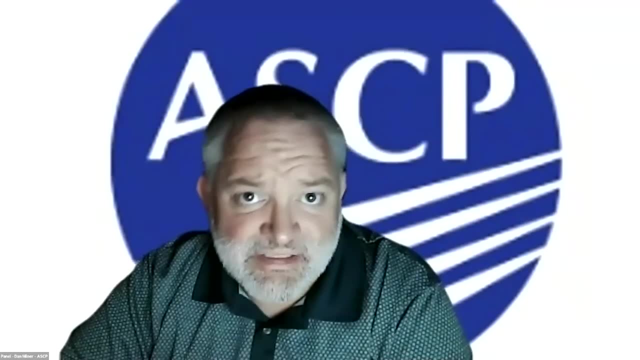 mitotic counts, classification of tumors to a very high level degree, are often used as the ground truth or the gold standard by which to then look at omics data sets or genetic data sets, et cetera. And I think you know. 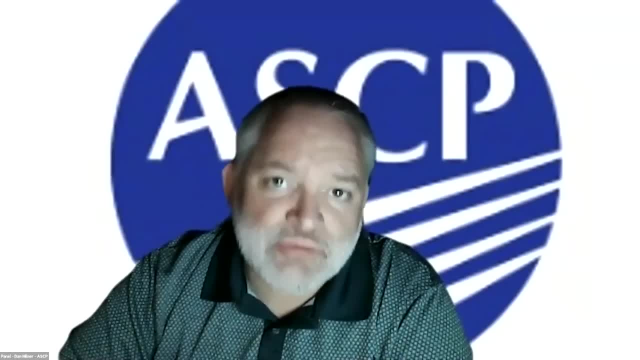 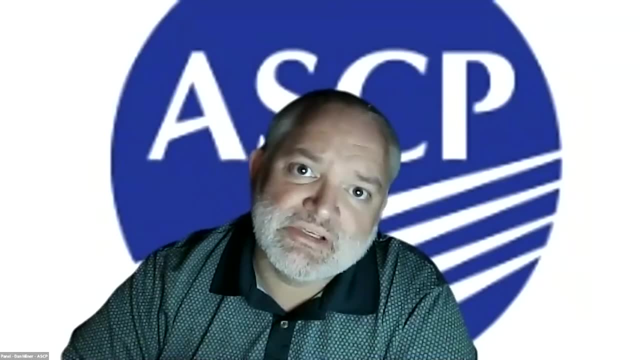 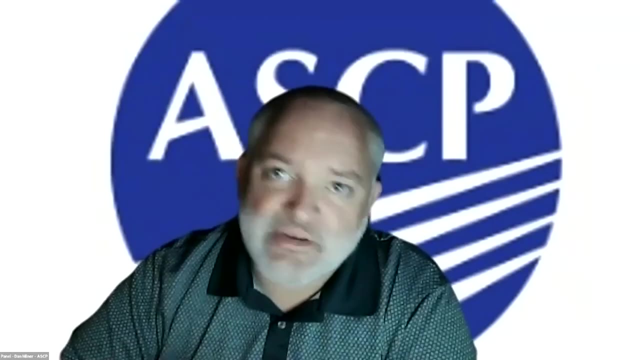 early studies, for example of transcriptional profiling of tumors, demonstrated that the transcriptional profiles matched up pretty closely to the histology. But then, when those data sets grew and became very large, it was clear that within so, for example, adenocarcinoma of the lung. 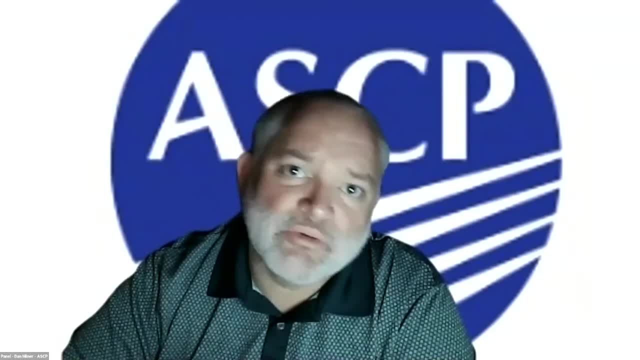 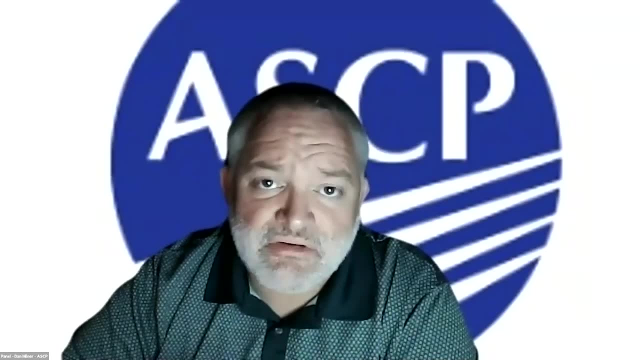 there were subsets of transcription profiles, and that's where new therapies, new diagnostics have actually come from, And so I think you, you know, you always start with a gold standard, and histology is obviously an excellent one if you have high quality, as I was describing. 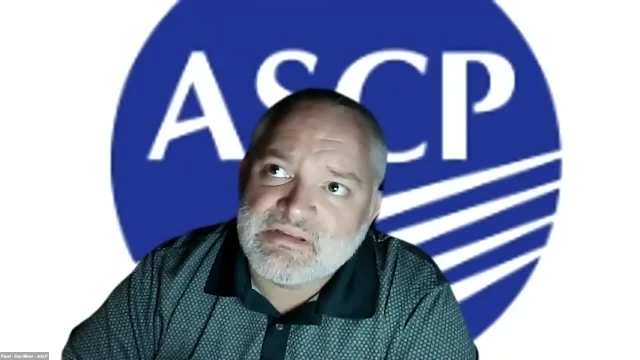 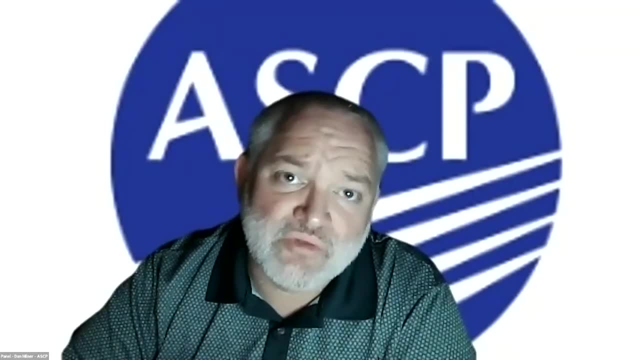 but the goal is for the AI, or the research that you're doing on the image analysis, to supersede that and to tell you something new beyond just what that gold standard told you. And I think, as you add more omics data sets to a given grounded data set in pathology, 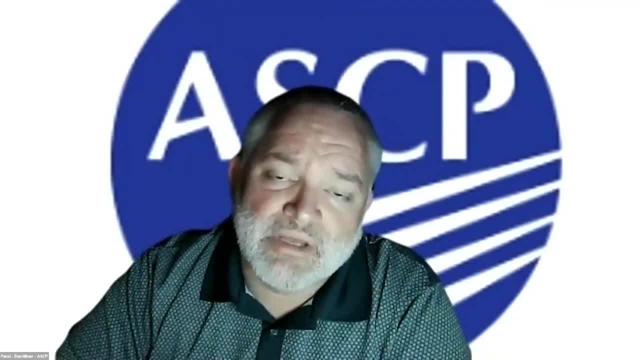 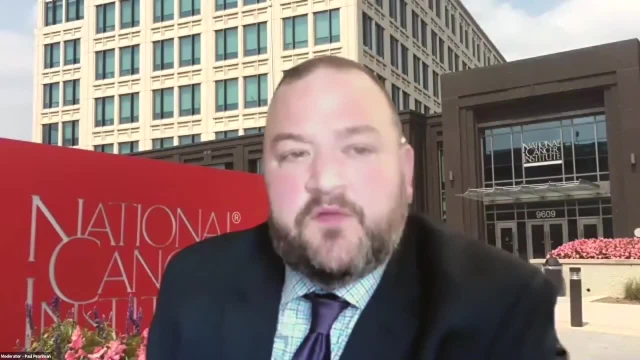 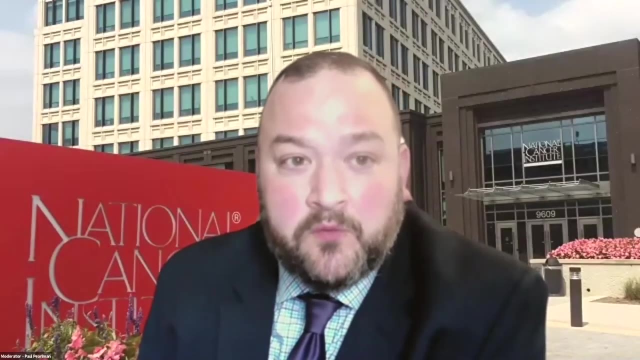 you learn more and more about those images and ultimately come up with better diagnostics. Thanks, I think. this one is for Celia, And so this is a question around sort of how you approach achieving an equitable AI tool, That is to say, and the question goes further to ask- 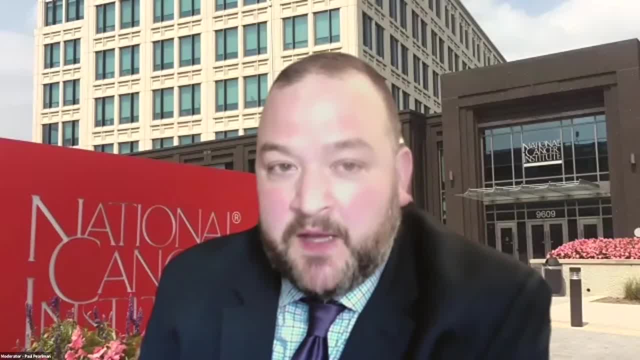 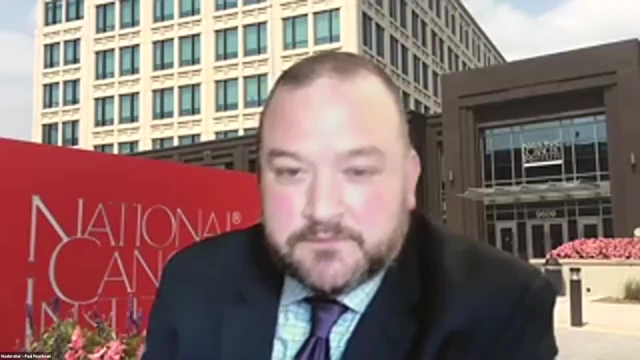 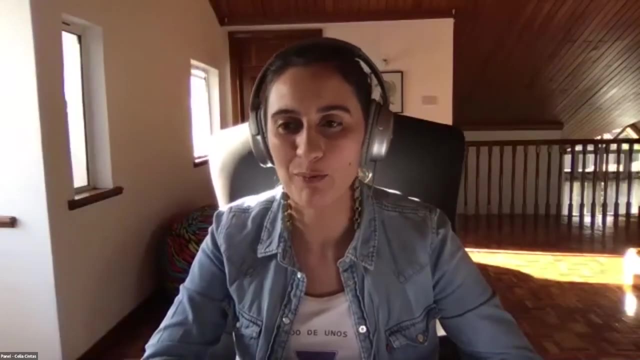 whether you use a multi-model, sort of per country or per population approach, or a single model attempting to be more general. That's a good question. What we learn, at least for our specific problems, is always by population base. You will not have a one single model. 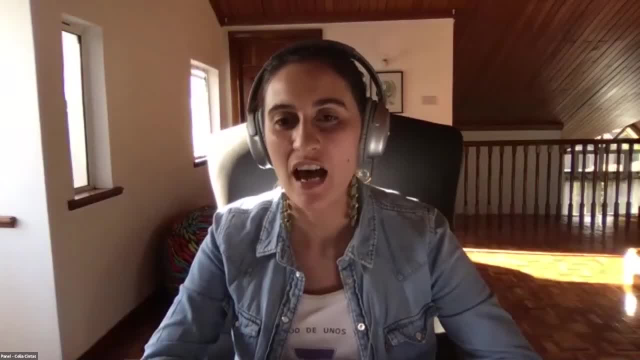 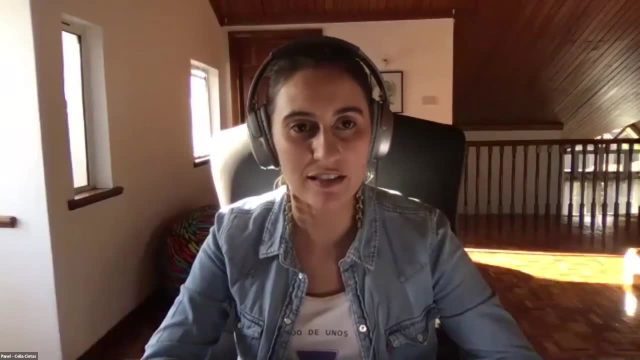 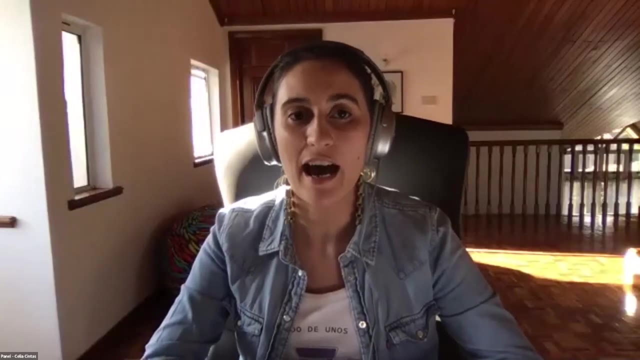 that will tackle all different populations. Regarding fairness and equitable machine learning, I think the first step is be transparent about how the model was trained. what is the population that was working on? As when other researchers in other cultures or other side of the world are adopting, 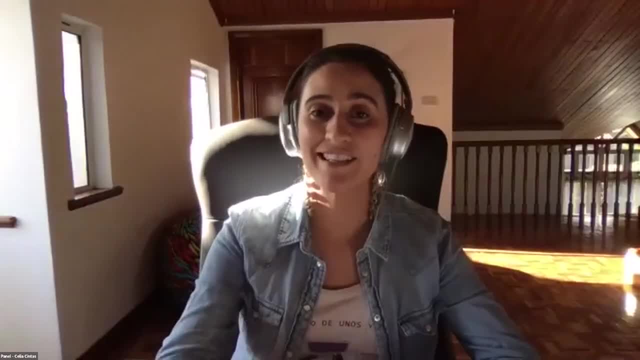 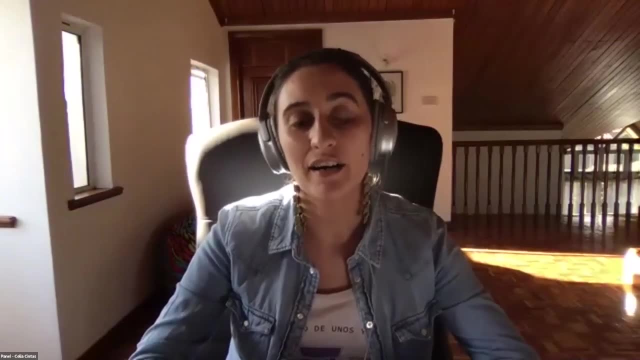 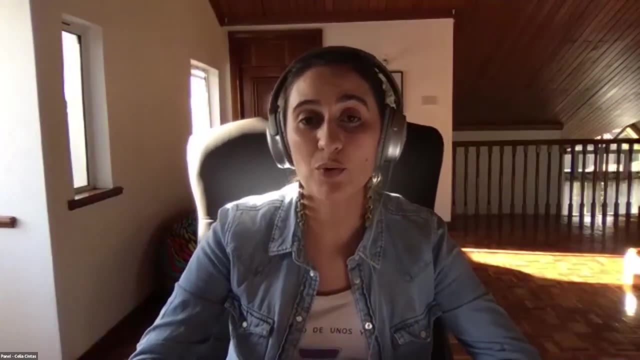 these already trained model, they can know to what extent this model will work for my problem. So the first thing it will be to be transparent, And then one very interesting comment is: how can we introspect these models? One of our panelists showed the ground cam visualizations. 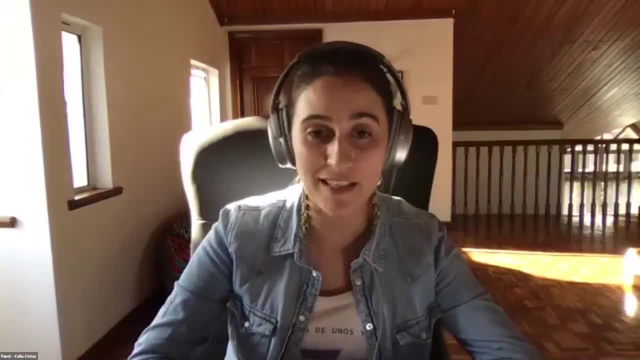 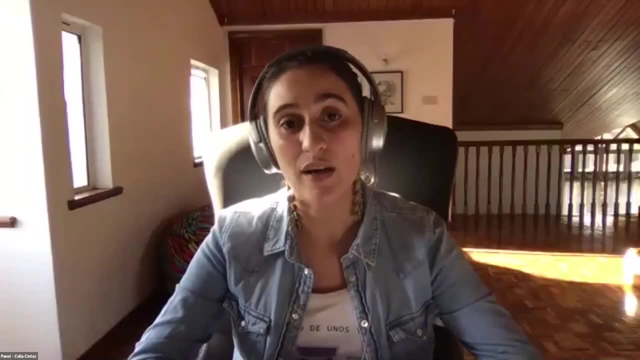 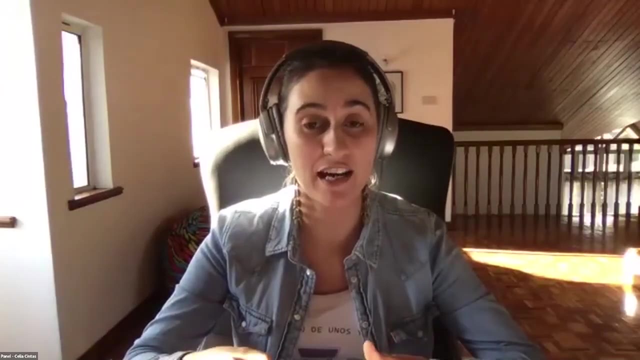 These are things that help you understand how the models makes the decision So you can have a notion on why that decision was made. So I think introspection of the model and be transparent on the limits, on how it was trained and the performance is done is super important. 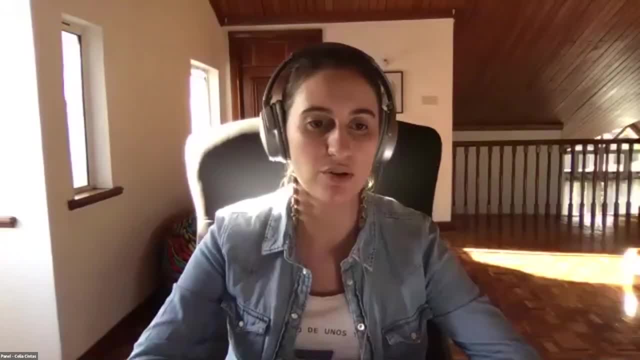 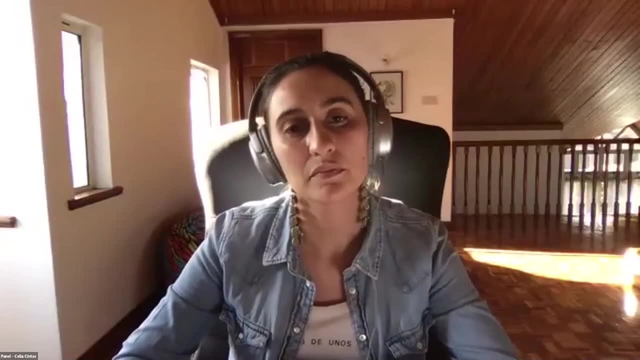 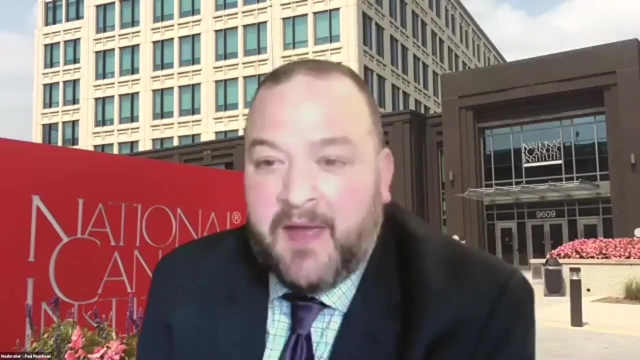 to build better machine learning solutions And thank you. And our next question is for Michael, And the question asks: sort of how big of a data, sort of a collection of data, do you need to start thinking about image analysis And AI diagnoses in the context of ultrasound? 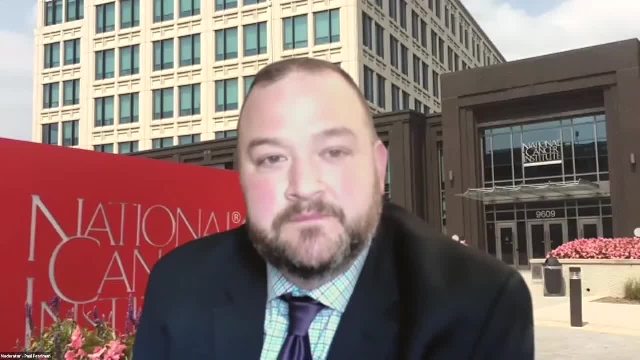 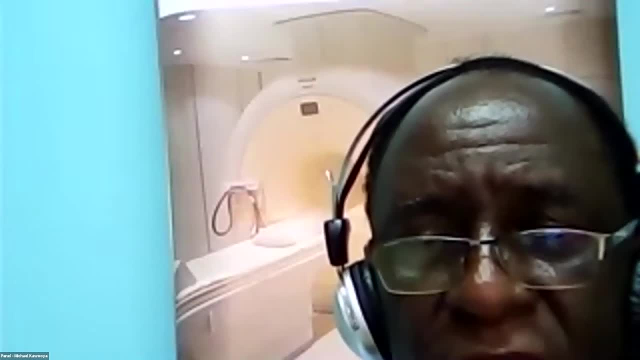 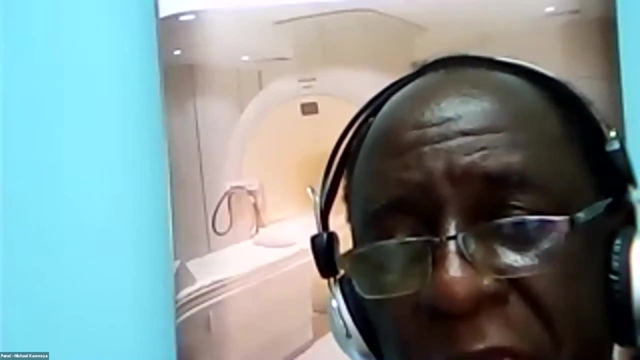 Ultrasound can be very tricky And depending on, for instance, if it's something like a gallbladder stone, where it's a yes or no, then you may not need so many images to train that. But if you're looking at something a little more complicated, 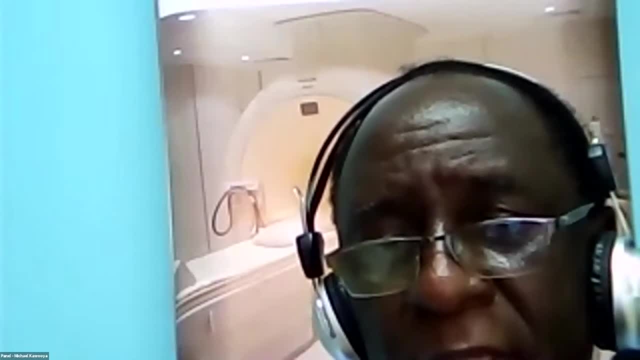 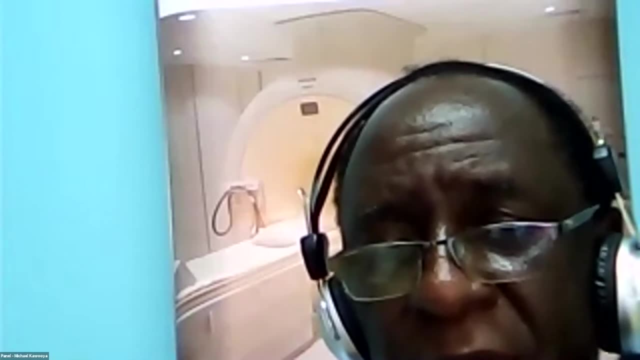 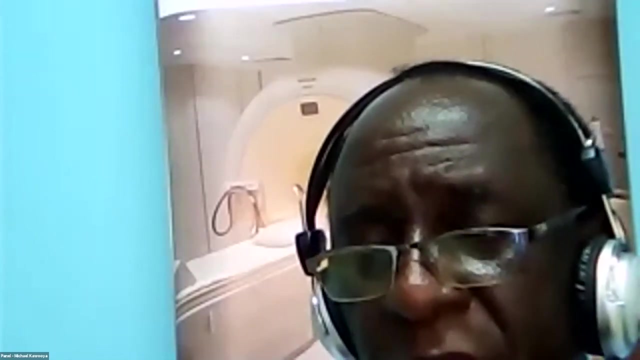 for instance, if you're looking at a breast cancer where there are different varieties depending on the virus, then you would certainly need several hundreds of pictures to do that, So it will depend on whether it's a black and white like gallbladder stones. are they there? 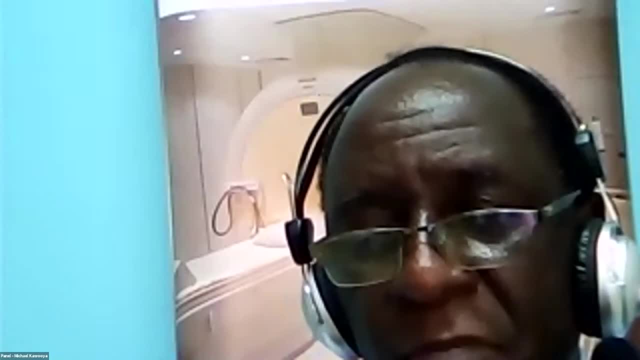 or they're not there, or whether, if you're measuring, for instance, bipyretic diameters, in effect, if you're measuring, for example, if you're measuring, for instance, bipyretic diameters, in effect, if you're measuring, for instance, bipyretic diameters, 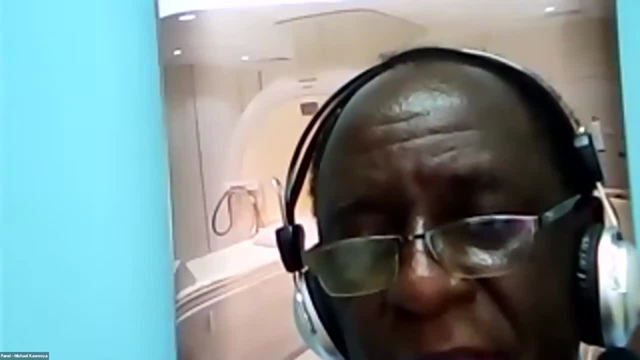 in effect, if you're measuring, for instance, if you're measuring, for instance, if you're measuring, for instance, like the fetus in the femur, in a fetus, that's a little more straight forward But where there is a little more heterogeneity. 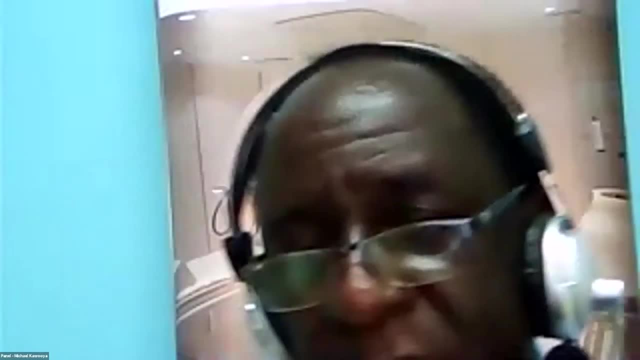 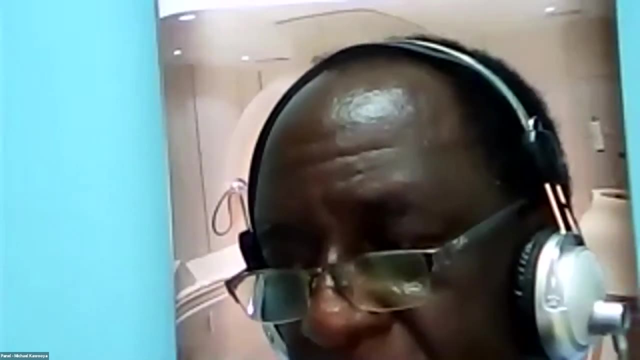 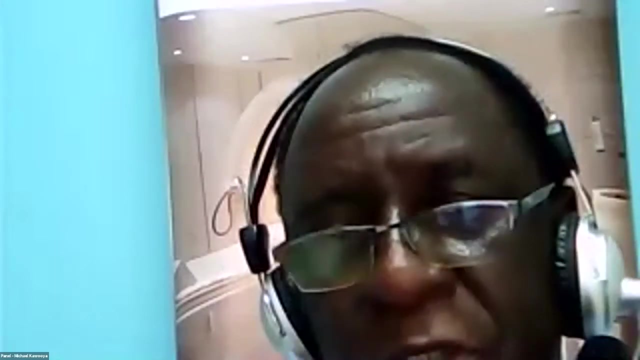 but where there is a little more heterogeneity, where the image is more complicated, then you certainly would need more models because there are several varieties of that disease. But usually the ratio is: we'll have about 70 training data sets to about 10 or 20 of testing and validating. 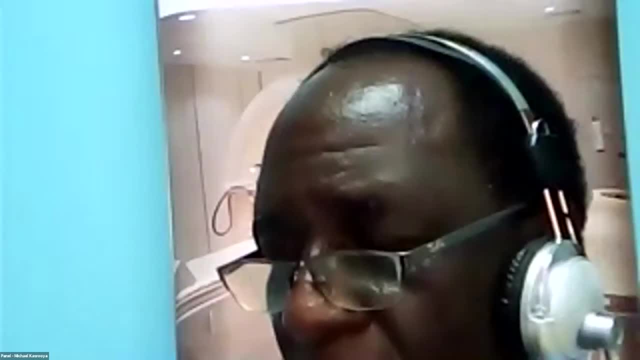 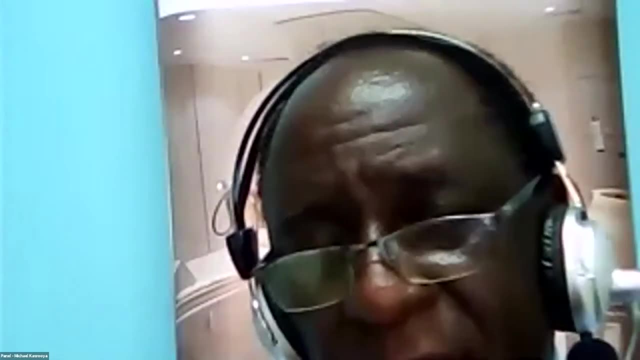 So the that ratio is going to depend on the size, the size of the image, that ratio. one should attempt to have a big training data set and then about 10% or 20% of that as testing and validating data set. Thank you. 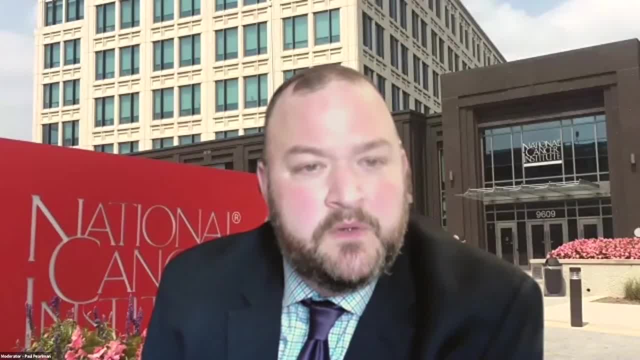 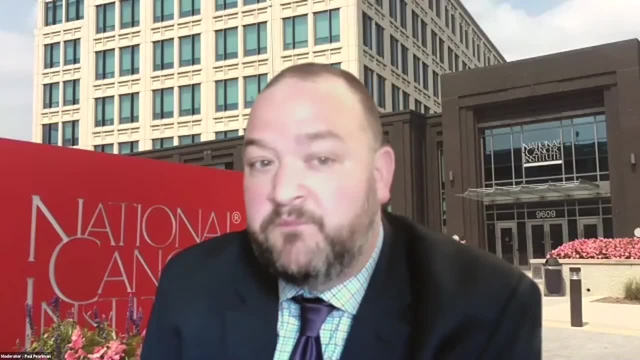 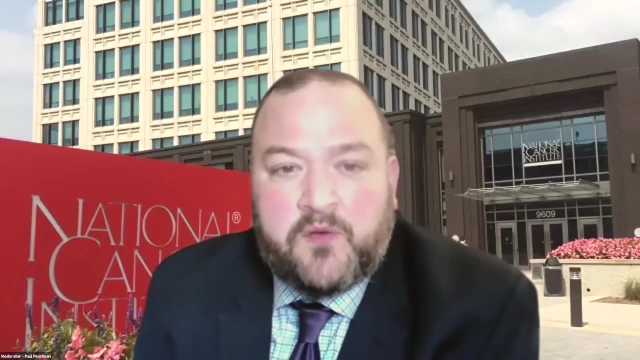 I think this next question could be for everyone, And it asks whether there are international standards for characterizing images that could be helpful for having good data sets. And then there's a second part to the question, where the person asking the question is concerned, that, based on the discussion we've had so far, 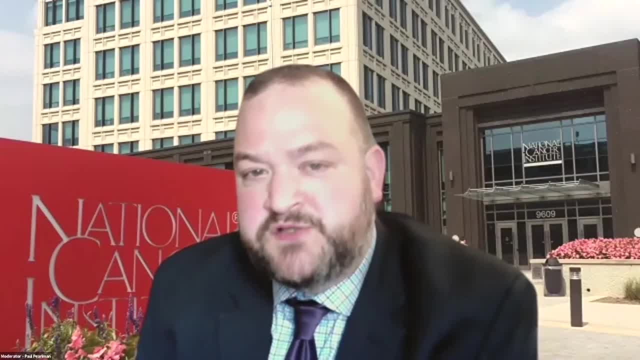 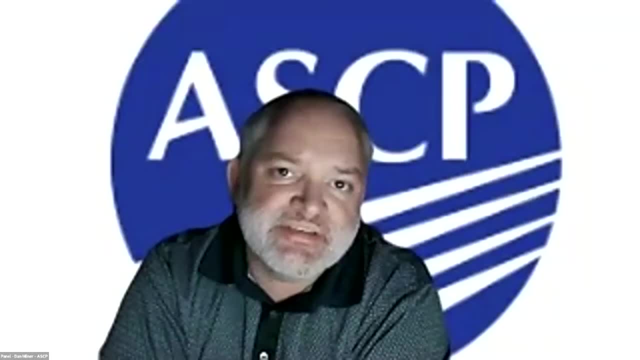 that each research group would really have to collect their own initial images to make sure that they're clean or conform with what is needed for the algorithms. This is Dan. I'll just comment very quickly. For pathology there are, as Samir alluded to: 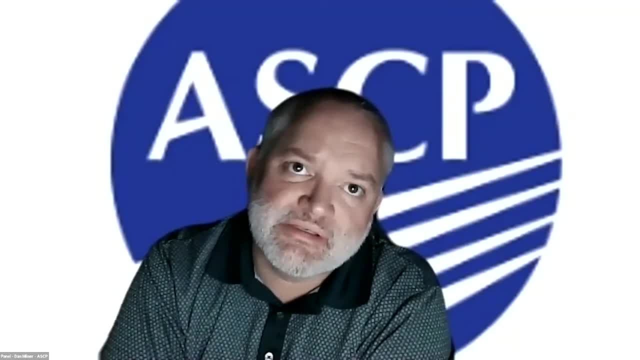 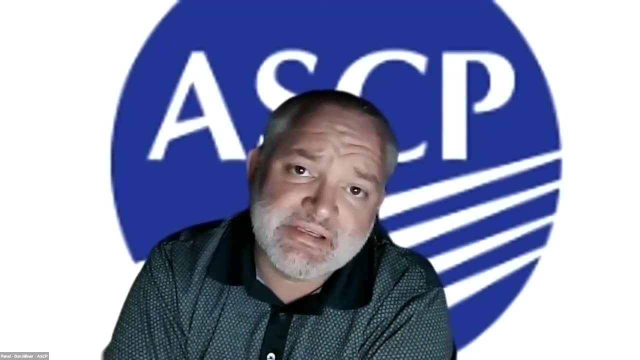 there are standards for how to use full slide imaging systems to collect images. There are also standards for histology quality, cytology quality, et cetera, And those are sort of large and complex But at the end of the day, when you are doing, for example, 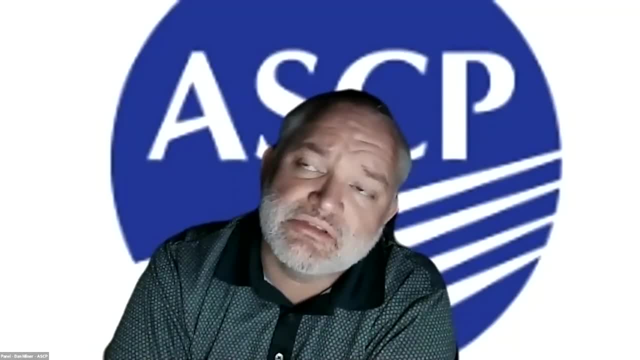 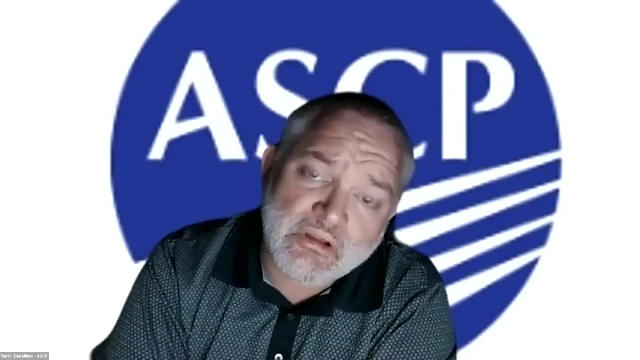 an oncology project or a clinical trial, as could be done in this grant program, and you need a correct diagnosis. there are standards for reporting of cancers, which include all the different features that come from the image, but they aren't about the image itself. 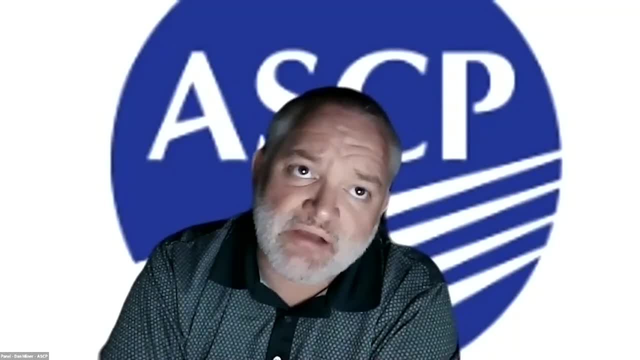 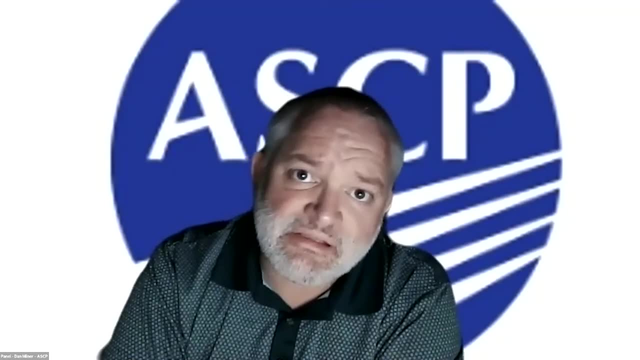 They're about all the other things. So there are quite a few standards out there. And for the second question, I think you know if you are going to collect your own data and I think Celia's point is really well taken. 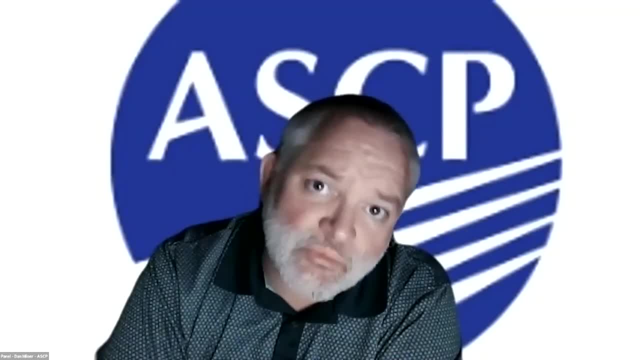 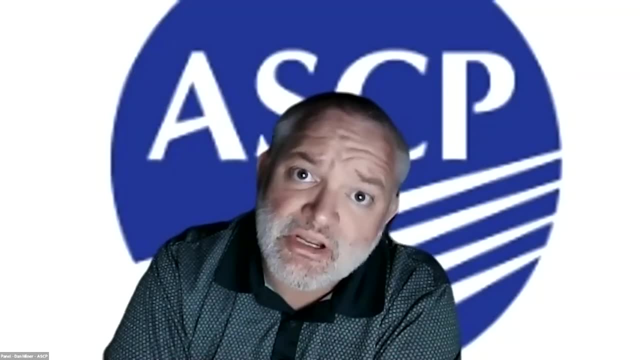 if you're going to collect your own data, likely someone has collected a data set like that before, And so seeking out those existing data sets to use as a comparator, to use as a high quality gold standard against your images, is probably the best way. 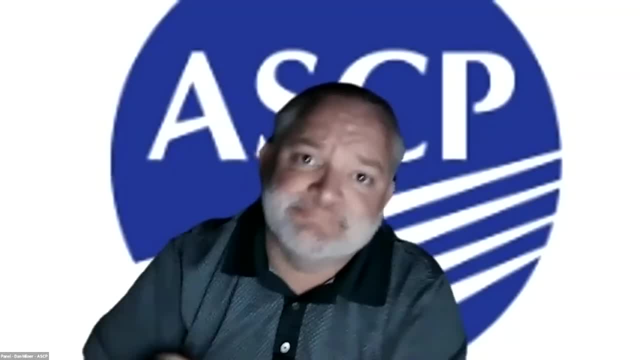 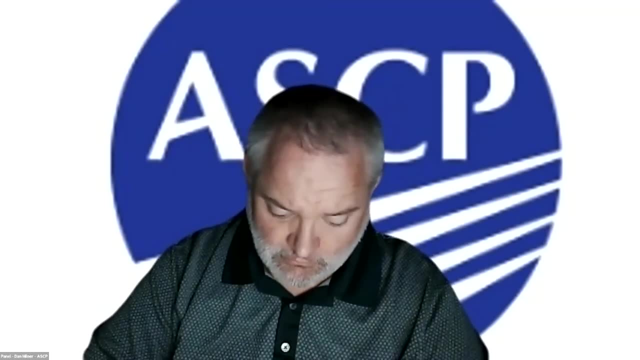 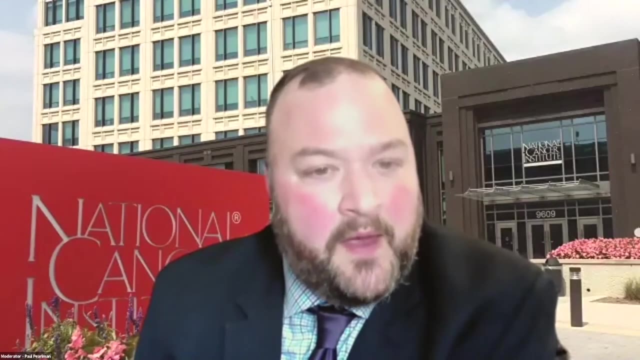 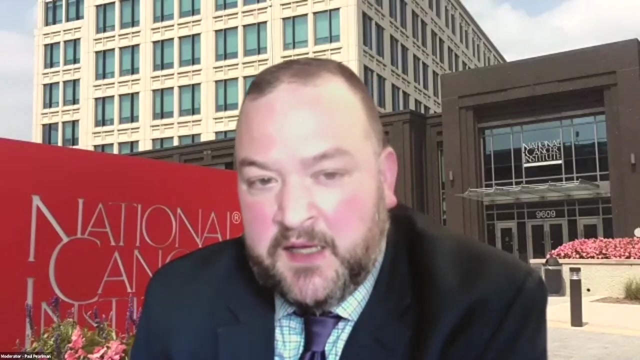 to normalize your data set and correct any problems early on. OK, thank you. So our next question is: what- and I think this is for the whole panel, potentially as well- what are your thoughts on the utility of crowdsourcing or other similar strategies for annotating imaging? 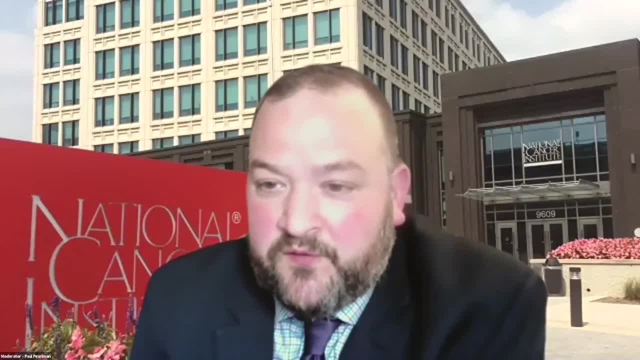 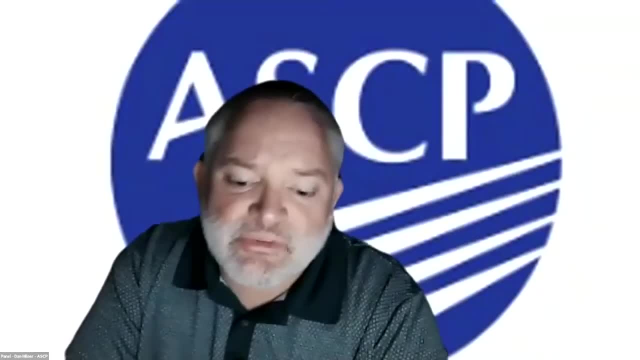 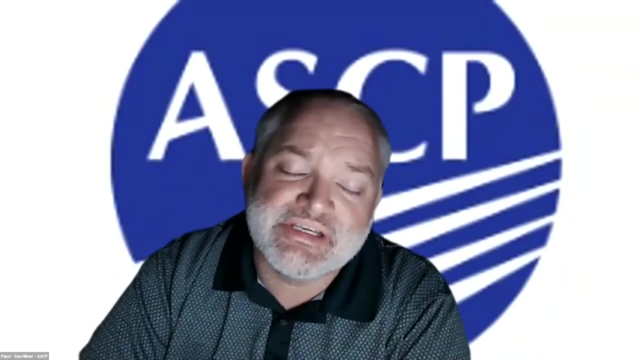 data or pathology data, So the potential role of citizen science. I'll just add really quickly: So part of what we do at ASCP with our telepathology virtual support system is each country where we place whole slide imaging equipment has a team of 15 US-based pathologists. 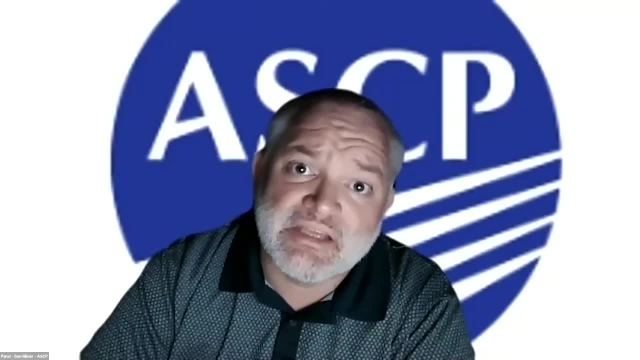 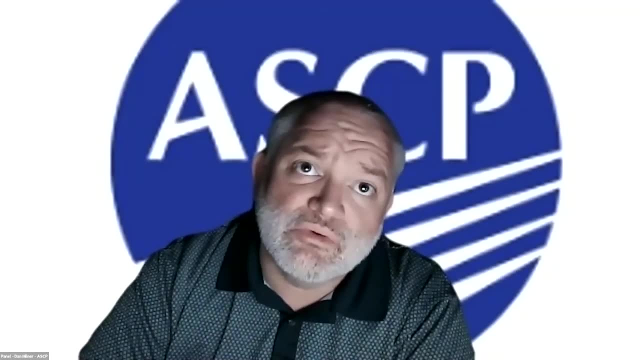 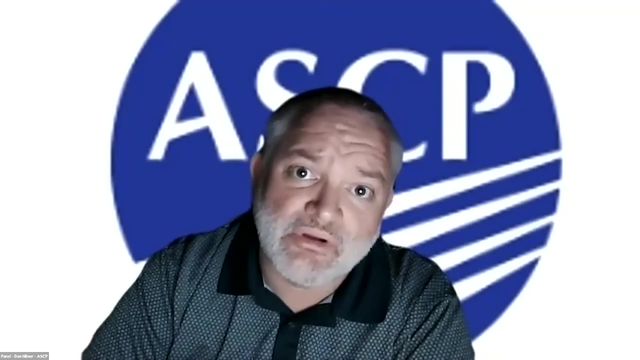 that review those images with them. So if that site decides to engage in a research project, they have automatic crowdsourcing of 15 experts to review their cases. For those of you who are planning on or thinking about pathology, I can offer that ASCP would fully help to support you in that regard. 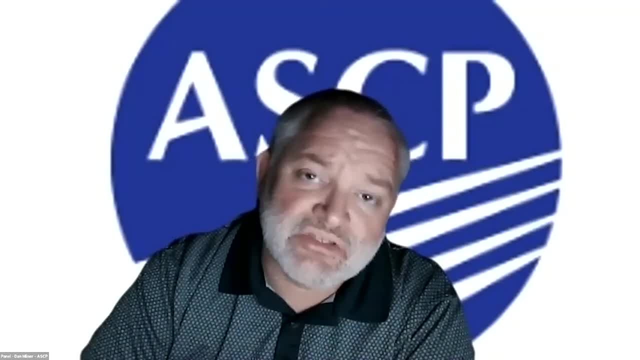 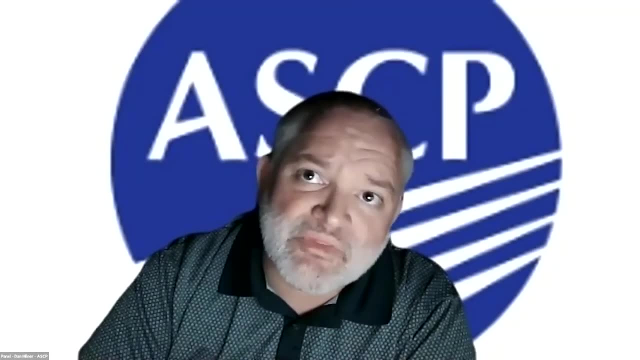 if that's something that would be helpful for you for image validation, And I think it is a very, very vital way to make sure your images are high quality. If you have one pathologist, look at a histology slide. they're about 60% accurate. 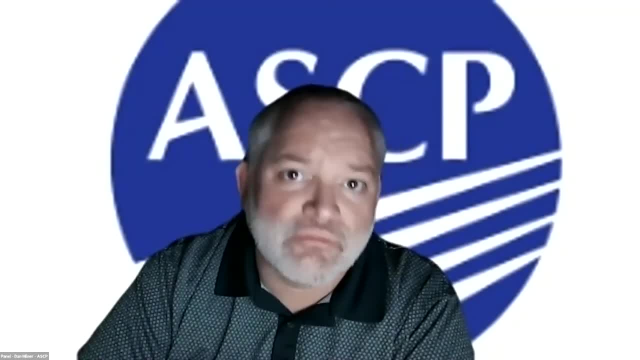 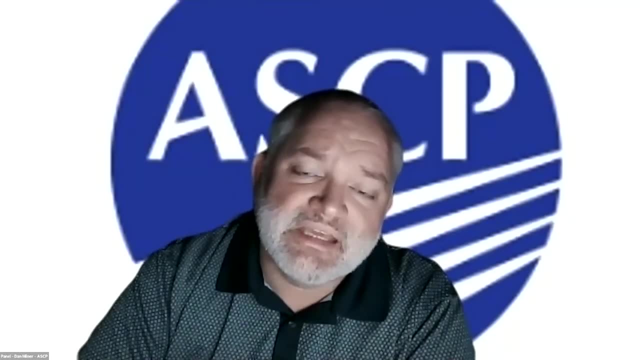 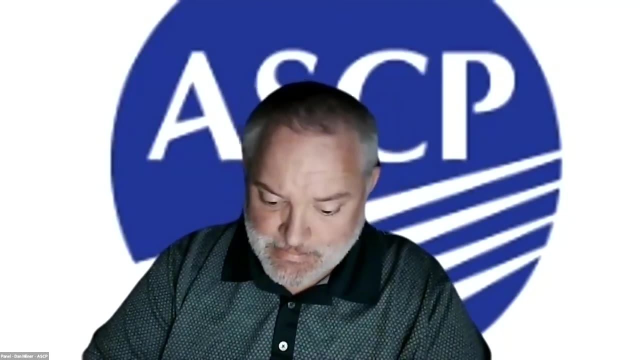 If you have two, they're about 85% to 90% accurate. If you have three, it's a 99% accuracy on the diagnosis. So crowdsourcing is really crucial, especially for complex cancer cases or difficult histology. Any other thoughts? 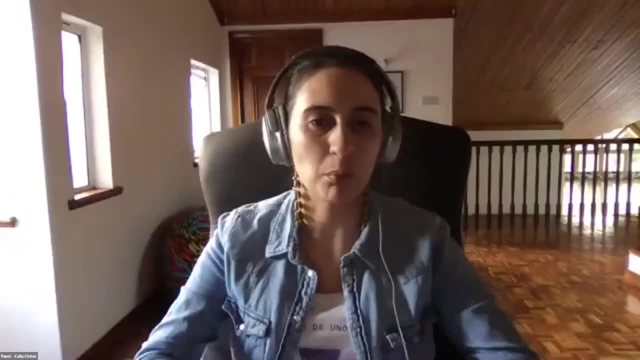 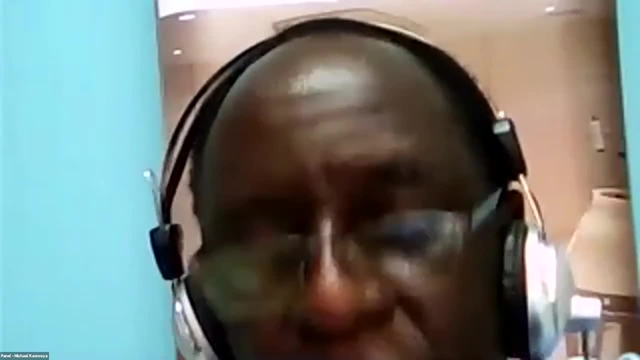 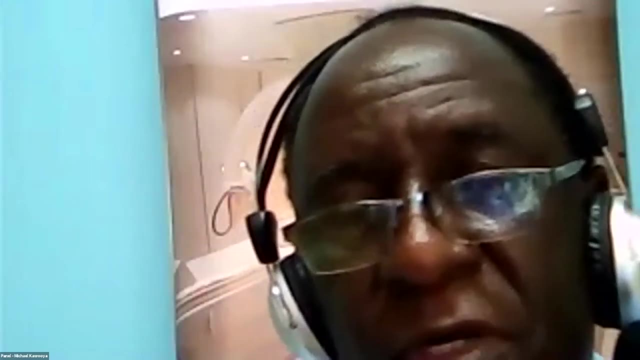 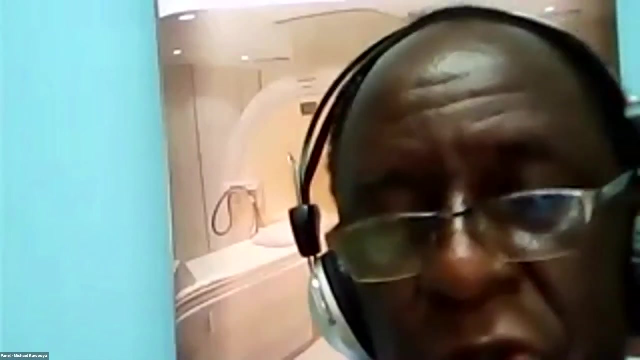 In Africa, where you have limited expertise, certainly would need to have some other person look at it and validate the imaging, And that's why it's important for us to have colleagues in the US or elsewhere who have experience in that disease condition or who see many of those pictures, so that together then 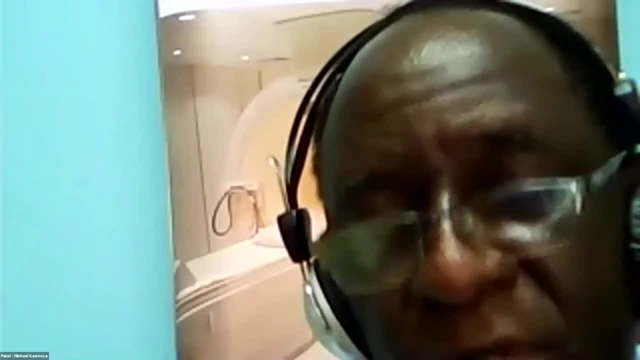 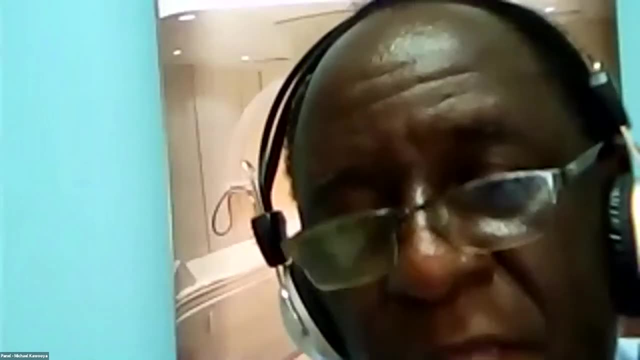 we can have a have a higher degree of accuracy or validity for that image. So for us in Africa certainly it's important that we team up with another university or another research center where they are also seeing many of those images and have more experience than we have. 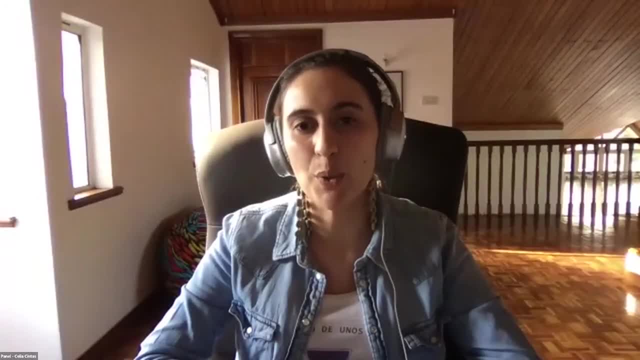 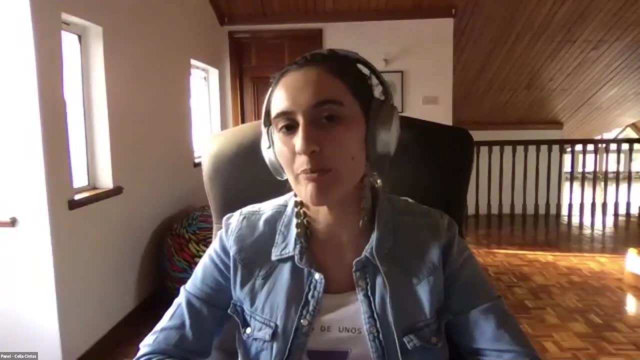 And a small addition to this will be to always keep inter and intra-observer errors measurements when we use crowdsourcing. So it's important to keep in mind that there's a lot of evidence to be found on the data set for using the data set. 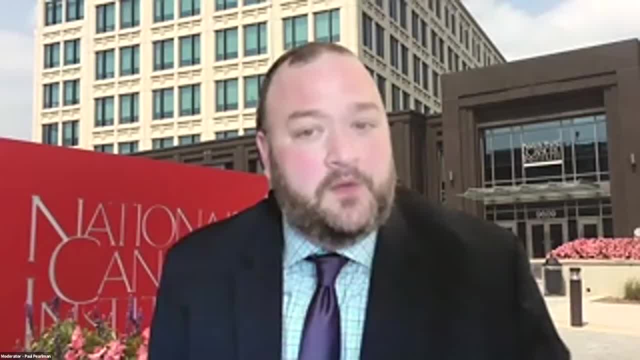 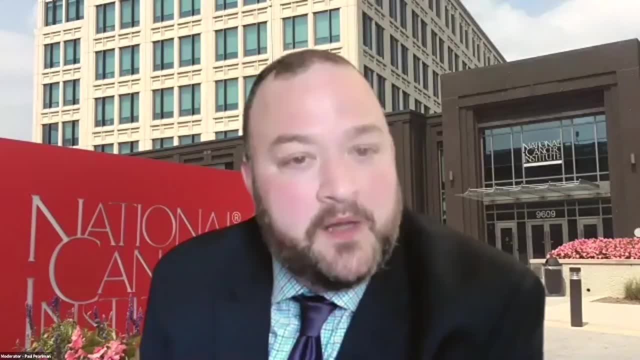 And there's a lot of evidence to be found to be used for testing the data set. So if we can't do that, we have to try to minimize the evidence that's being used to find out where the data set is, And so if we can't do that, then we have to keep in mind 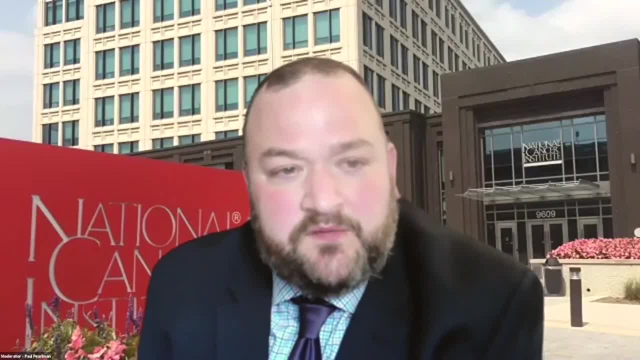 that we have to keep in mind that the data set is not going to be long or long enough to be reported next to the data set and the labels. Okay, I'm afraid Dr Milner is going to have to drop off of the panel. 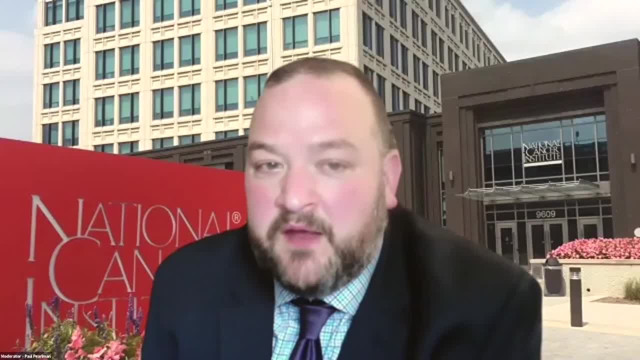 from this point I want to jump into our next question. So the question is that it seems that good machine learning predictions can often disagree, And the question is whether any new disease mechanisms or insights have been derived from ML- machine learning predictions that allow pathologists to 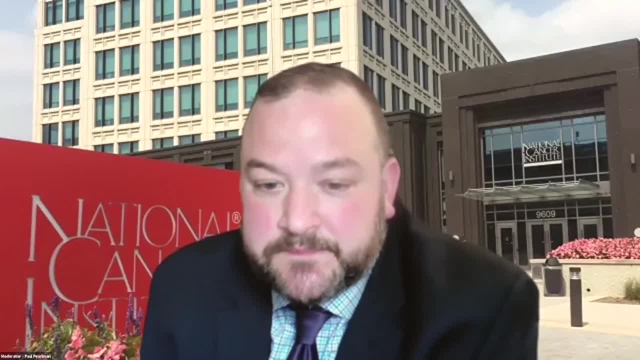 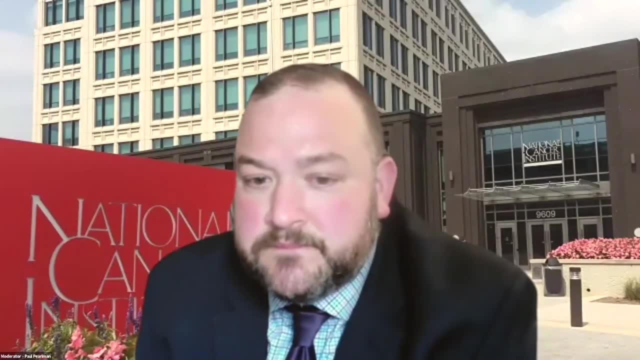 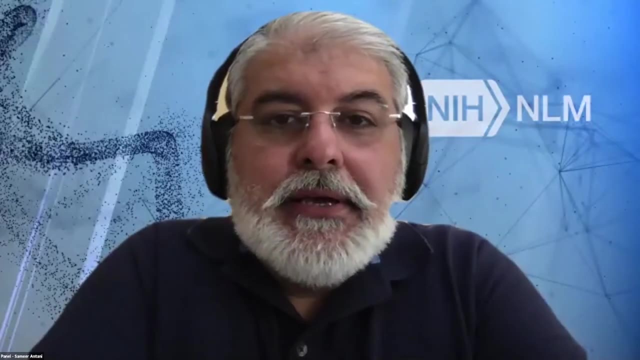 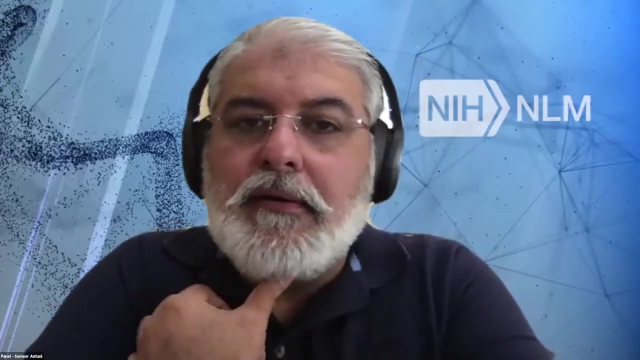 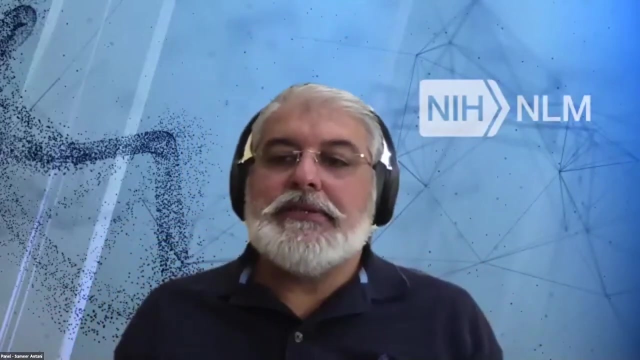 assess sort of new ground truth. I can't answer for pathology- I mean Dan's dropped away, unfortunately- but in the limited experience I have with finding so question is the way I would cast this question is: if different ML predictions disagree, is the disagree if and we agree that what it has found? 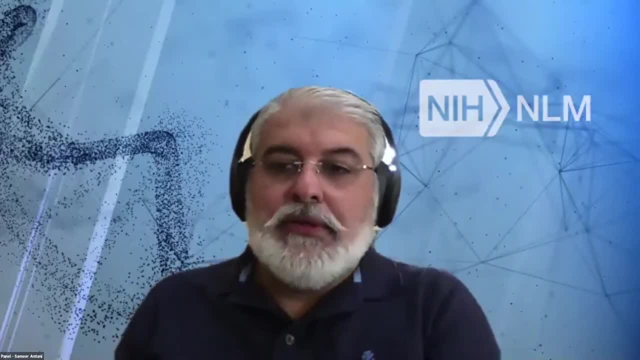 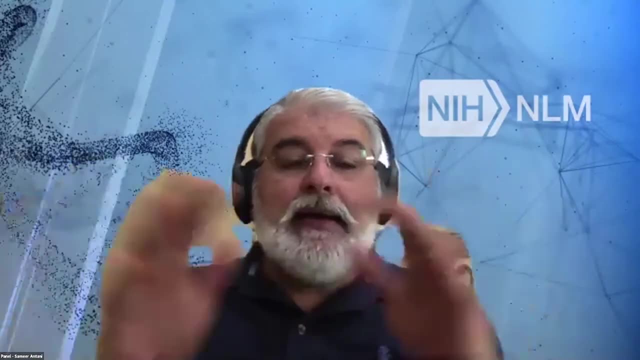 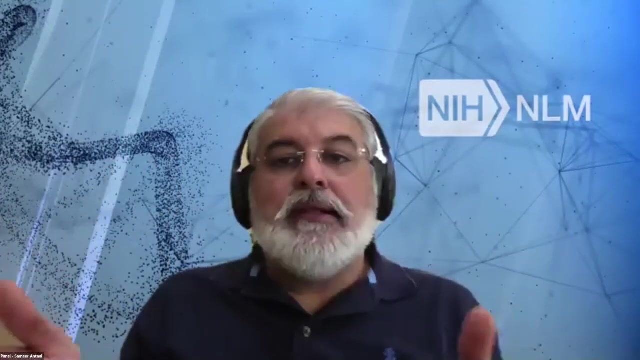 obviously deviates from ground truth, unless a ground truth was a, was a an aggregate label, so you don't know where the disease is, but that the ground truth is not the cause of the disease. So if the ground truth is not the cause of the disease and if this entire image represents 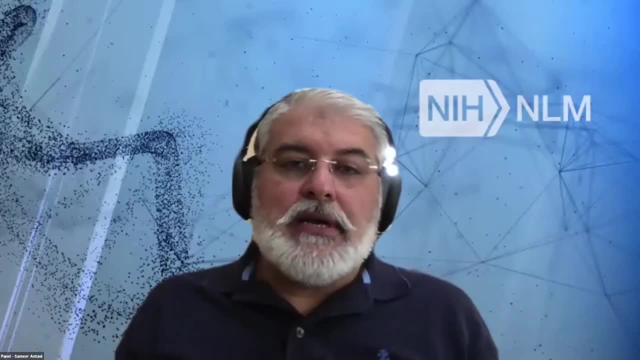 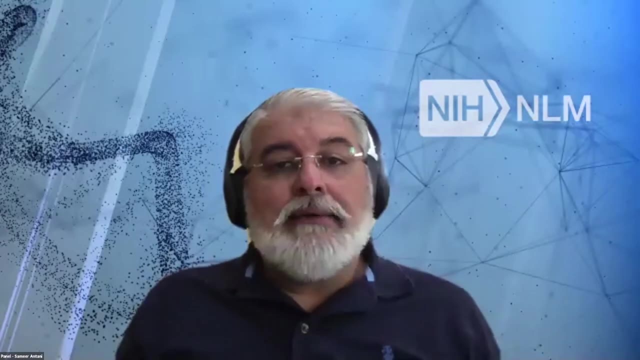 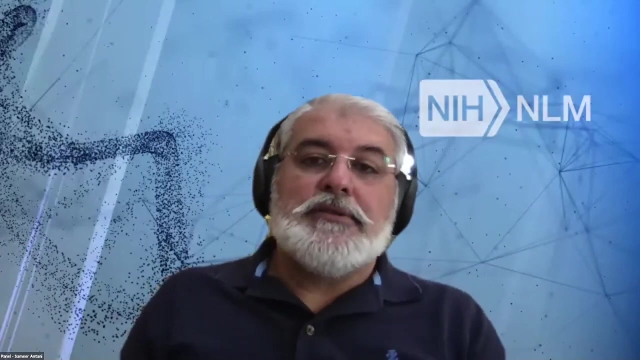 disease somewhere, then human expertise could step in and verify if the highlighted regions are indeed diseased and if there are any correlates there. However, if you do have localized truth, then the immediate response is that, or the naive response might be that, if the 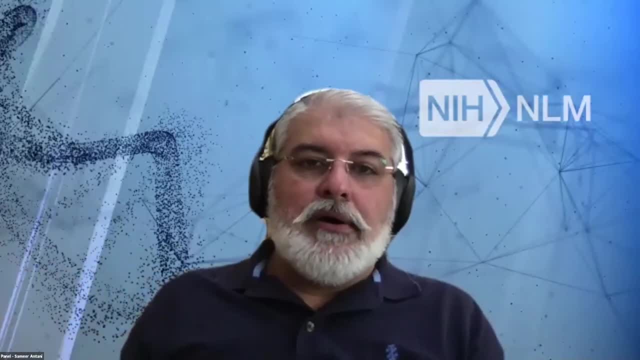 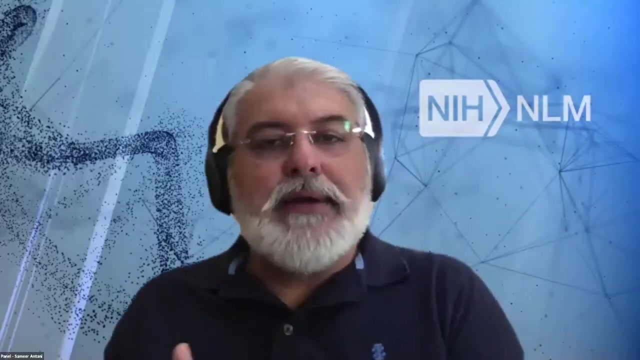 is a surrogate or an alias of the true region. is it really a false positive or is it something indeed new? is it a correlate? And that again goes back to away from computer science and data science into the into interaction with clinical experts or biomedical experts, to see if this is. 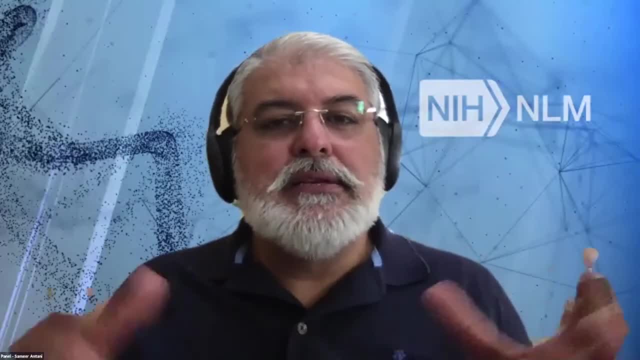 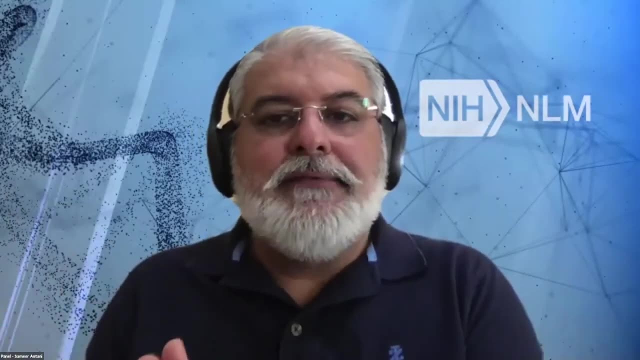 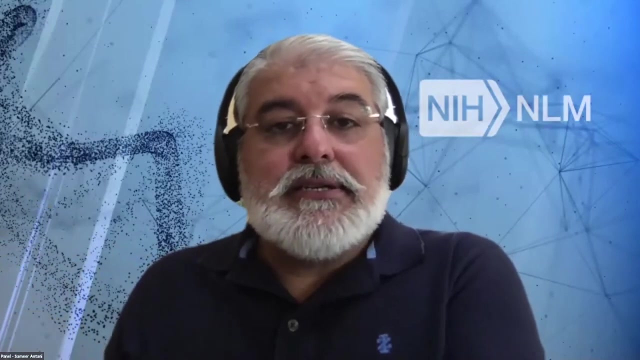 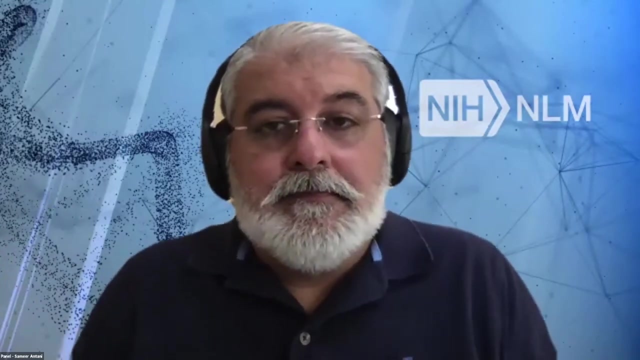 a prevalent condition that is seen widely across the population of the of data being analyzed, or is it an outlier? And if it's an outlier, are there other information in other records, other tests that might suggest that this is a meaningful fund? Okay, if I understood the question. in imaging, for instance, there's been a lot of progress with. 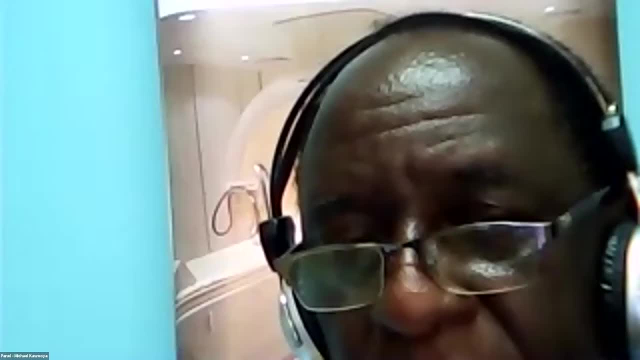 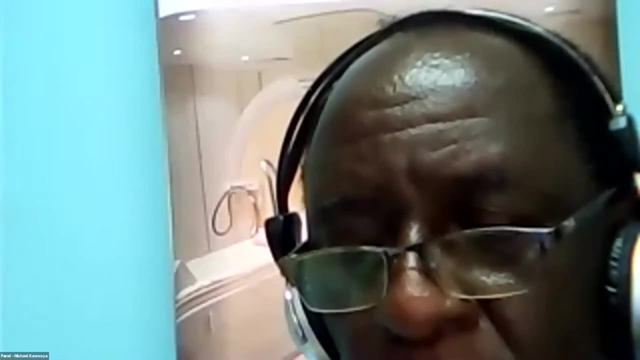 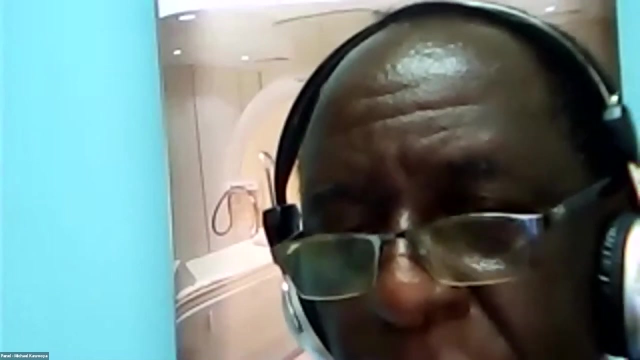 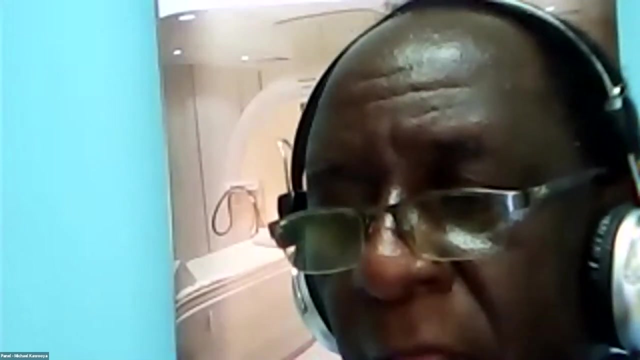 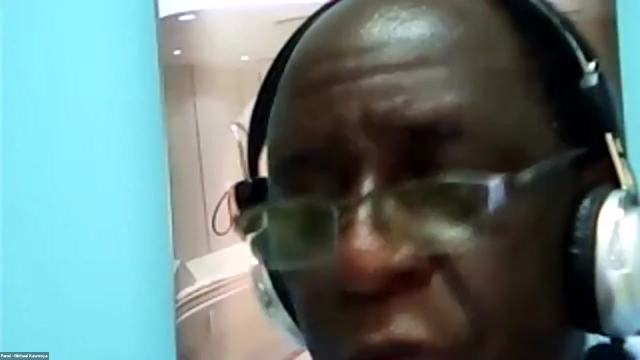 glioblastoma, which is a tumor of the brain, in MR and we see now that MR may help to make a difference between the different type of glioblastomas- the mutant type and the wild type- using machine learning, And the naked eye may not be able to pick those differences between those mutant varieties. So in 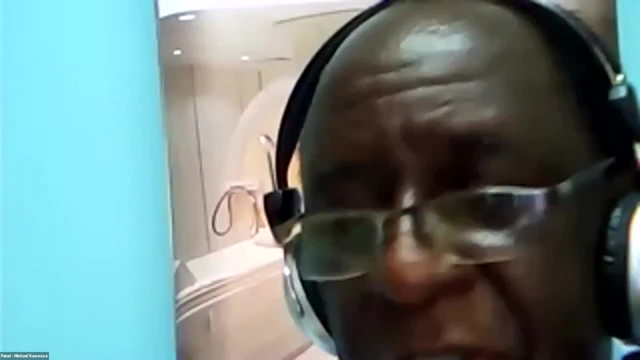 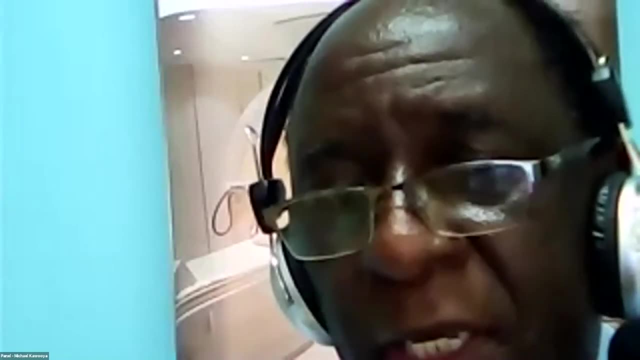 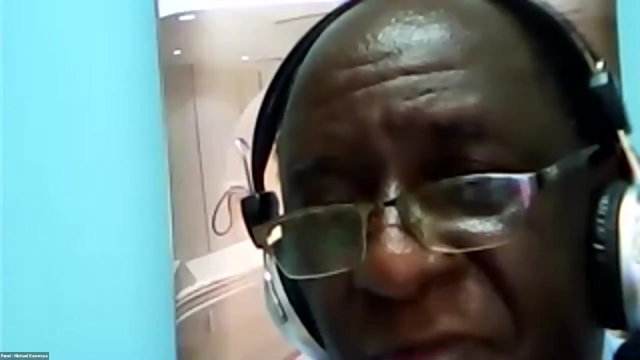 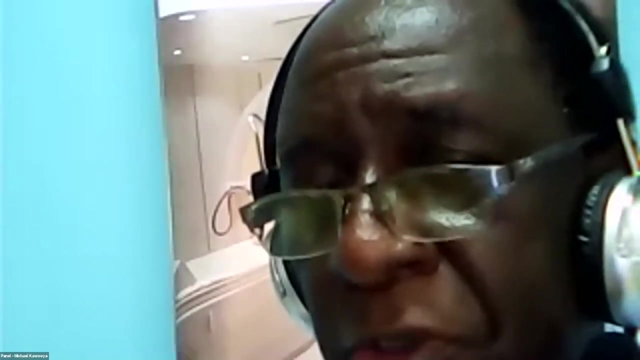 other words, machine learning or artificial intelligence sees what the eye cannot see and can, and this correlates very well to biomarkers in molecular imaging, because the biomarkers for the mutant type of of glioblastoma are different from the biomarkers for the wild type of glioblastoma, And artificial intelligence can help us to sort out this, whereas 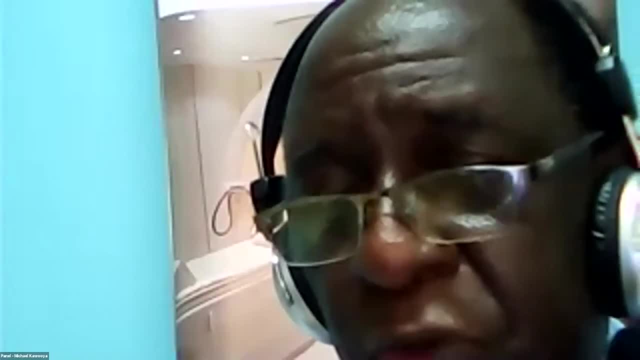 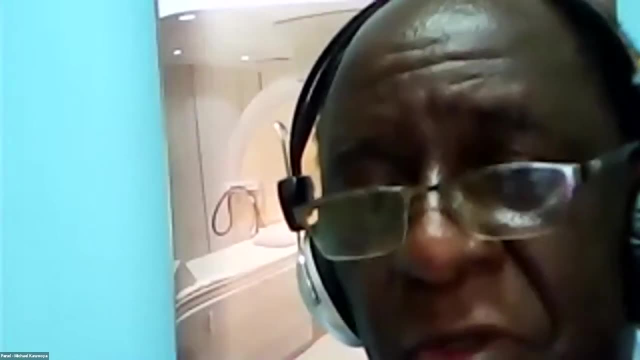 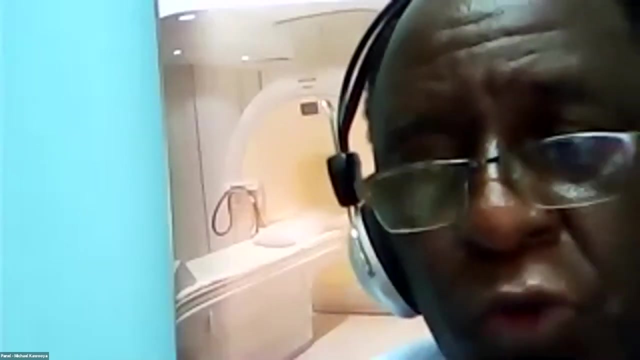 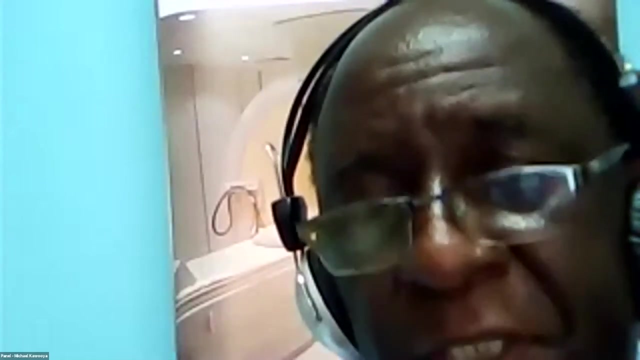 the human eye may not be able to make that difference between these two varieties of glioblastoma. So there are areas where artificial intelligence has gone a long way to see what the eye cannot see, and helps us even to be able to predict what the molecular type that may be, whereas the eye cannot predict that. 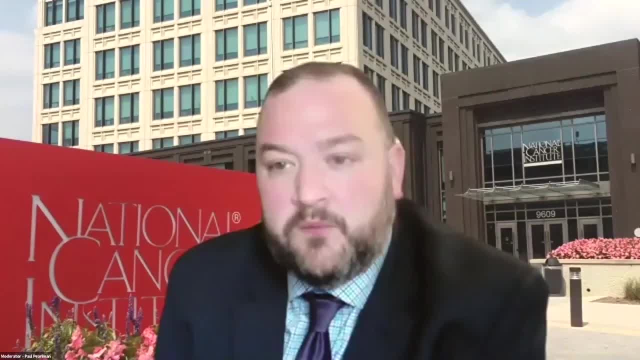 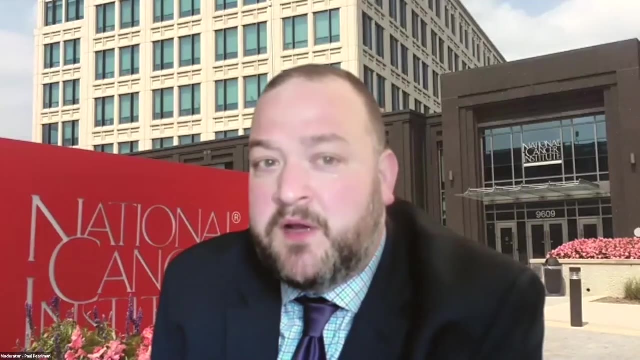 So I've got another question and I want to start with with your view on this, Celia. The question is where individuals can go to learn to build some of these machine learning models, and is there computing capacity in Africa for building and interpreting machine learning and? 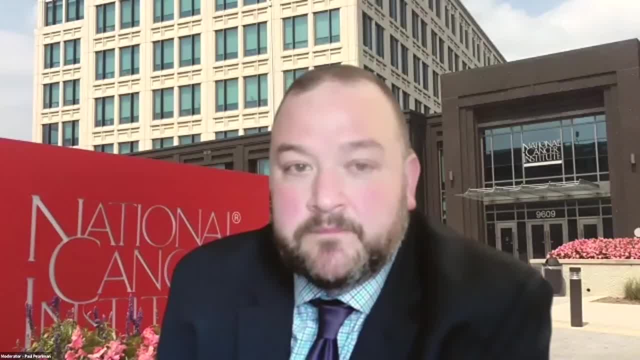 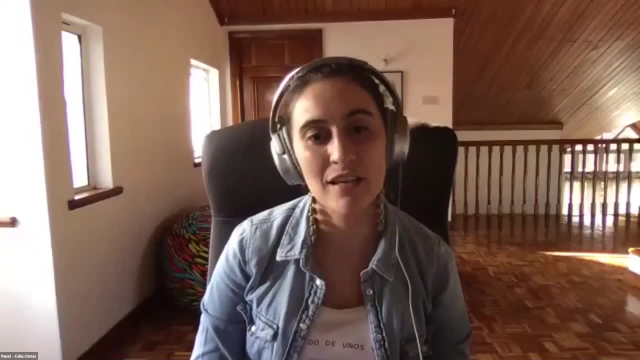 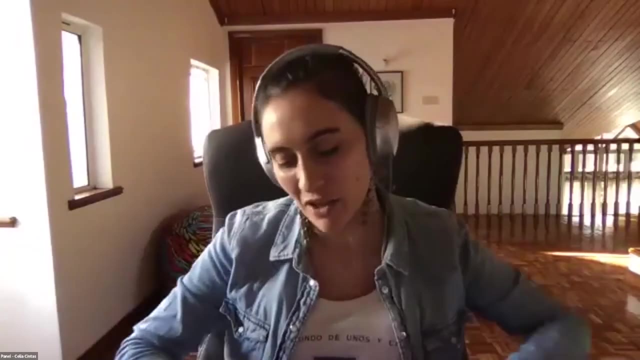 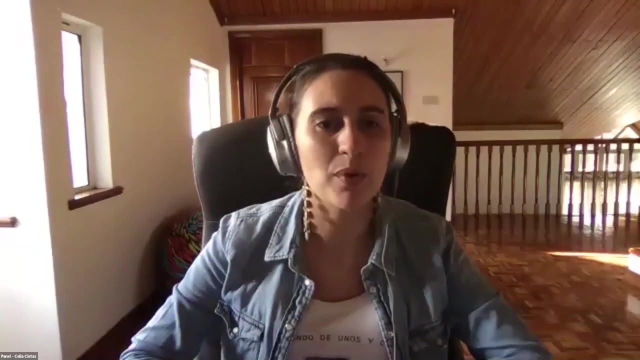 AI solutions? Yes, definitely So. our lab has a stronger relationship with the School of Engineering in CMU in Rwanda. We always have a great network of master's students from the university, so I will definitely recommend those programs. IBM also hosts several courses with machine learning basics, also blockchain and other. 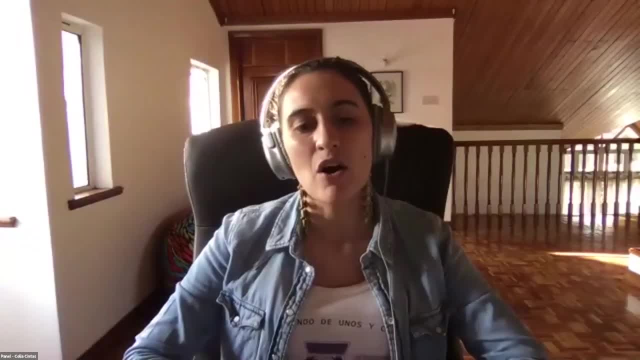 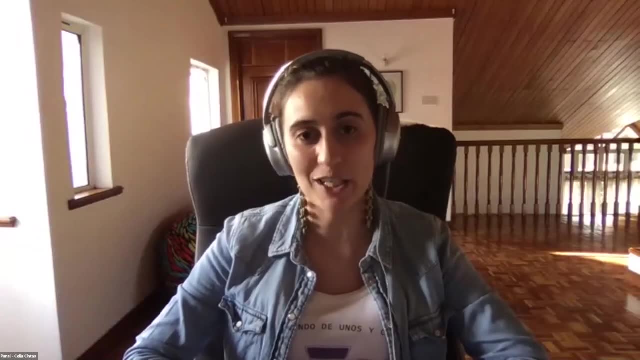 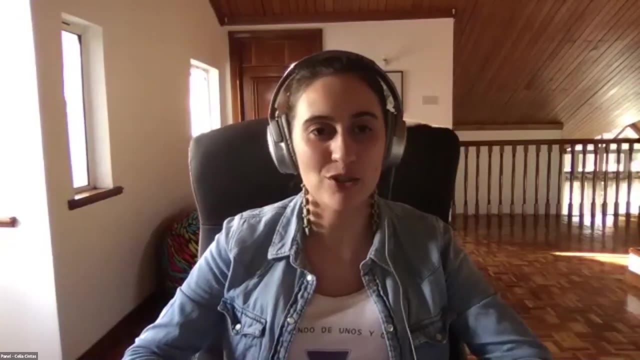 similar topics. Hopefully, year by year, we see that all these models are being able to run in cheaper and cheaper hardware, so this is great for everyone. Also, if we have a project with some of these models that doesn't have access to big clusters, 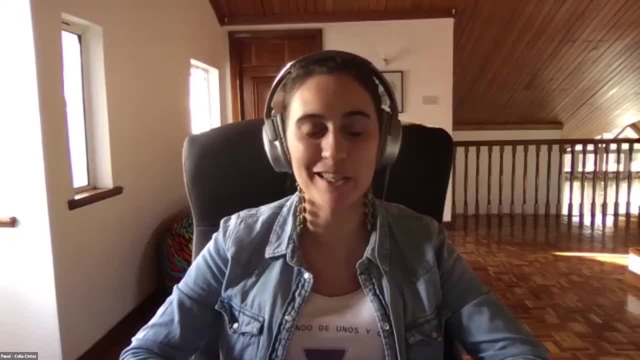 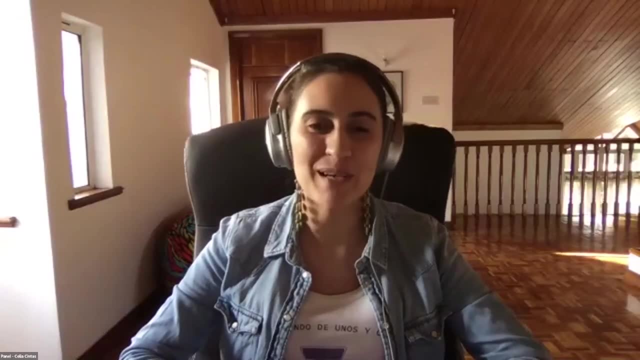 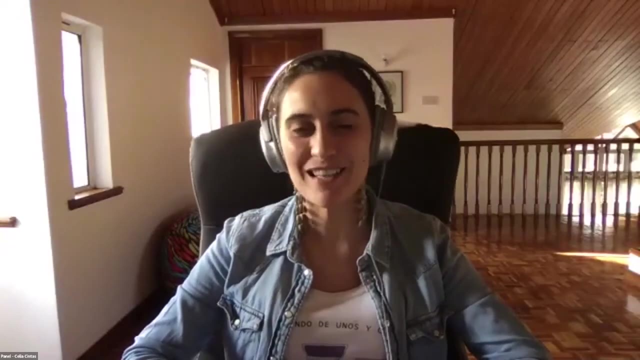 and so on. They can still with a few notebooks or a small small cpu. they can still run experiments. Also, all the portraying models that we can access, all those need neural networks have been running for weeks and weeks in millions, of millions of samples And we get those fine tuned matrixes, values in our 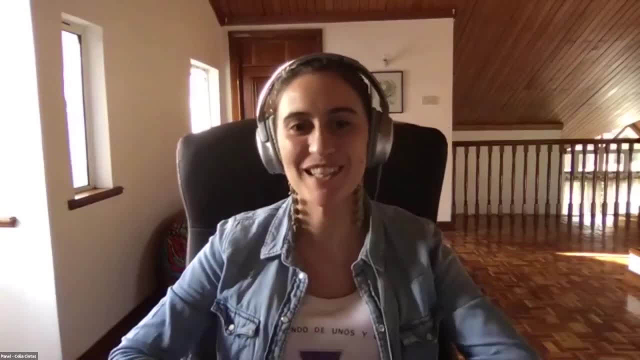 computing system. So we are using a lot of knowledge and knowledge of the need of maternal intelligence. This is gonna be useful for us. I also think there has been a lot of research in our computer with zero computation cost and usually we will train with the. 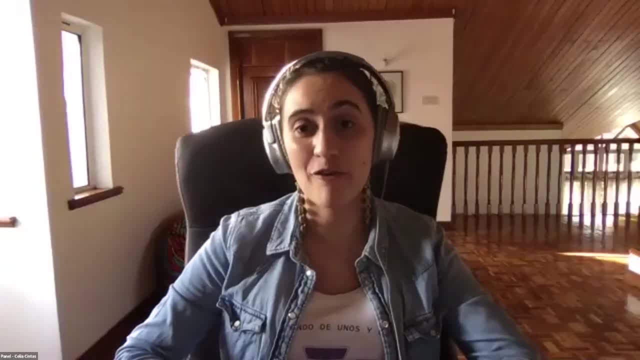 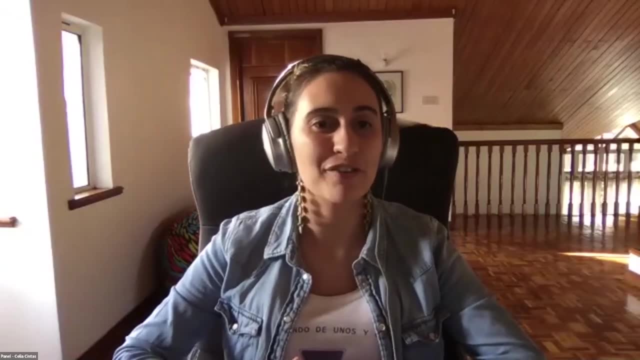 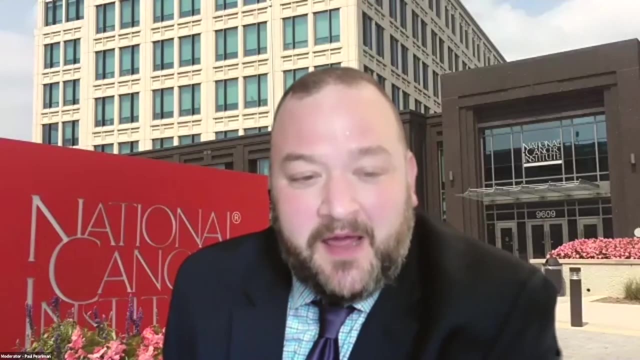 smaller, that sets. so I will say yes, for small brands, of course, we have the capacity, and for bigger, of course, we have the cloud, thank you. so I'm gonna ask one last question, and and it's the question is why, by and large, are many of these machine learning and AI tools not yet being used in clinical settings? 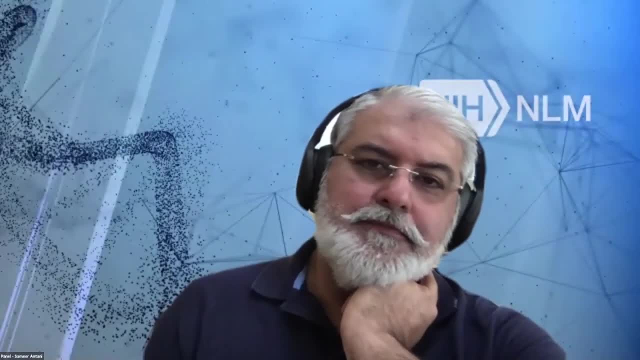 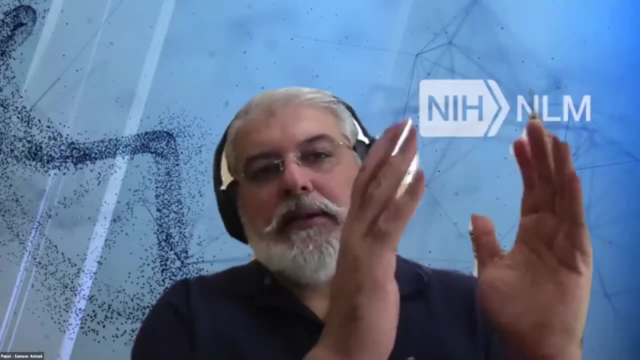 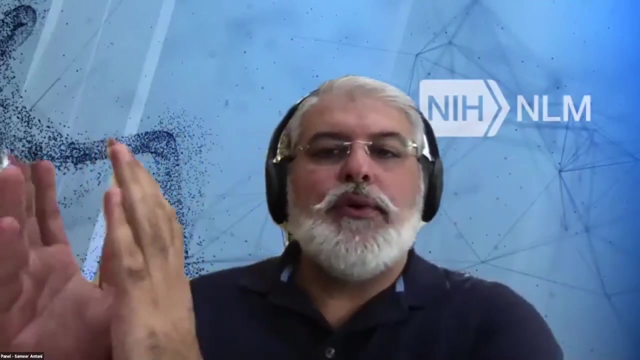 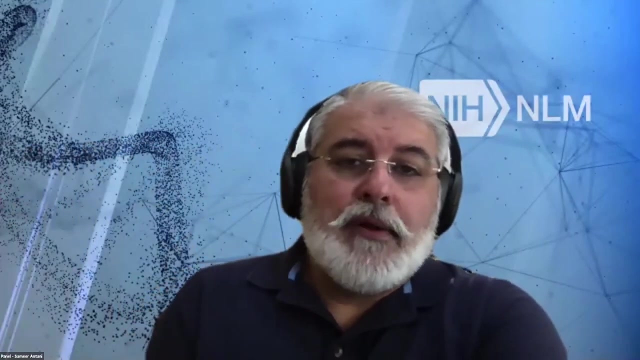 that's a tough one to answer because a lot is, I think, in between, between technology, that is, the developing a machine learning tool, developing, even, even say, a product to it, fitting into a particular clinical protocol. there are many steps and they include approval from, in the us, the FDA or appropriate. 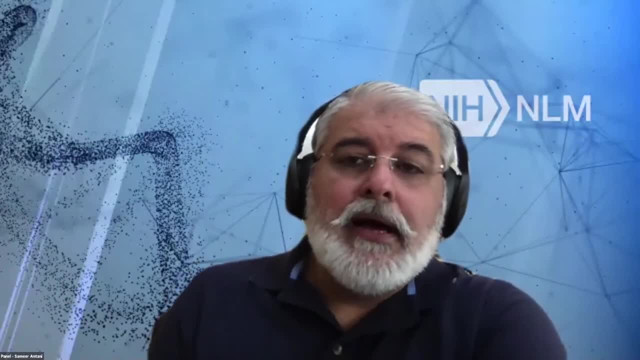 health ministries agencies in respective countries, acceptance by the community of how they would translate results from a machine learning model to clinical practice? merely a classification score or is it a prediction of risk to the patient that would suggest an appropriate intervention for the right member of the community? Is it, for example, 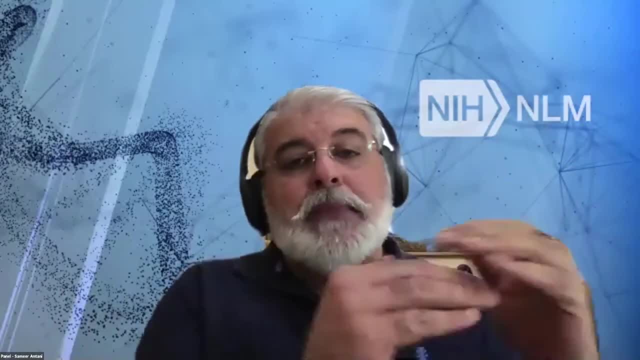 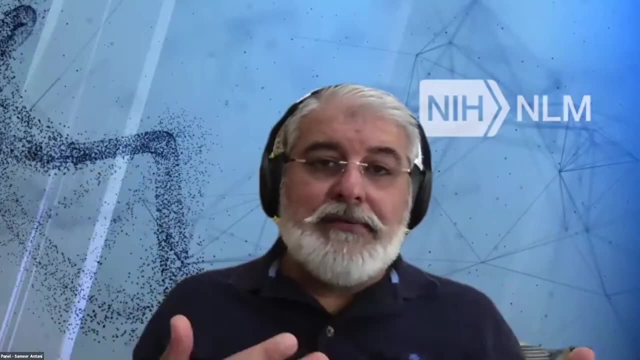 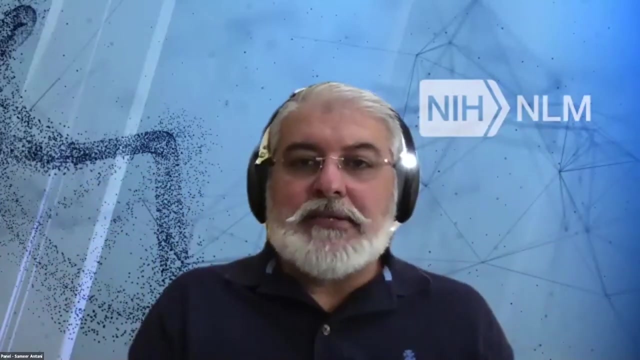 from a pathology standpoint, it might be as naive as highlighting regions to look at, which of course reduces the time and there is a performance metric there, but if you skew away from missing any cases, you allow false positives. You still have saved time, but you will not risk. 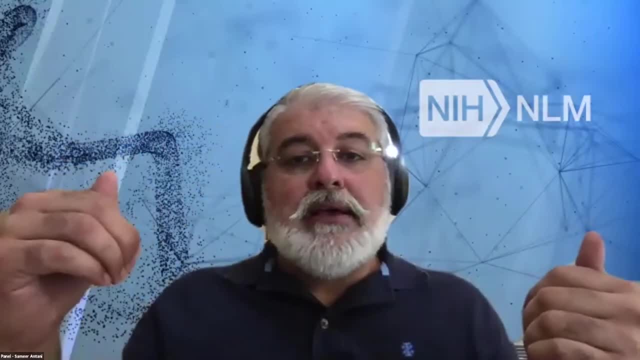 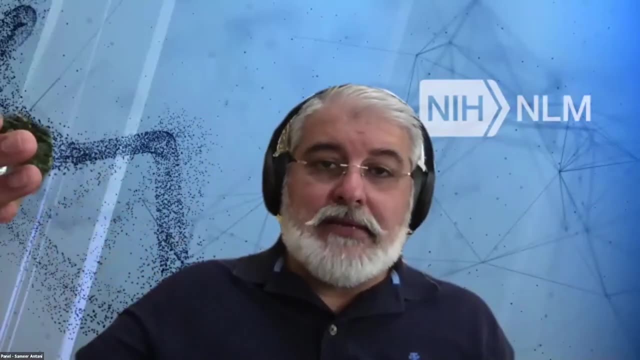 losing the patient. However, intervening from a surgical standpoint, when the patient doesn't need to be intervened or you are in the midst of a surgery, you can imagine a live system as an AI system that is serving as a guide and you have an unnecessary excision. Now, the risk is much. 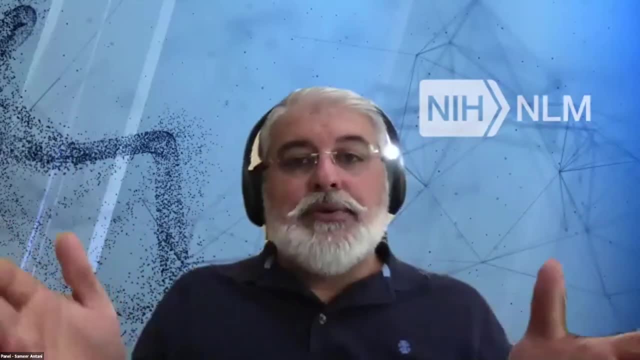 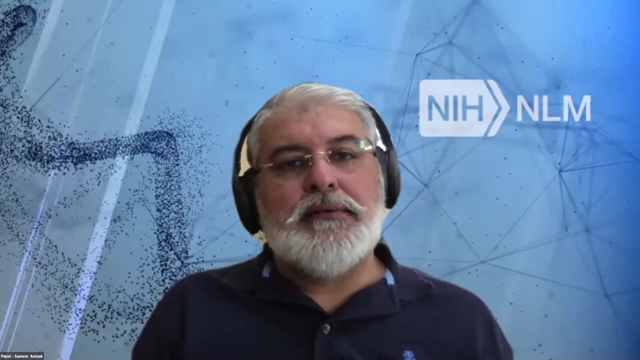 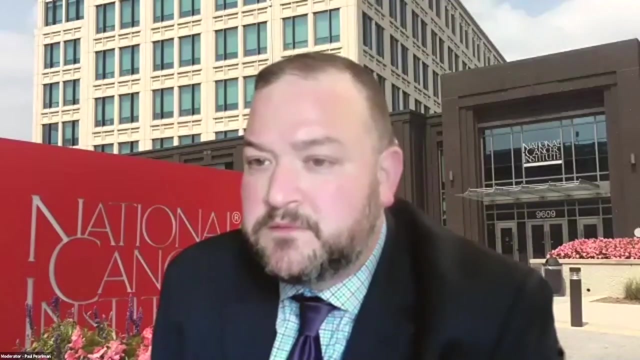 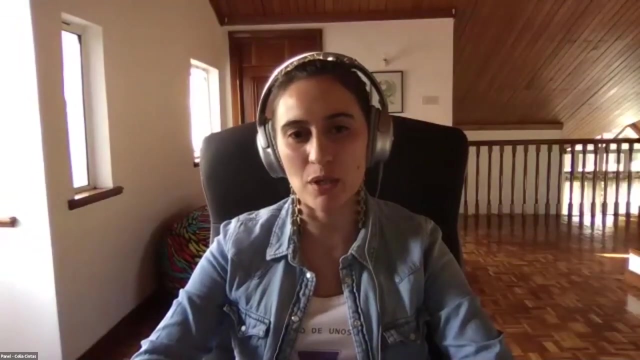 greater. So there are several factors that play into it. that mostly allude to risk approvals and acceptance by the community and other factors. Anyone else want to add to that? Yes, I think, for a machine learning perspective in clinical settings. I think we will get to the point to. 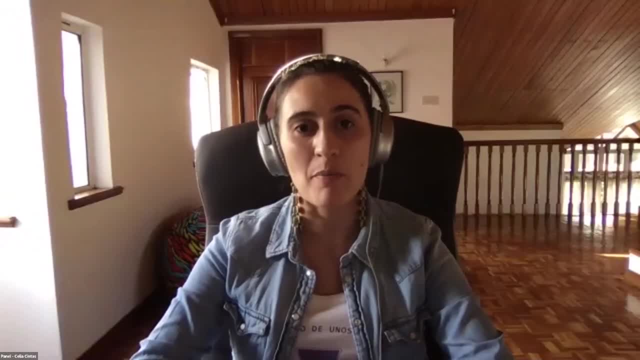 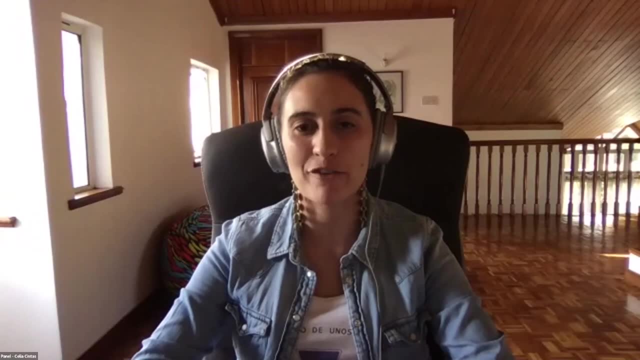 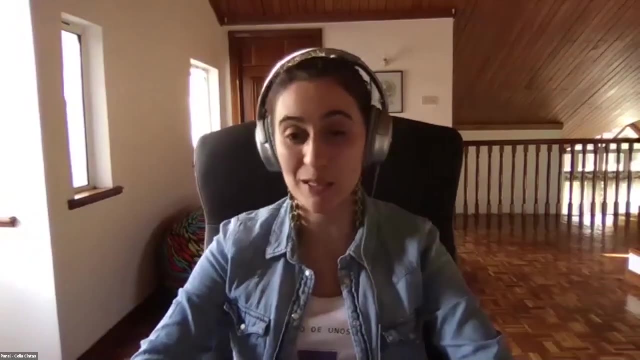 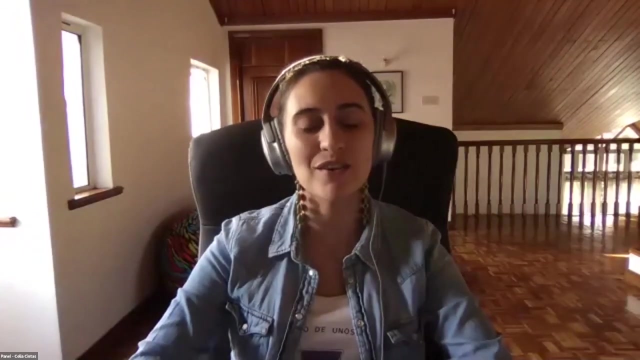 help professionals to make decisions, but currently we cannot allow machine learning models to make their own decisions, as we don't have clear transparency on how the decisions are being happening or over under what population this model was trained And, given that health is such a critical thing, we can hope for this type. 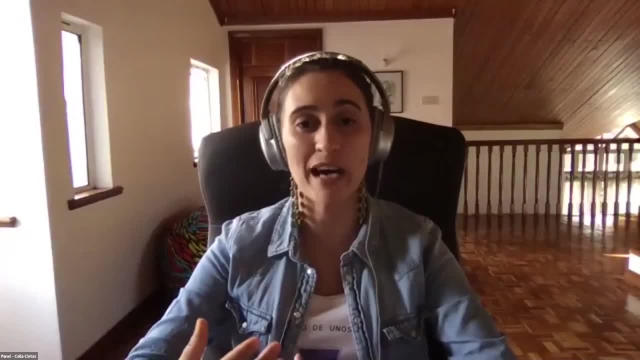 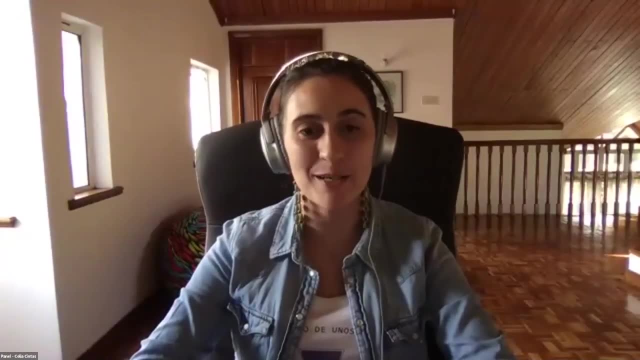 of models to assist professionals to see different patterns that maybe they wouldn't have access to, or see other second opinions. let's call from machine learning models. I think that is going to be more viable but, as you said, it's not going to be easy and it's going to take a lot of time. 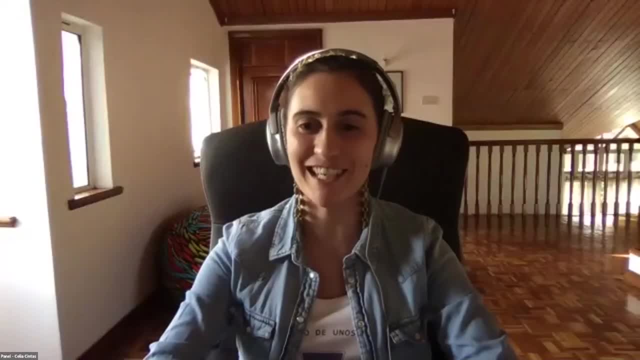 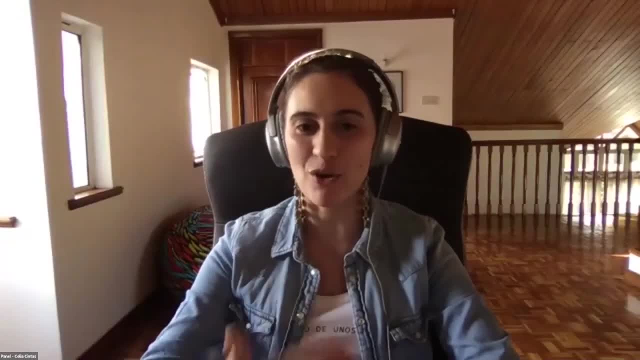 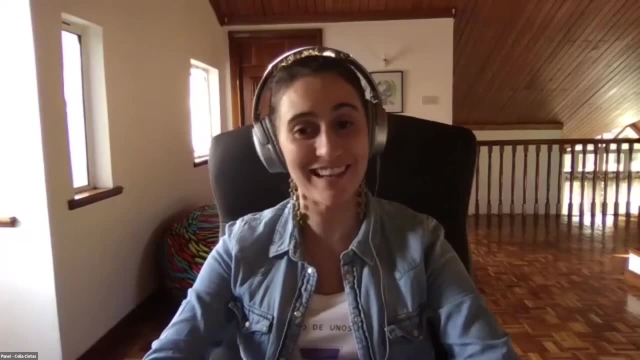 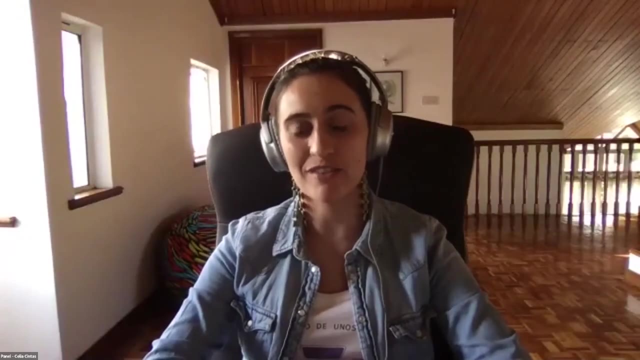 you need a Cambria approvals. you need to go over a process of ethical consultants, see that you are compelling to everything, as any product, as anything that gets to a clinical environment. There are a lot of regulations and we need that. the models that we deployed: 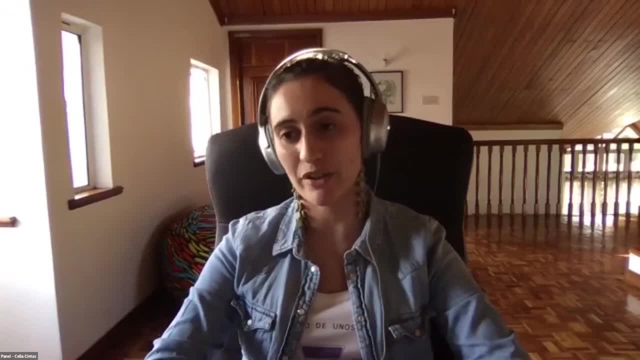 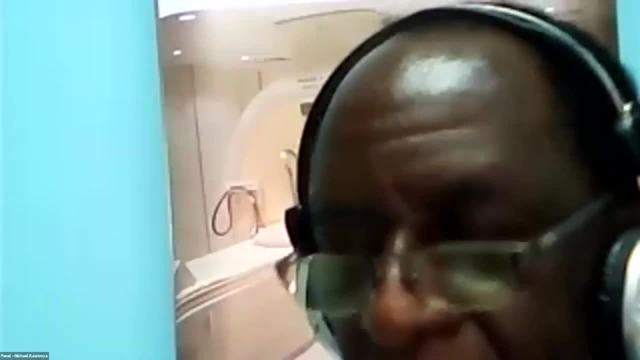 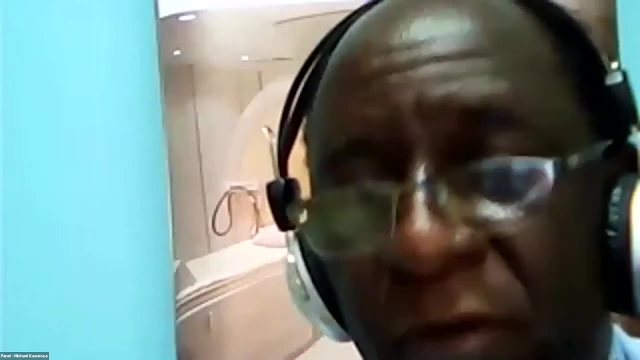 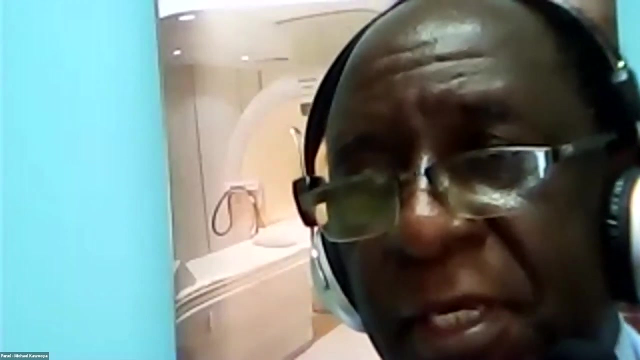 are being transparent and know the limits of their support. I also want to add that artificial intelligence and machine learning is something very new to Africa and many doctors, many practitioners are not yet used to that and I think we have to see how can we get this into the curriculum for undergraduate and 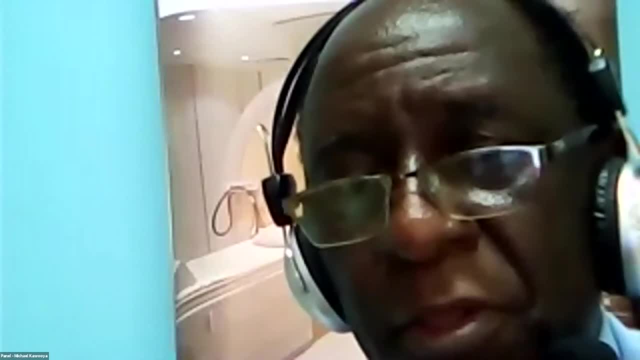 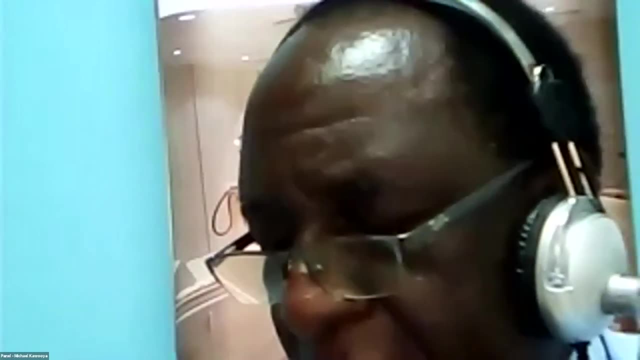 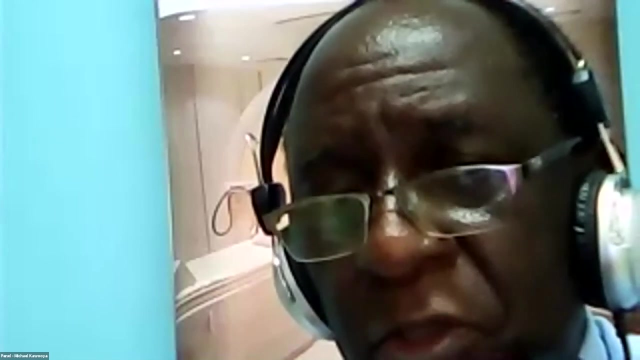 postgraduate training so that they know the benefits of applying this in routine clinical practice and where it's applicable. So I think that training is important. and then, secondly, it's also the relevance: if it does not address a clinical challenge, a clinical problem which I encounter every day, then I'm 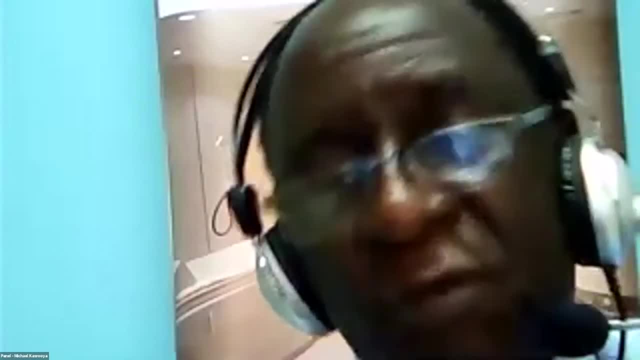 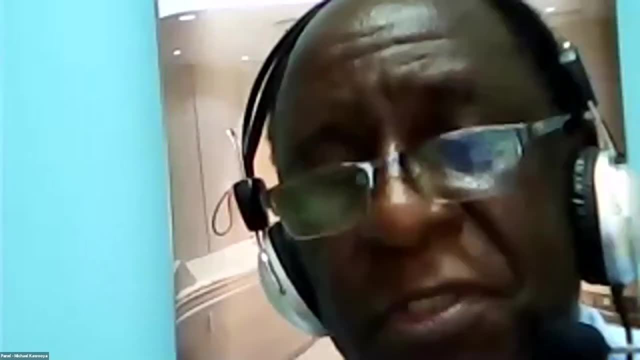 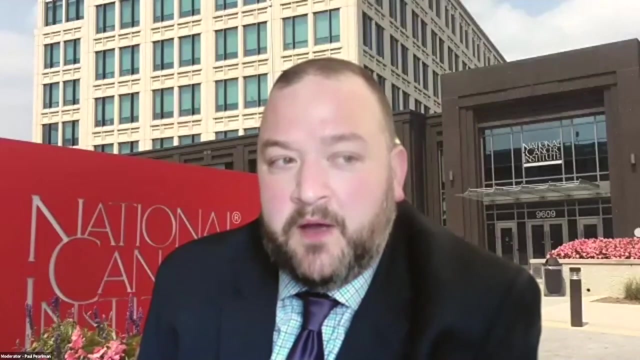 not likely to use it, but if it addresses, if it's relevant to my setting, my healthcare setting, then I'll take that up, Plus, of course, the ethical legal implications, as already noted. I guess I would take the risk, as a moderator, of adding a thought as well, and that's that. 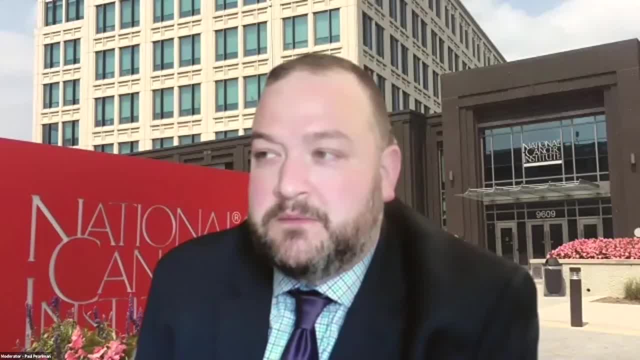 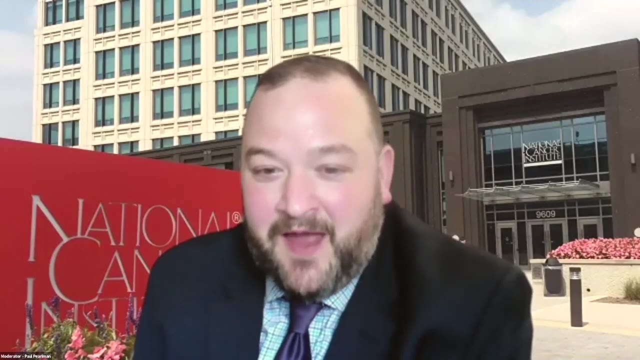 the regulatory science is really developing in parallel, and only recently have we seen sort of machine learning and AI, specific regulatory pipelines from our FDA, and so a lot of this is still happening in real time. With that said, we are out of time for new questions. 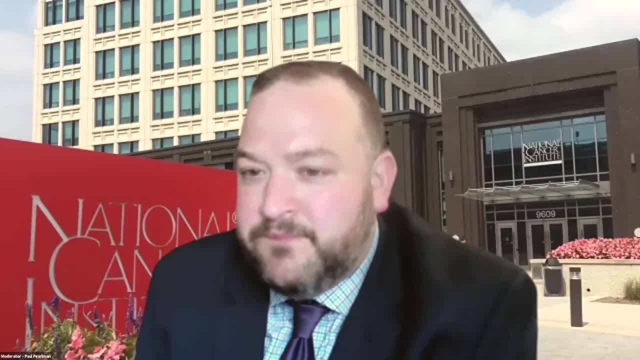 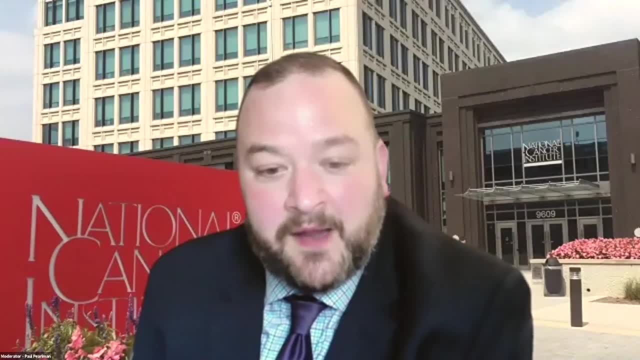 I want to invite each of the remaining speakers to maybe add a final thought, if you have one, on the session as a whole before I turn it back over to Maggie. Well, I think I'll quickly end the silence there. I think this was a wonderful session. 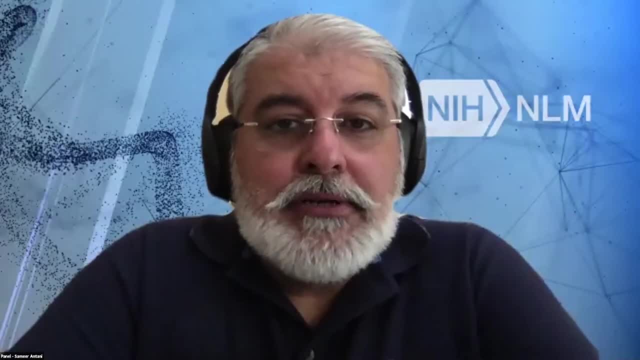 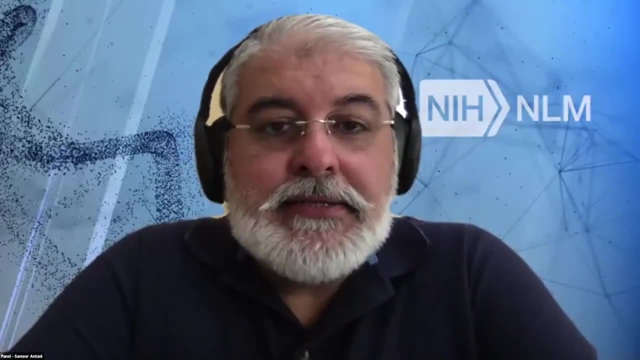 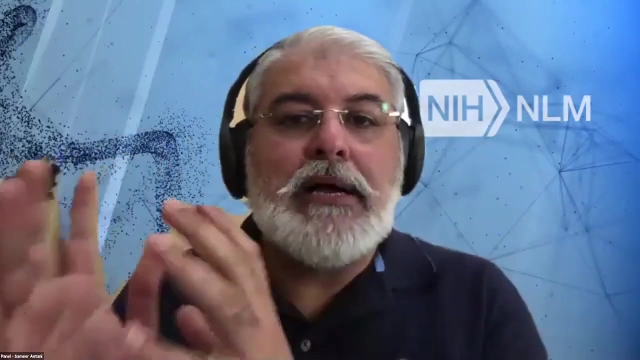 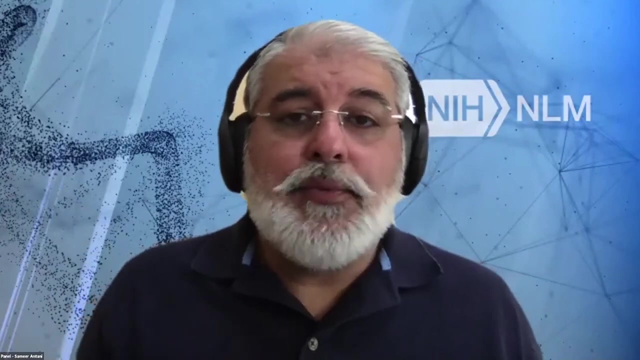 I particularly enjoyed it because it provided a broad spectrum of opportunities, challenges, close interaction between data and design and the bridge between computational sciences and biomedical sciences toward improving patient care overall. That is our ultimate goal and there are many steps toward that, which are broadly data science. 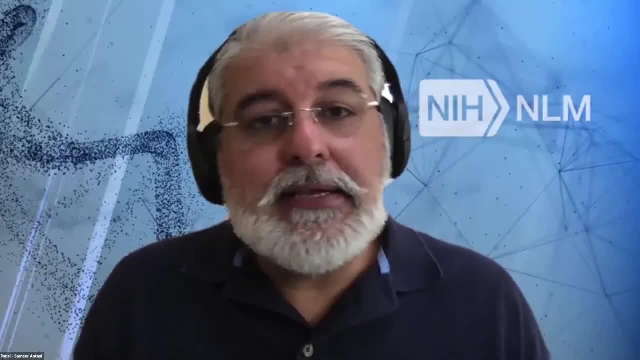 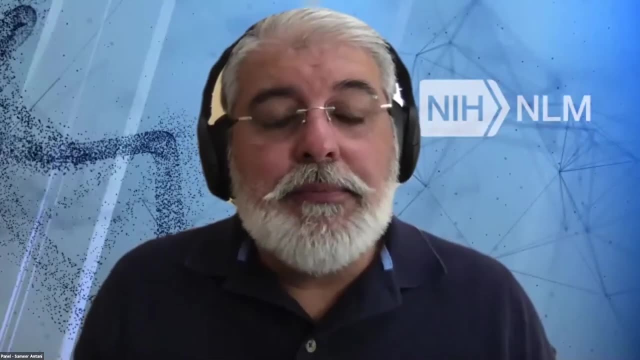 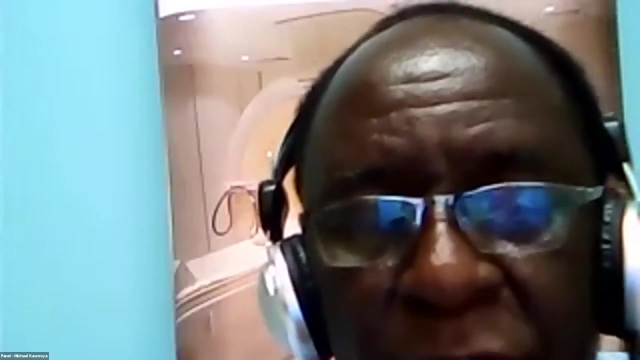 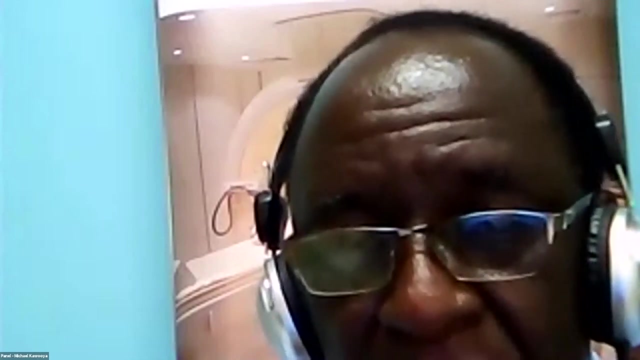 So I hope that the attendees have been inspired and the opportunities that NIH is providing would be taken advantage of. I also want to say that, yes, we have embarked on the process to bridge the gap between the high and low and middle income countries with regard to data science application. 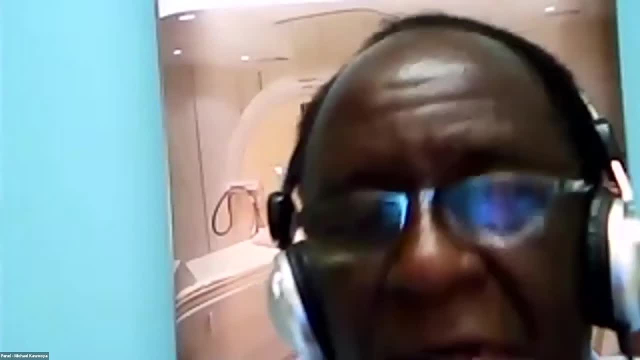 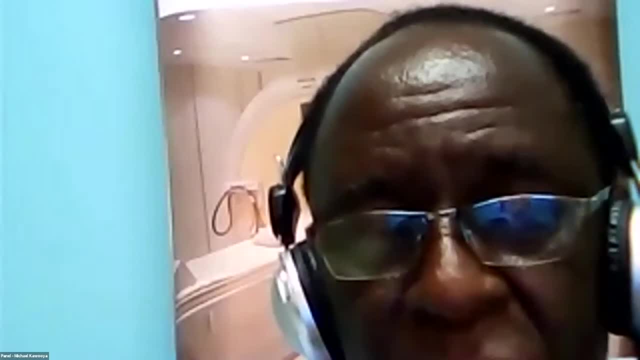 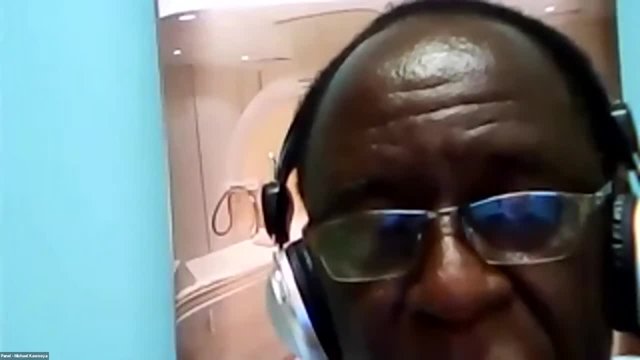 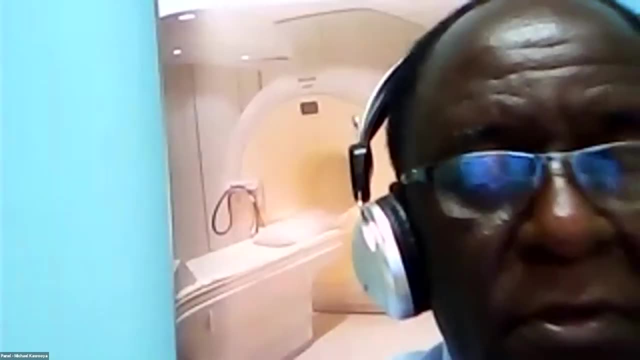 It's a very important baby step. we should have as many people on board, as much collaboration as possible, to make sure that this works. this very fast baby step really works. Some closing remarks From my side. thank you very much. The panel was pretty interesting. 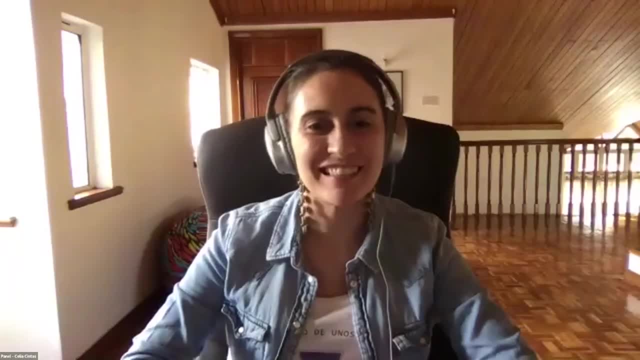 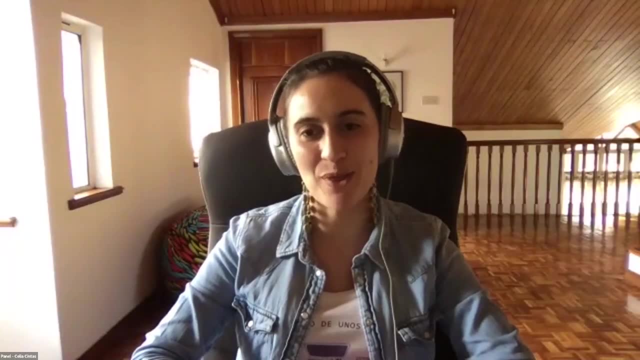 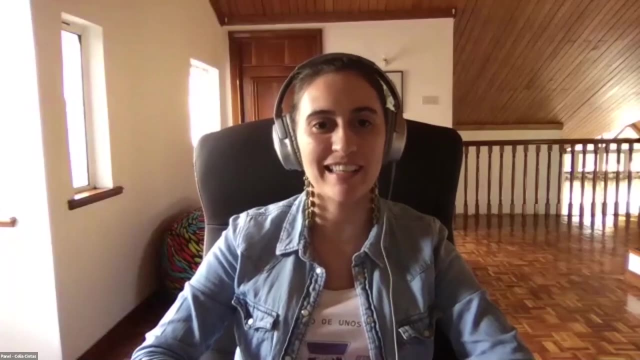 I learned a lot too. Something that I will very highlight and reinforce is all of these machine languages. Ah yeah, I really enjoyed that. learning solutions are done with domain experts side by side. as computer scientists, we cannot sit alone in a lab, get a bunch of data, match it to a deep learning model and and publish that. 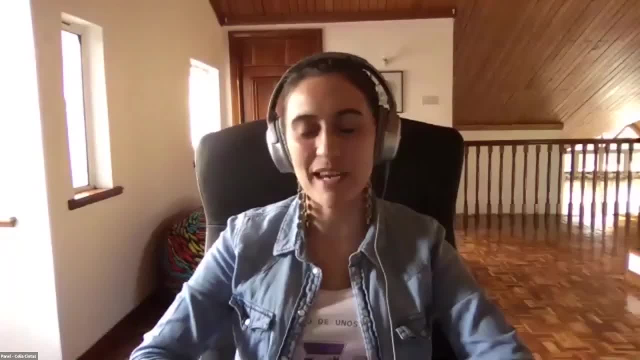 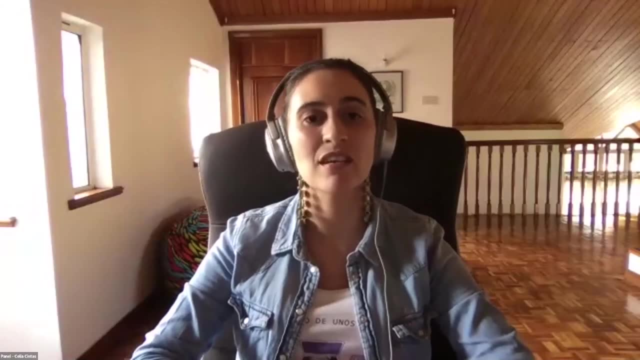 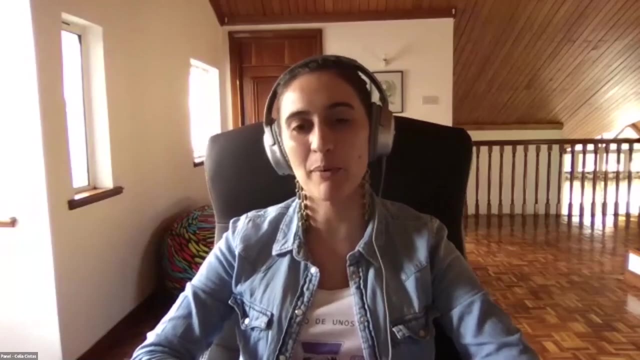 that is not sufficient. we always need a domain expert showing us new patterns on the data or new patterns even on the insides of the models. so my highest recommendation was always to work with the main experts in any problem that you're trying to solve, and especially with with the 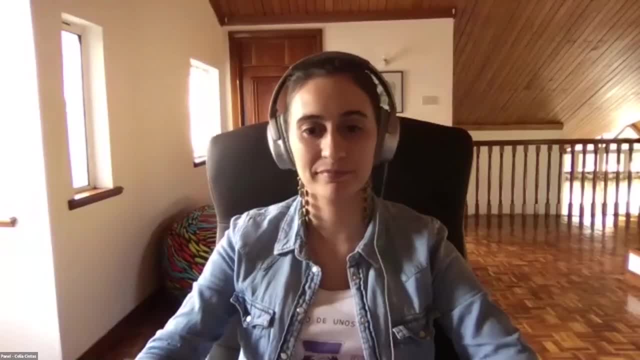 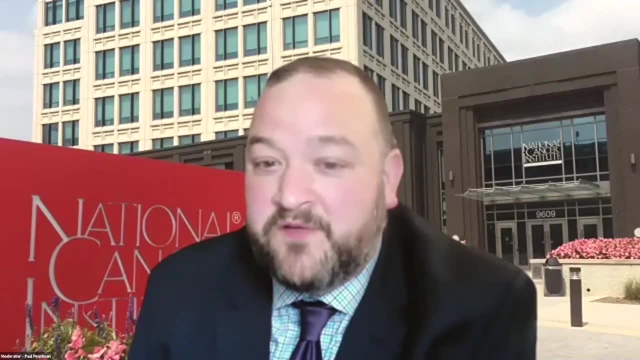 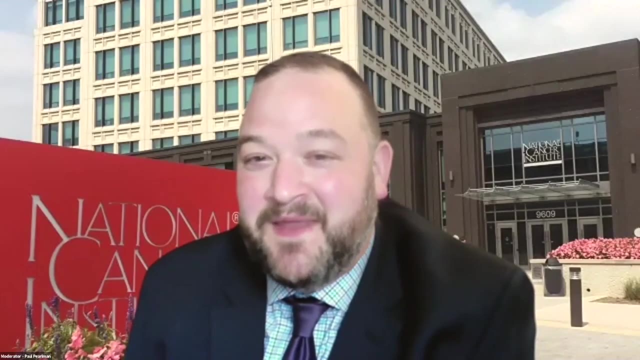 community that you're working on for sure. so i want to thank our speakers again. i um and i want to thank our attendees as well. we had well over 100 participants in this session, so i think there would be a booming round of applause happening right now if we weren't virtual um and with that. 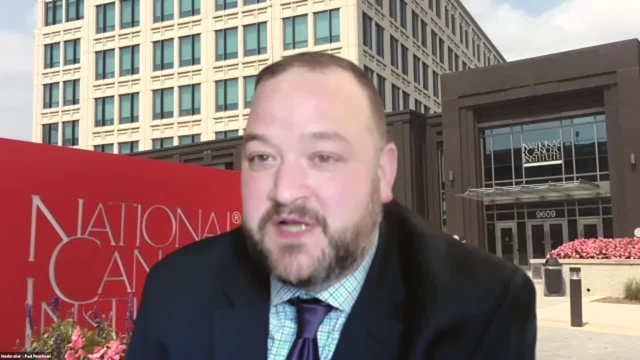 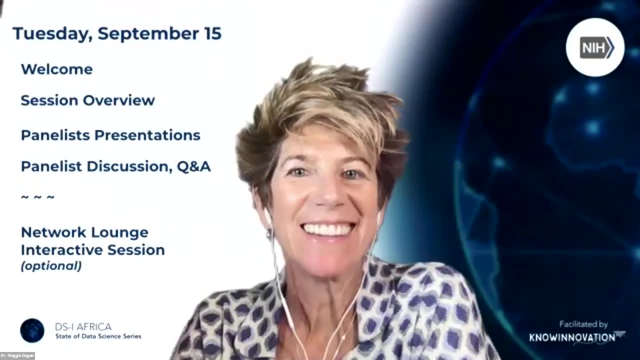 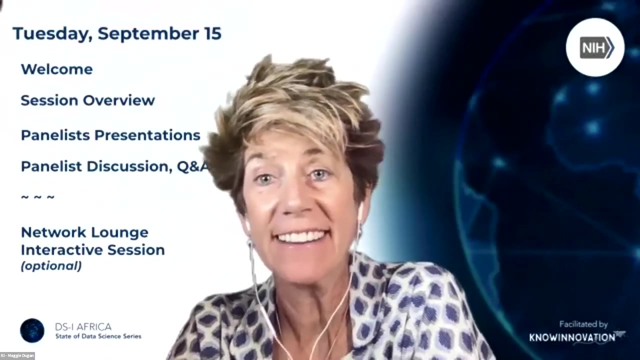 said i, i hope to see all of you in the networking lounge and i'm going to hand it off to maggie, who will explain how to get there exactly. um, yes, we have come to the end of this webinar, but we are not necessarily finished. you are invited to continue the conversation by joining the. 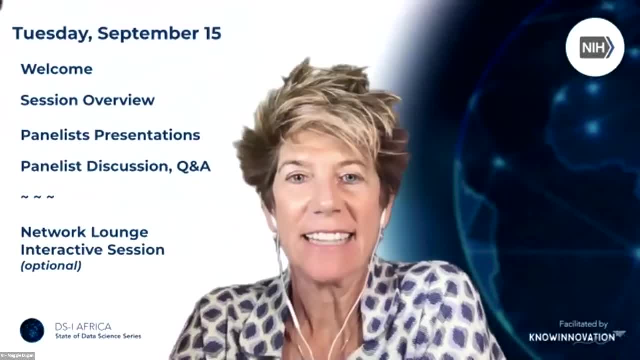 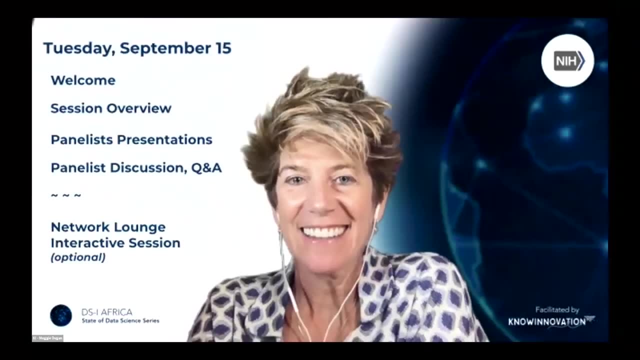 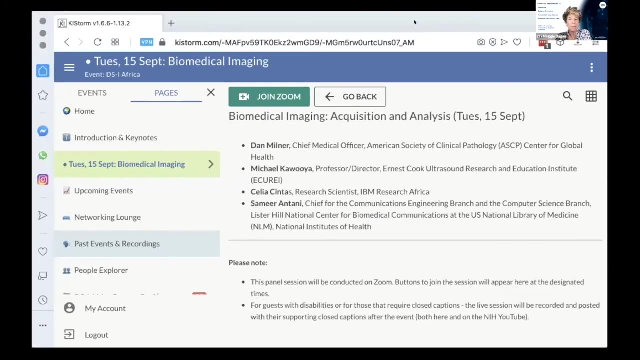 interactive networking session in the network lounge and i am going to give you a little uh demo of how to get there. maggie opens the event page on the kai storm website. so i am going to imagine that you are probably go back to kai storm. i would imagine you're on this page. this is today's page for this session. 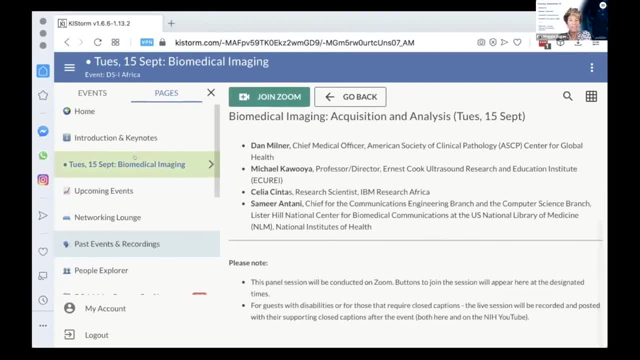 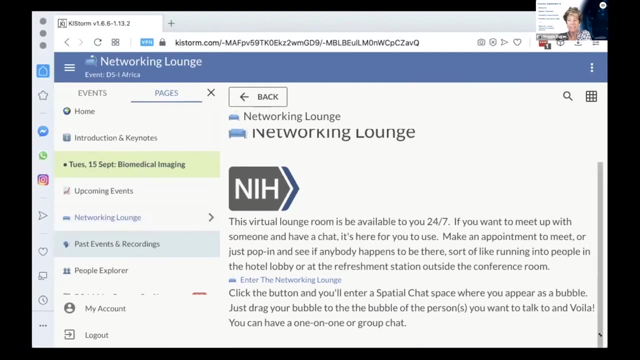 this was the zoom button that you joined to get here and if you just go down one two pages, you'll see the networking lounge on the sidebar. the networking lounge has two options below the event page. that's where we invite you to go after you leave here and when you come into here you will. 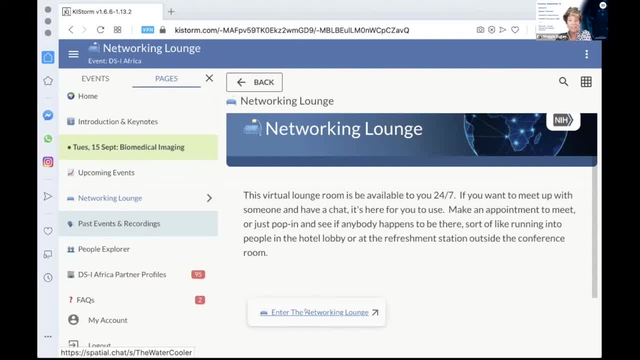 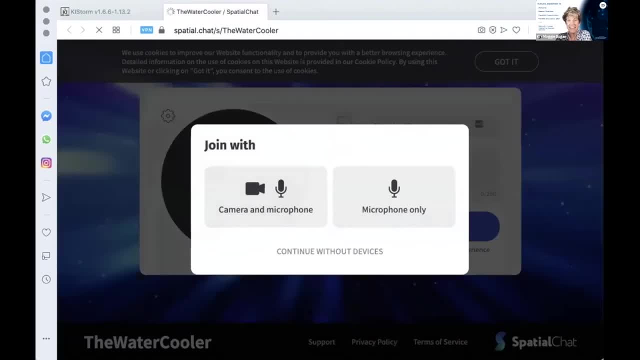 see that there is a button to enter the networking lounge. the button is at the bottom of the page. it will take you into another interface called spatial chat. you can choose for your camera and microphone. i would encourage you to do that. you can do microphone only if you want, but it's nice. 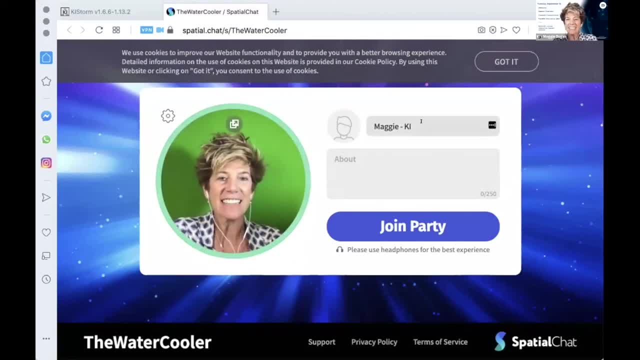 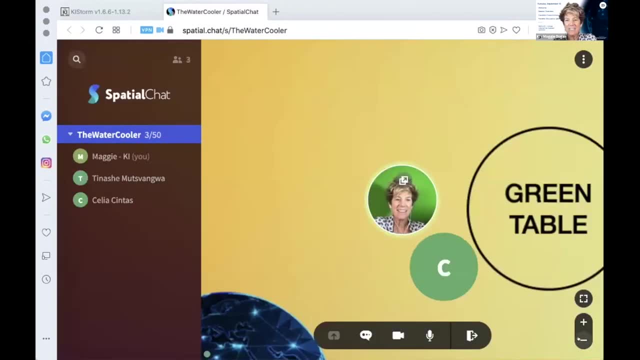 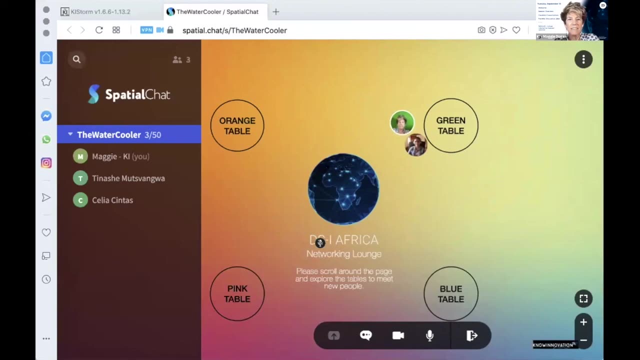 to do the camera as well. you type in your name here and then you can join the party. the screen is divided into four virtual tables and then you see that you are in the lounge. if you hit the little negative sign here, it will make the screen change for you, so you can see that there. 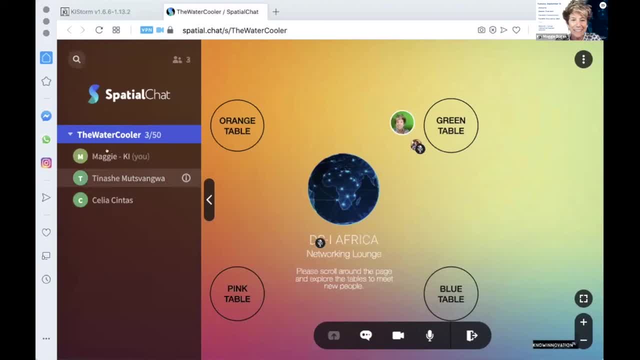 is a button on the sidebar. you can also see who else is here in the sidebar. got a couple of other people here with us already. um and uh, what we've asked our panelists to do is to place themselves at tables. so samir is going to be at the orange table, celia will be at the green table, dan will. 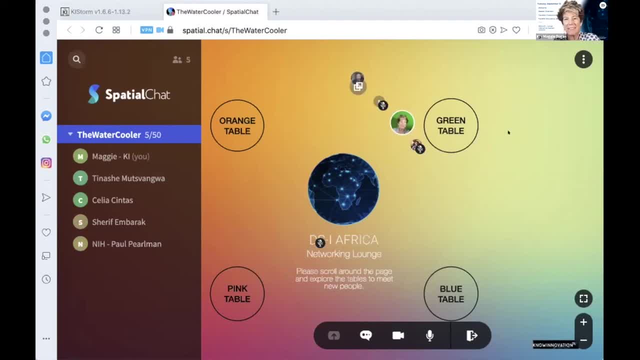 be at the pink table, hope and michael at the blue table. we'll have some other people in there you can see, and what happens is if you move your- uh, your avatar close to someone else, you can see them, and if you move away, then then you can't. so you can have conversations and you can go to different. 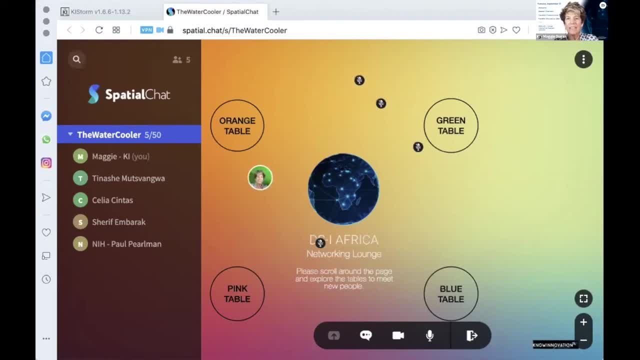 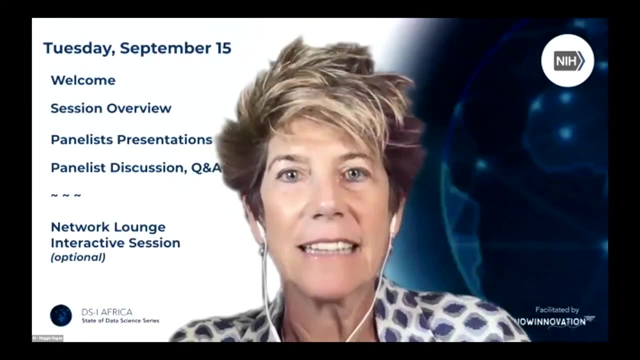 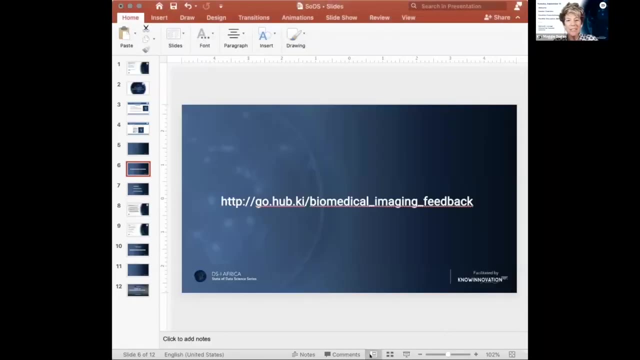 tables and check with different people. so that is how you will get to the network lounge, um. but before you go there, i just have a couple of other things i would like to share with you that are important information for you to know. um. first of all, we're really interested in your feedback. 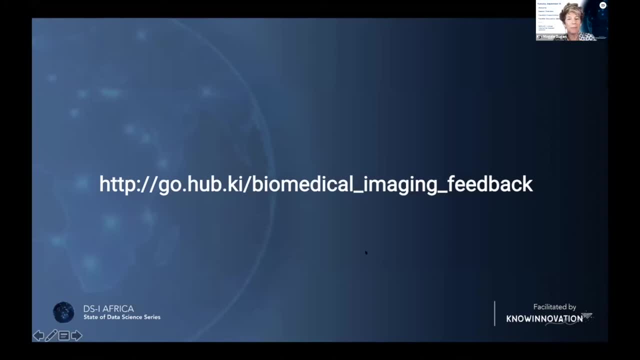 on today's session. so, uh, in the chat we'll put this link as well, so that you can easily click on it. gohubki: biomedical underscore imaging underscore feedback. but, uh, we invite you to just do this very quick survey to let us know how today's session went for you. i want to 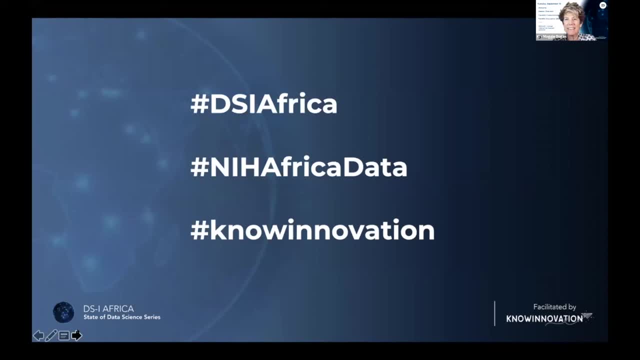 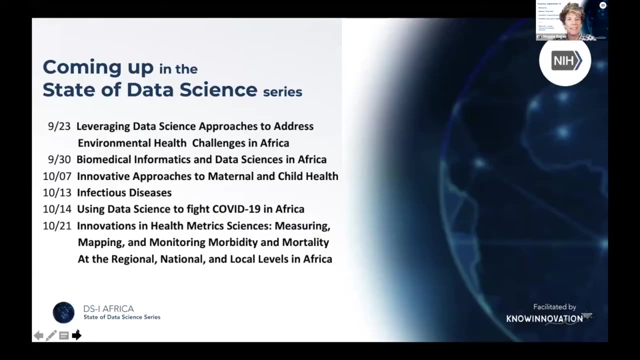 remind you about the hashtags. if you think that there was something interesting that came out of the day that you want to talk about in social media, we encourage you to use these hashtags: dsi africa, neih africa, data and no innovation. There are some more series coming up for the State of Data Science series.